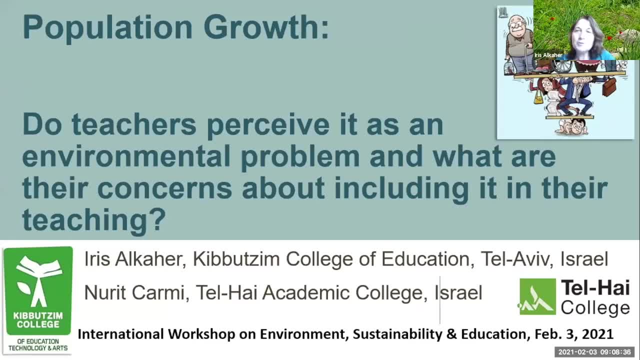 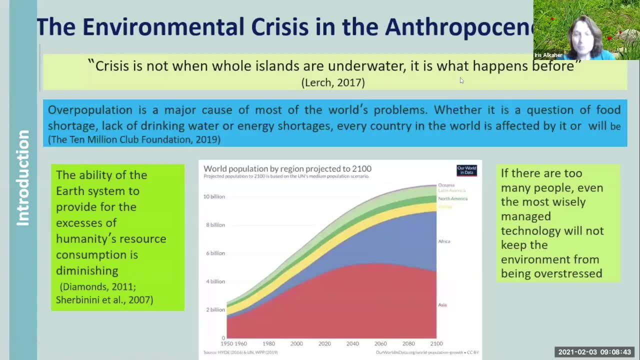 And I hope it will be interesting for you. So I want to start. So today. the current world population is 7.8 billion people as of February 2021.. And the big question is: do we have any boundaries? Can we continue in this way forever? 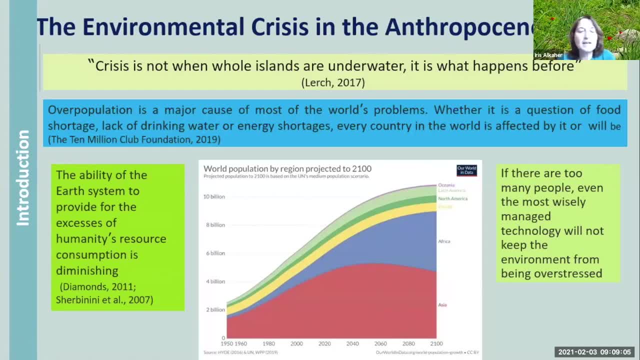 So scientists from diverse disciplines agree that human population growth dramatically contributes to environmental crisis, And it plays a major factor in the damage caused to the environment, as well as to the degradation in the quality of life and the well-being of people around the world. 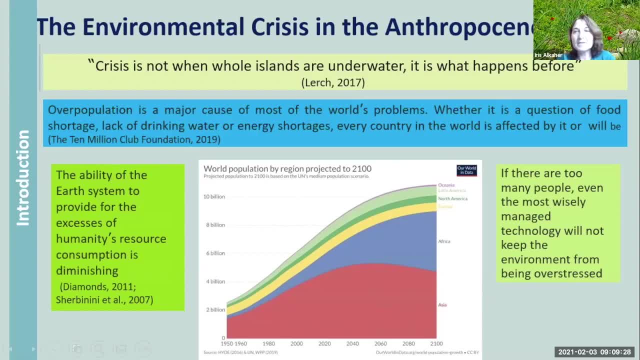 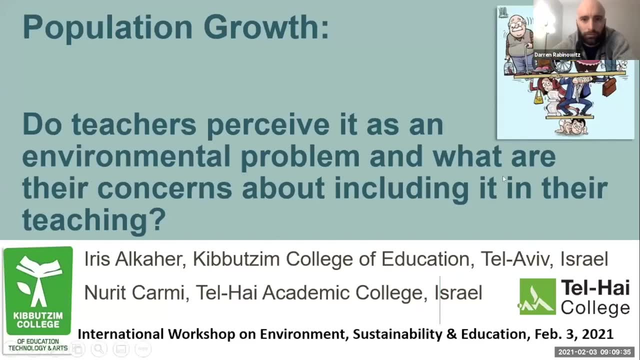 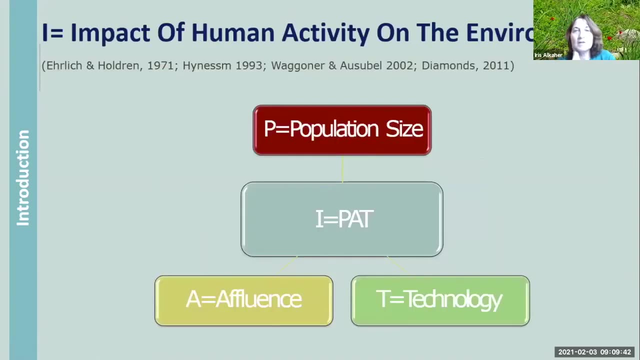 And as it says here and as it says here: oh, sorry, Sorry, If there are too many people. even the most wisely managed technology will not keep the environment from being overstressed. Most of the scientists agree that the impact of human activity on the environment is a multiplication of three major components: population size, affluence and technology. 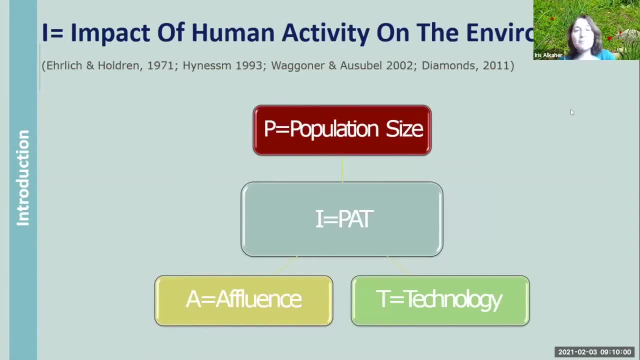 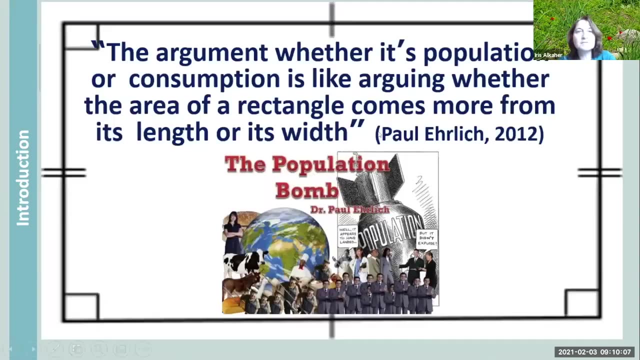 They might not agree about the proportion of population size, But they agree that it is a major factor. The big one major claim says that it's not the population growth which is the problem, It's the lifestyle of human being which is the problem. 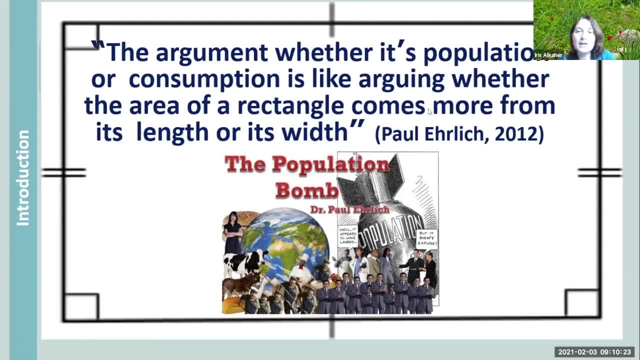 And Professor Paul Ehrlich answered this claim as follows. The argument whether it's population or consumption is like arguing whether the population growth is the problem. The answer to this claim is as follows: The argument whether it's population or consumption is like arguing whether the population growth is the problem. 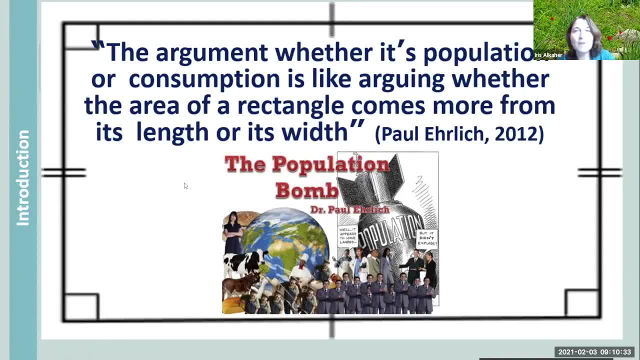 The answer to this claim is as follows. The argument whether it's population or consumption is like arguing whether the population growth is the problem. The answer to this claim is as follows. The answer to this claim is as follows. The answer to this claim is as follows. 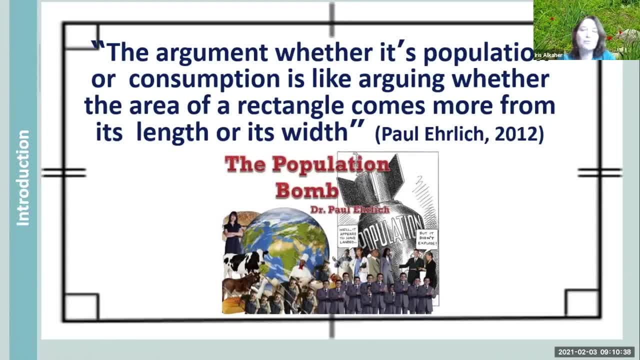 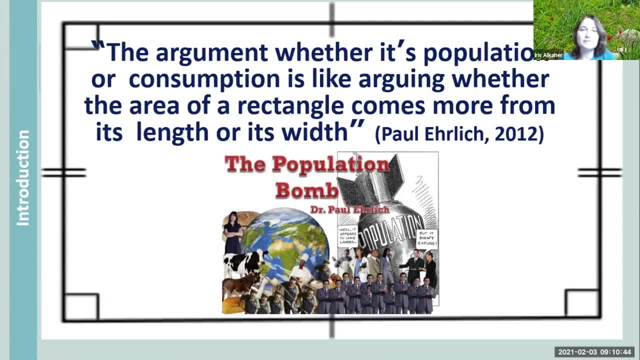 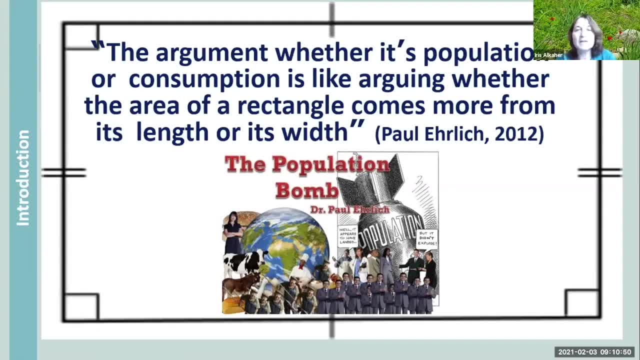 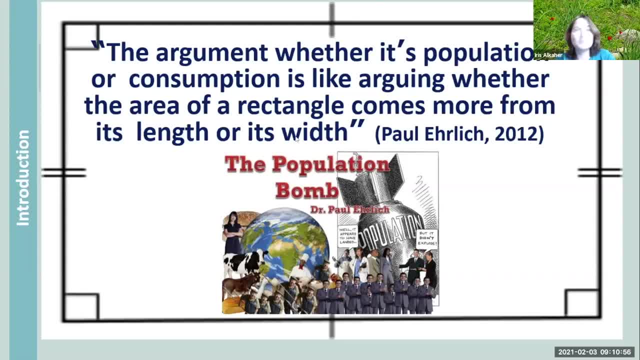 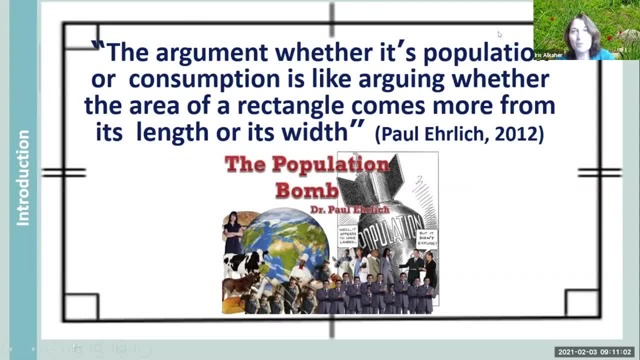 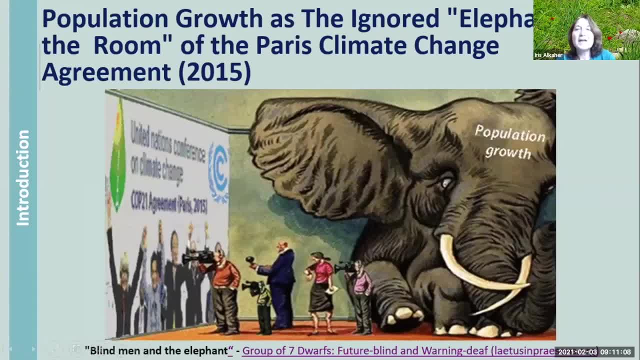 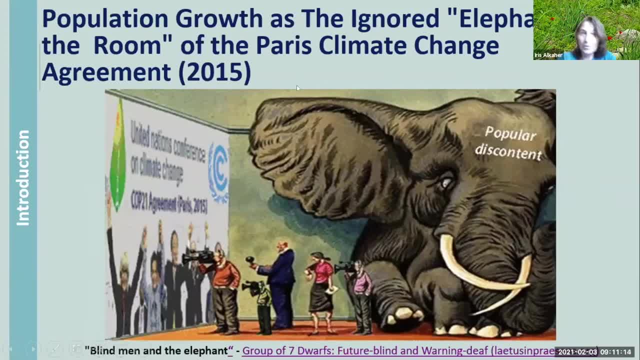 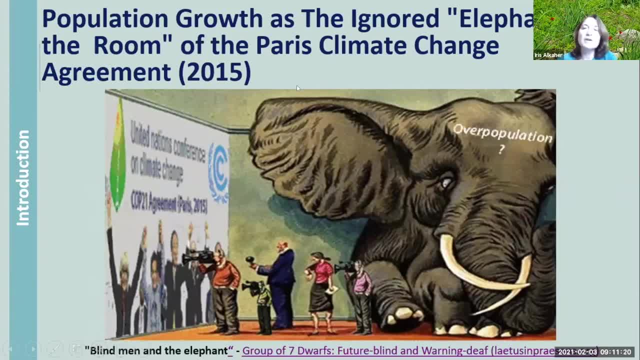 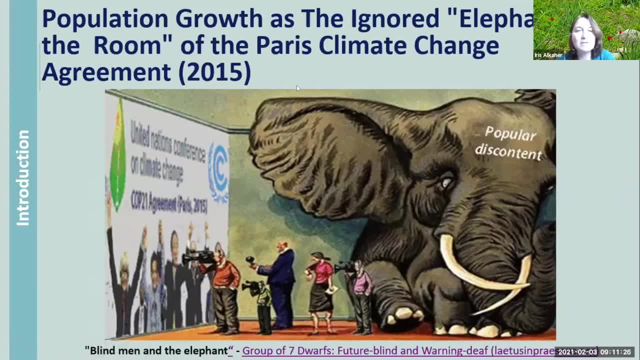 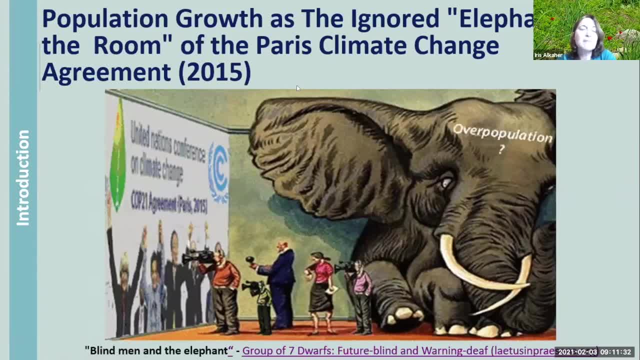 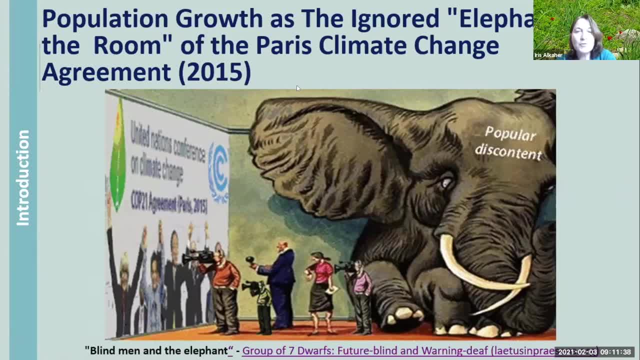 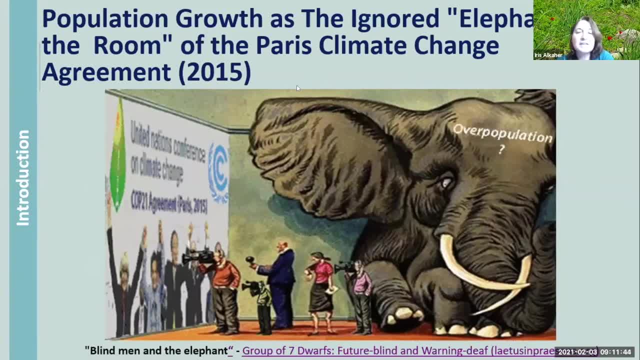 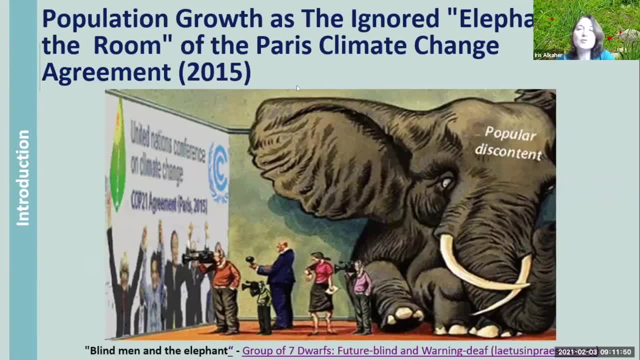 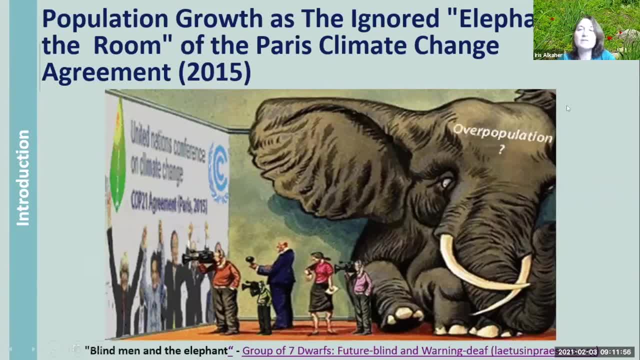 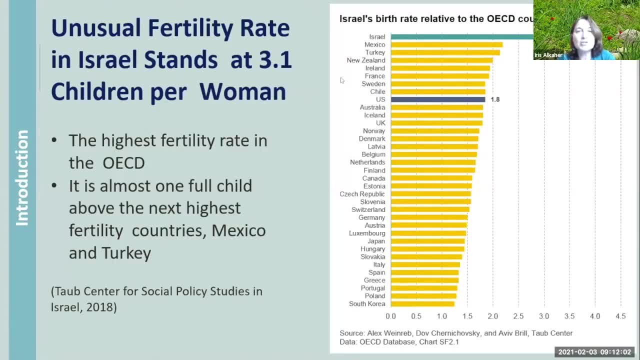 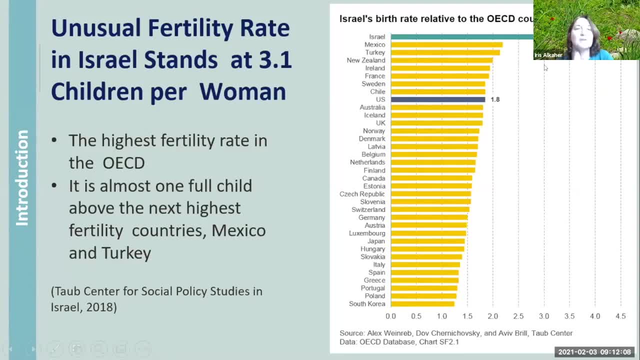 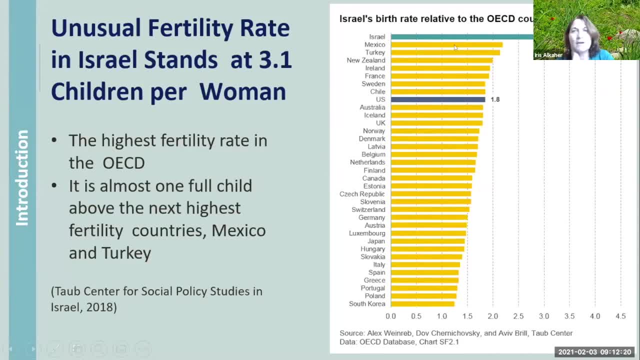 You can see the green column And this is the highest fertility rate in the OECD countries And it's almost one full child above the next highest fertility countries, which are Mexico and Turkey. You can see the US in the ninth place. 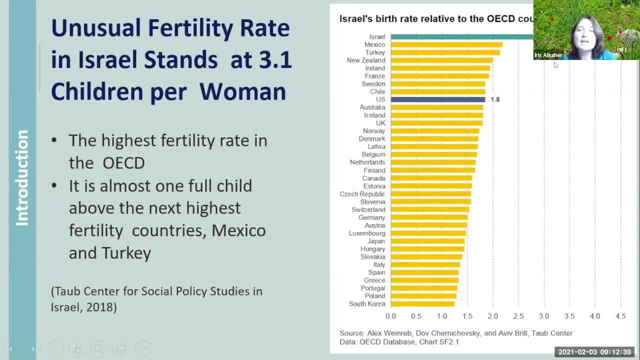 There are many reasons for that. One major reason is the pro-natalist agenda of the State of Israel, which means that the State of Israel encourages birth rate and support it. But there are other reasons that I cannot go into, but they will be presented in the findings. 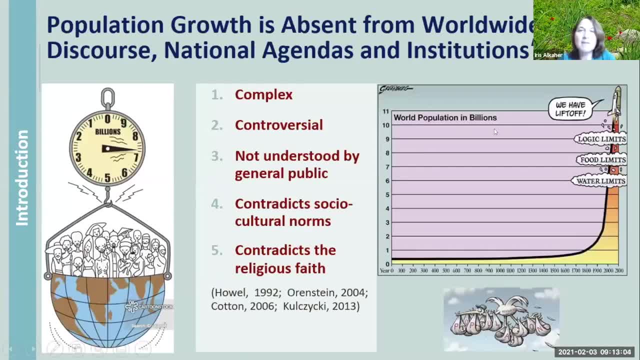 According to the literature, population growth is absent from the worldwide public discourse, From the national agendas and institutional policies of many countries, And there are several reasons found in the literature, such as that this topic is complex, controversial, is not understood by the general public, contradicts social, cultural norms and religious faith. 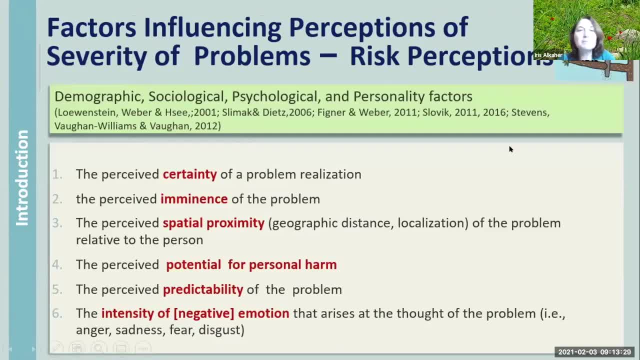 When we are looking about how people perceive a severity of problem, what are their risk perceptions. So, based on, So based on the literature, there are demographic, sociological, psychological and personality factors, And here you can see several of them. 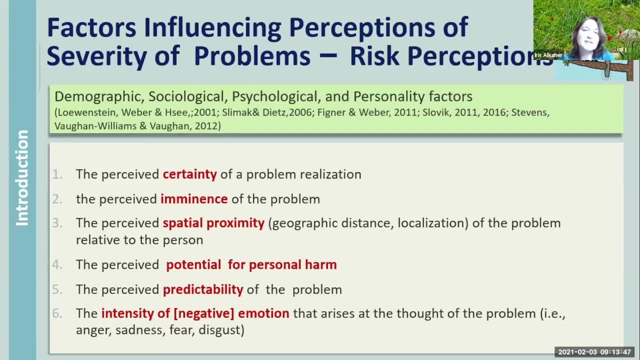 For example, how certain is the problem? What is the imminence of the problem? What is the spatial proximity of the problem? Is there any potential for a personal harm? Is the problem predictable, And what is the intent of a negative? 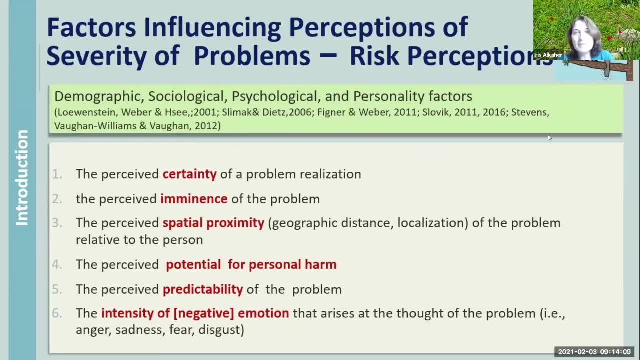 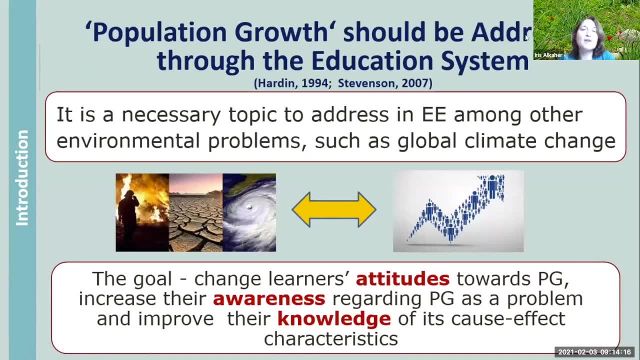 emotion. We will continue with these factors. in the findings, Scientists, science educators and environmental educators mostly agree that population growth should be addressed through the education system. They claim that it's a necessary topic to address in environmental education and that this topic is as important as other environment problems such as global. 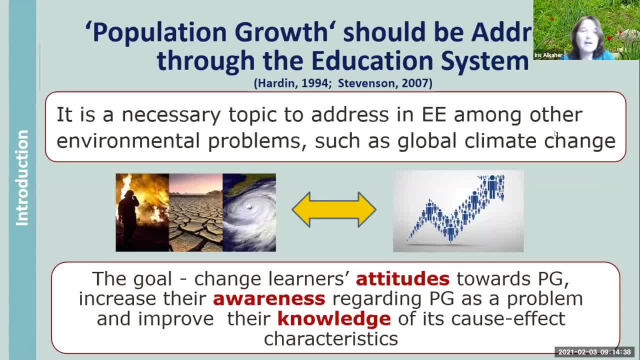 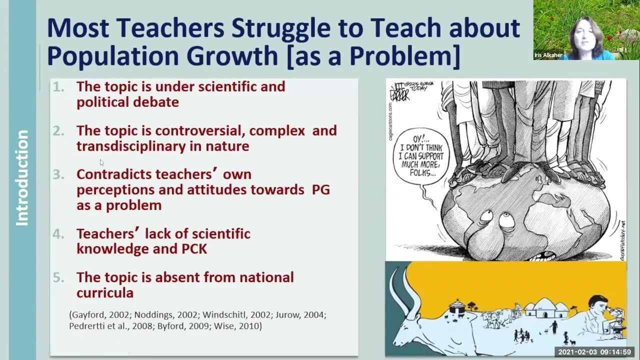 climate change. They further claim that the goal is improving or developing the learner's environmental or social environmental literacy with respect to population growth and its consequences on the earth and on people or human beings. However, we know from the literature again that most struggle to teach about population growth as a problem. 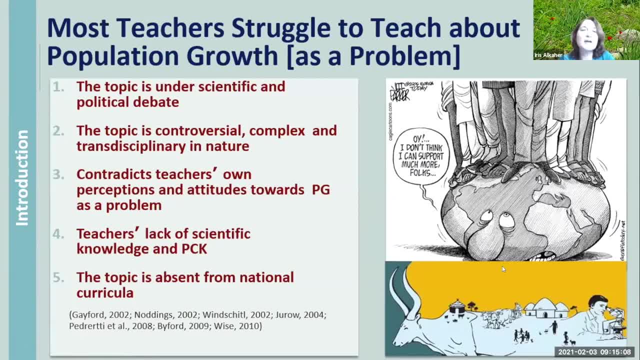 According to the literature, teachers are stressed because of several reasons. For example, they think that the topic is under scientific and political debate, that the topic is controversial, complex and transdisciplinary in nature and therefore hard to teach. It contradicts their own. 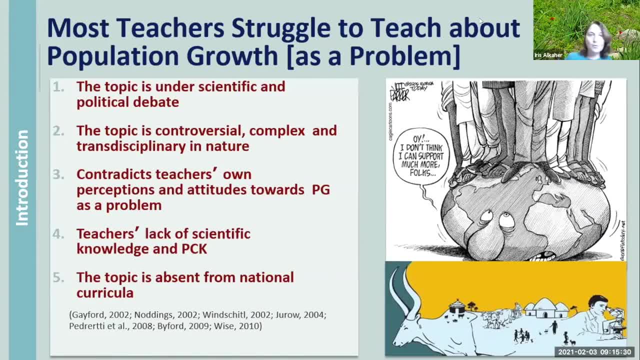 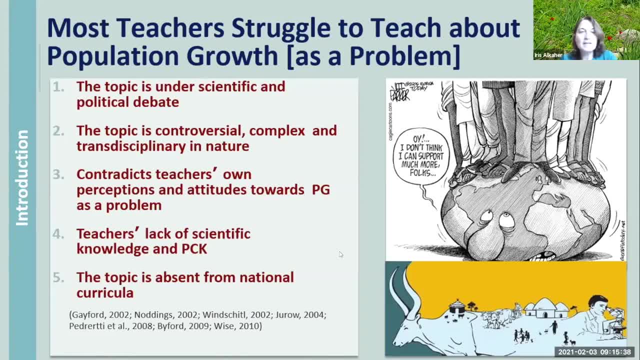 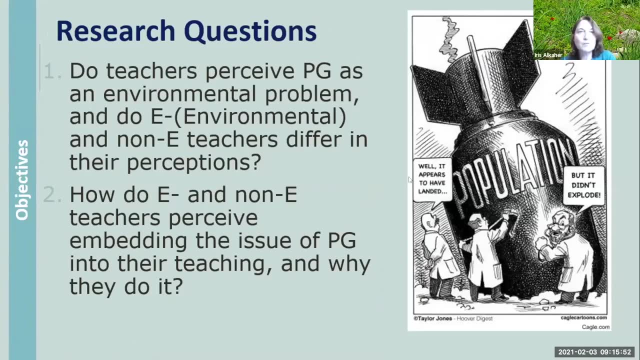 to teach. They don't know how to teach. They don't know how to teach. We just make a whatever they study And they continue to speak thisis issue and that the topic is, in most cases, absent from national curricula. So this was a short, very speedy introduction that led us. 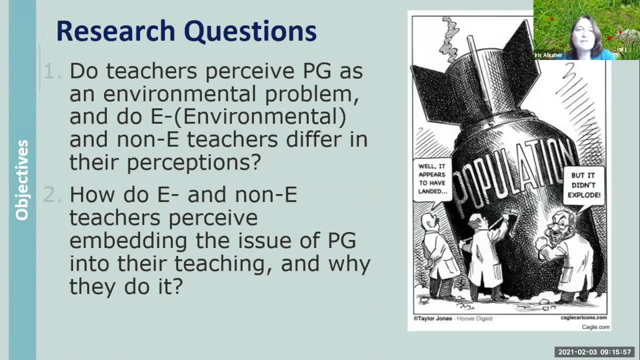 the researchers to ask two main questions: Do teachers perceive a population growth as an environmental problem or as something or that is a factor that is causing environmental problems? teachers differ in their perceptions. and the other question was a: how do a environmental and non environmental teachers perceive embedding the issue of 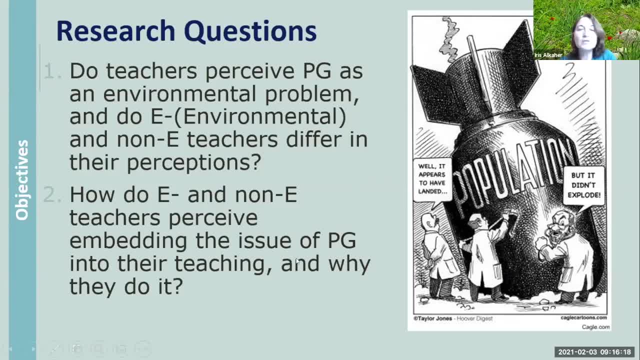 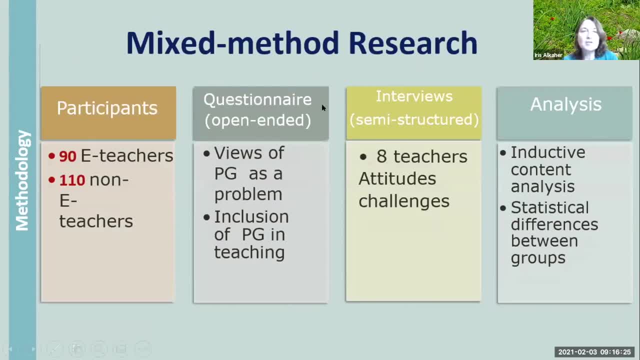 population growth into their teaching, why they do it or not, or or, or why do they don't do it. we use the mixed method research and we had a two hundred participants. about one hundred participants were environmental teacher and the other were non environmental teachers. environmental teachers where? 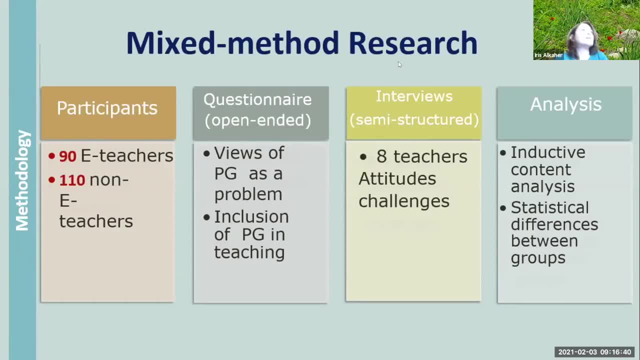 the teachers that way in that area reported in the questionnaire that they had environmental courses or that they were exposed explicitly to environmental topic during their academic studies, and while the non- the non environment teachers reported that they did not, that they were not exposed to environmental courses or topics, we used a question. 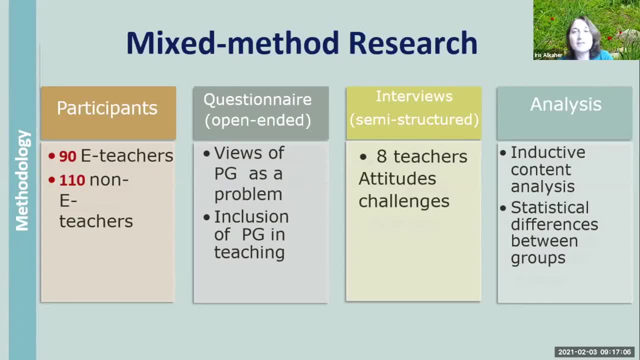 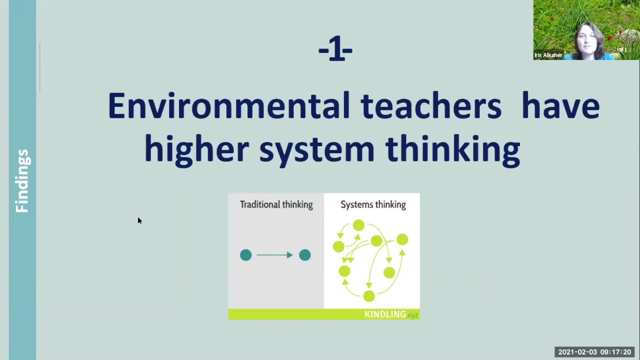 questionnaire with closed and open ended and in interviews, and today I will present a present several results from the questionnaire. so let's move to the finding a little bit. so first finding is that environmental teachers have higher system thinking. if you look at this and at this table you can see the 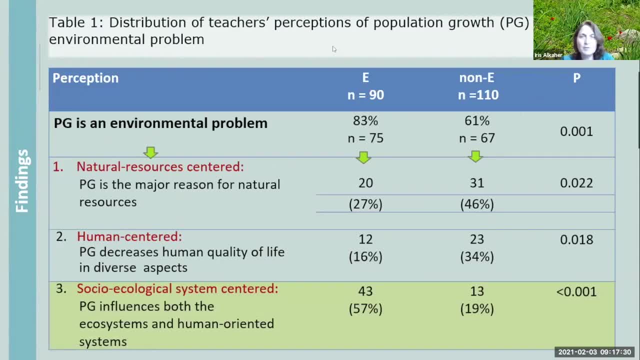 distribution of teachers perception of population growth. in the environmental program and among the environmental teachers population growth is perceived as an environmental problem problem, highly, definitely, highly and significantly highly. then, among the non environmentalist environmental teachers, most specifically in the environmental teachers had a more developed system thinking they and 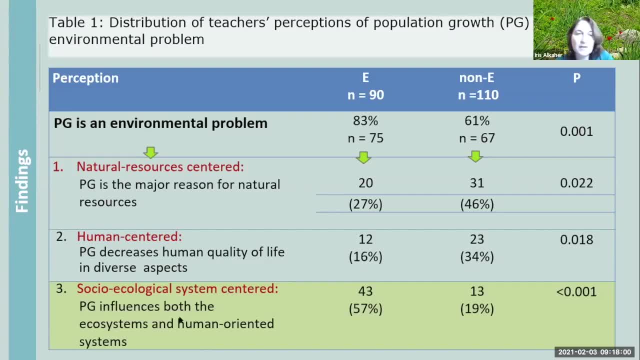 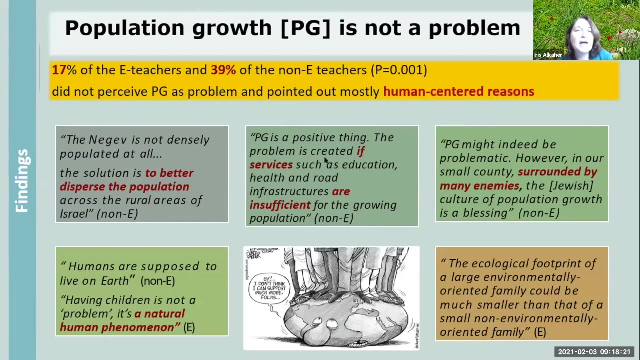 almost sixty percent of them understood that a population growth influences both ecosystems and human-oriented system, while only twenty percent of the non of the non environmental teachers perceived and PG in this way. I'll continue with some examples. so what's going on with the, with the 17 and percent? 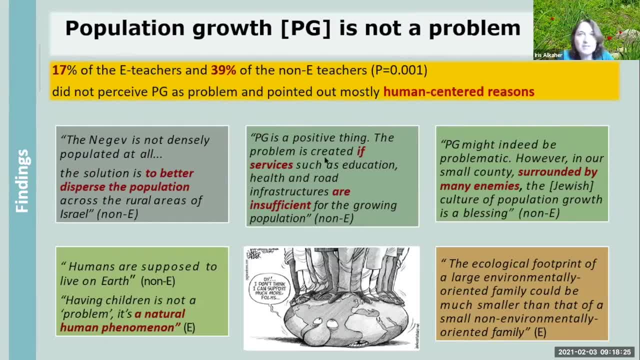 of the teachers and in forty percent of the non eat teachers that did not perceive a PG is as a problem. so we found out out that they pointed out mostly human centered reason, for example. I will read two examples: a PG might indeed be problematic, however, in our small country. 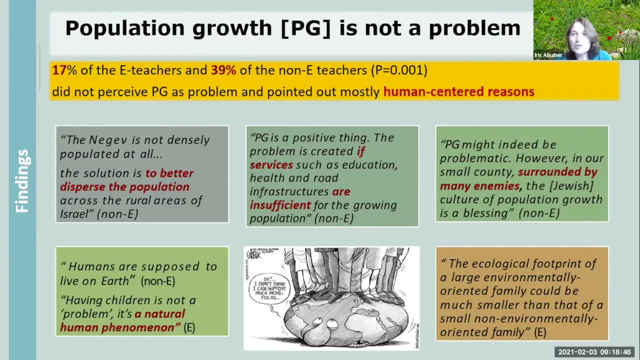 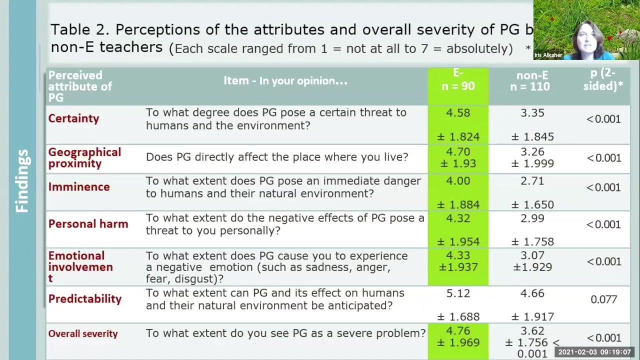 surrounded by many enemies. the Jewish culture of population growth is a blessing. a PG is a positive thing. the problem is: is created if services such as education, health and road infrastructure are insufficient for the growing population. so very human centered reasons in most cases. here you can see in this table the same. 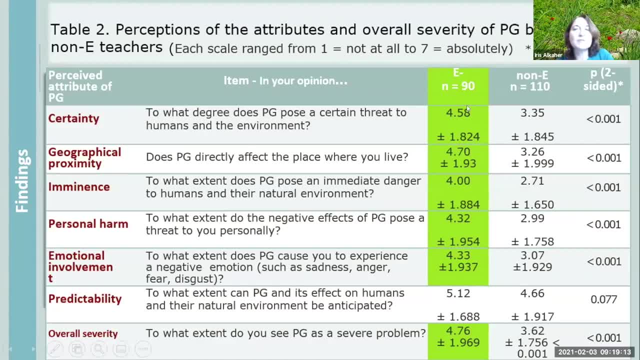 several attribute that I presented earlier and and here you can see that that the severity, the severity of population growth is a problem, was a perceived more highly by the environmental teachers and this significant in the in this was a significant different and this was except for a, for the predictability a factor and if you, if, if we will look at. 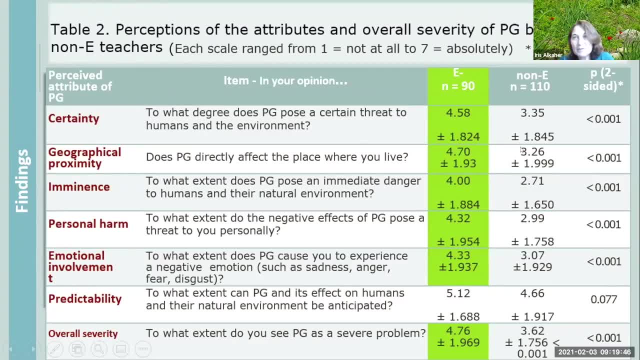 the and at the values of the non environmental teachers. we could, we could see that the, the teacher, somehow a, responded neutrally in a in, but the environment teachers did not, did not in responding neutrally. so there is the another difference between the two groups in their perception of population. 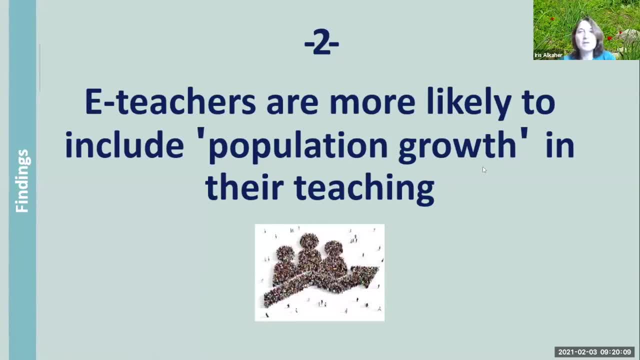 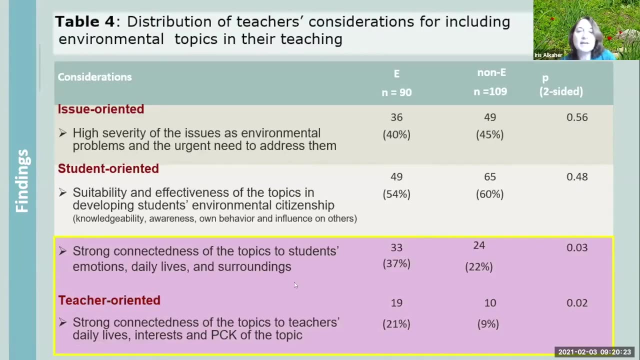 growth as a as a problem. and then the next finding is that e-teachers are more likely to include a population growth in their teaching. maybe it's not surprising, and in this table we can see a first. first of all, what are teachers consideration to include environmental topics in their teaching? we can see that. 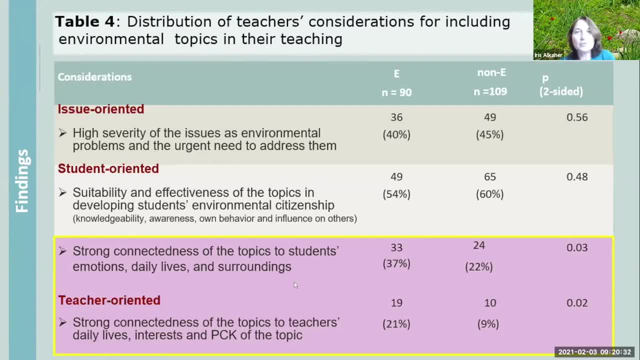 they are more likely to include environmental topics in their teaching and not only population growth. and we found that there are four, four, excuse me, three- considerations: issue oriented, so student oriented, and teacher oriented. and regarding the issue oriented and student oriented, we found that that in between a forty percent and sixty percent of teachers from both 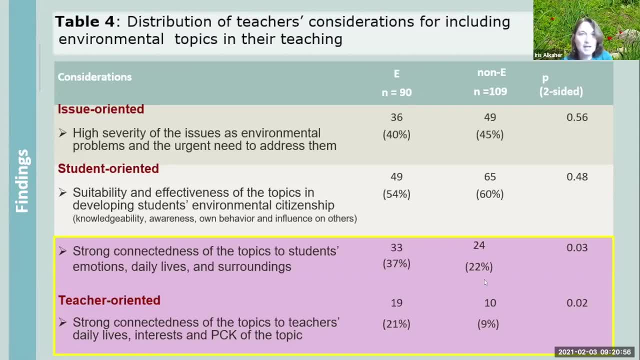 groups: a include environmental topics according to their harassment severity in in in high severity, as environmental problems and their suitability and effectiveness in developing students environmental citizenship. however, we did find some differences between the between the group with connected to to a to other other considerations, a strong connectedness of the topics and to students emotion and daily life. and. 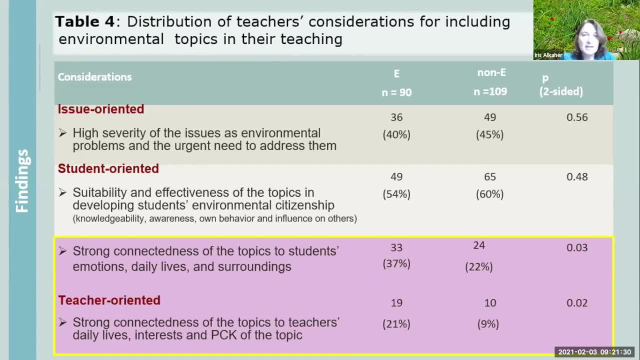 teachers also said that that they include environmental topic, according to their own, a strong connectedness of the of topics a into their daily, daily life interest and in their capacity of teaching, of teaching and the subject. so this was more general about environment, environmental topics and the consideration to include it more. 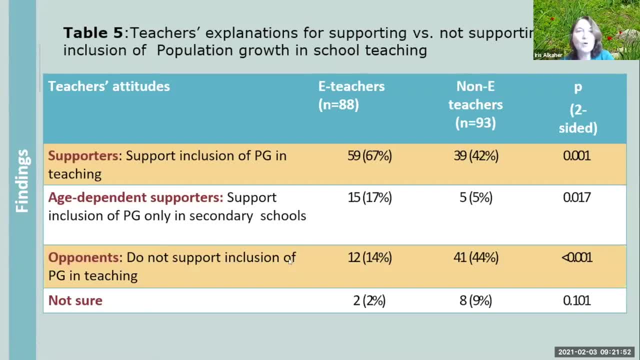 specifically about a population growth. as you can see here, we found a. we found a after a after an analysis, the analysis of teachers, explanation a for supporting or not supporting the inclusion of population growth and school teaching, that a teacher, a have three main attitudes: supporters, age dependent supporters and opponents. and 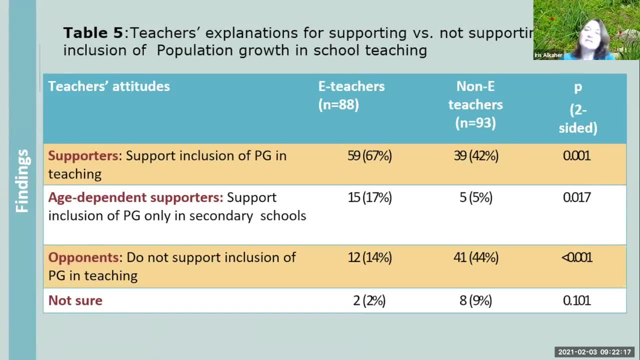 we found and a significant differences between the two groups: almost a almost, and let's say a two-third of the of the environmental teachers support inclusion, inclusion of population growth in teaching, and only only fourteen percent, a oppose this and vice versa, and another and another, a different picture is. 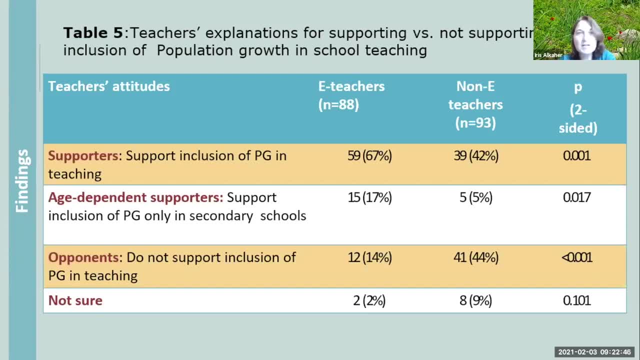 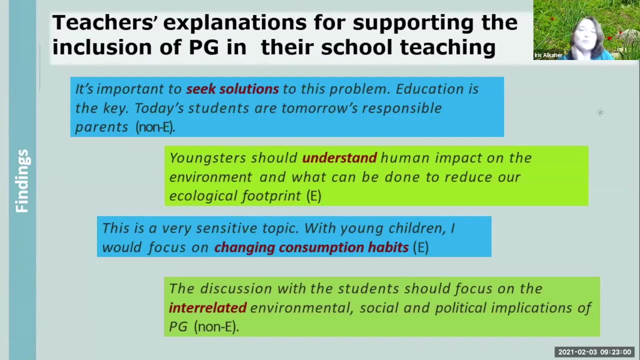 represented by the non, non environmental teachers and which we found a forty, about forty percent of supporter and opponents. so, excuse me, and when we looked at the teacher explanation for supporting the inclusion of a population growth in their school teaching and we found a, we found a interesting, interesting. 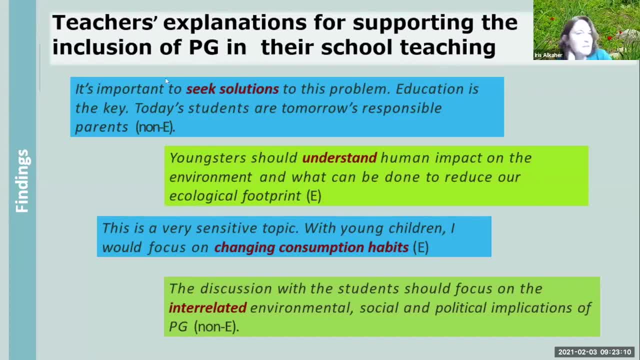 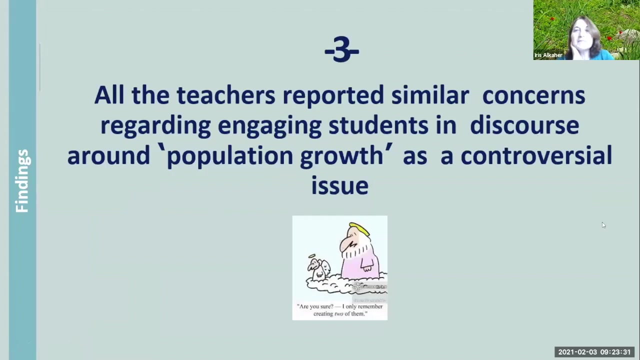 explanation in both groups. for example, it's important to seek solution to this problem. education is the key today. students are tomorrow's responsible parents and in another example, this is a very sensitive topic with young children. I would focus on changing consumption habits. I will not read the other and and I will move ahead to the third. to the third. 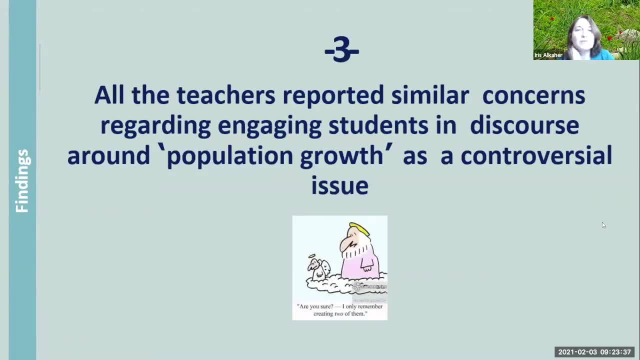 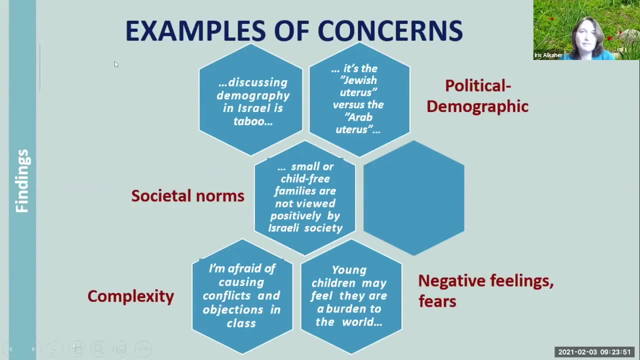 piece of finding. so we found that all the teachers a reported similar concern regarding engaging students in this course around. population growth is a controversial issue, so we did not. we did not find and concern that were inclusive for environmental teachers or in other examples or in other concern that was. 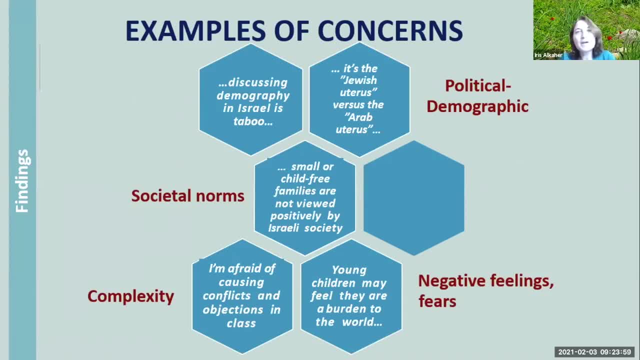 exclusive for the other group. so in the examples of student, of a teacher's concern, you can see here that they represent several themes: political, demographics, social, social norms, complexity of the topic and negative feelings or fears. and I can read the example. they are short: discussing demography in 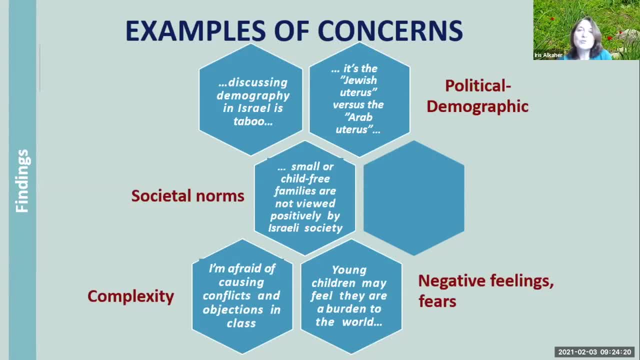 Israel is taboo. if the Jewish uterus versus the Arab uterus, small or child three families are not viewed positively by the Israeli society, I'm afraid of causing conflict and objection in class. young children may feel they are a burden to the world. I think I'll go to. 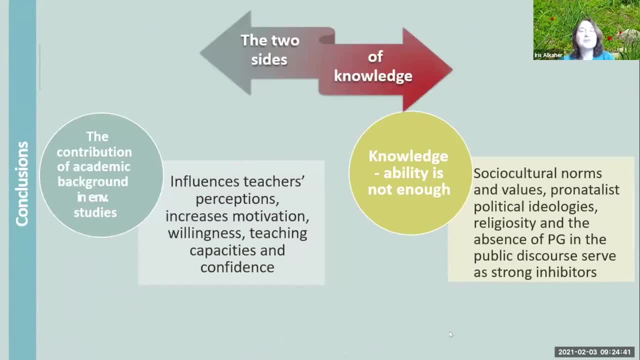 the conclusion. unfortunately because of the time, we have, of course, many, many conclusion, but one conclusion relates to the, to the role of of knowledge, and we found that there are two sides for knowledge. on the one side, in the environmental background of the teachers in in their academic studies, did influence their perception, widens, widen their perception. 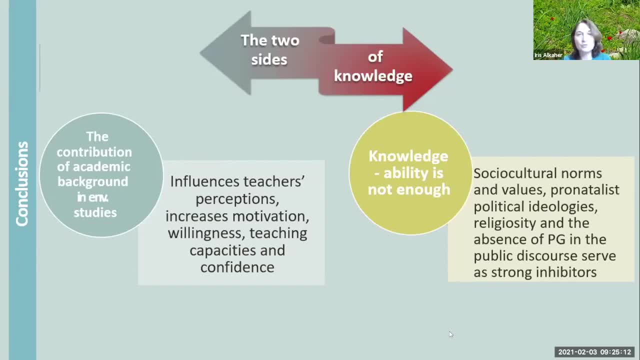 about the population growth and its connection to the environmental crisis. it also increases a motive, their motivation, willingness, teaching capacities and their confidence to include this topic into their teaching. however, no, gel ability is not enough. we found in both group other factors that inhibit, inhibit including this topic in their teaching, such as socio-cultural norms and values. 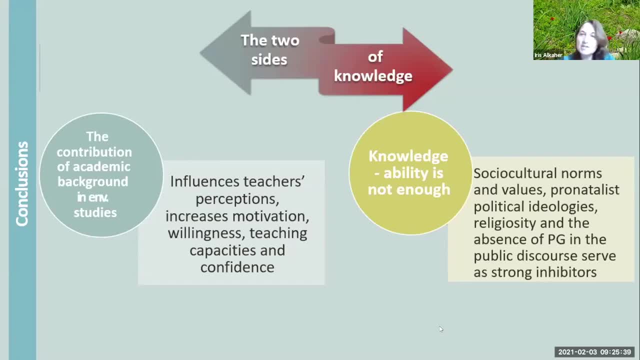 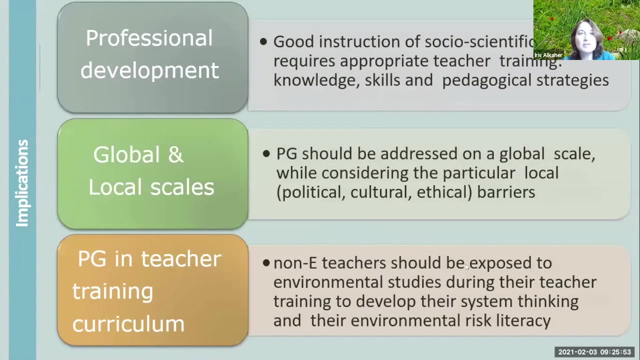 a pro-natalist political ideologies, a religiously, and the absence of the topic in the public discourse and some other factors. so if I would, if I would move on to the implication. so I summarized here here three: a good instruction of social scientific issues and in population growth is considered as one is a social scientific issue. it. 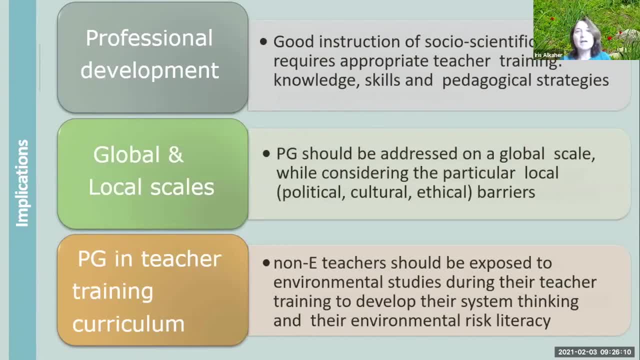 requires appropriate teacher training with respect to knowledge skills and pedagogy pedagogical strategies. population growth: we claim, or we suggest, that population growth should be addressed on a global scale, but also on a global scale, but also it's important to consider the particular, local, a political, cultural. 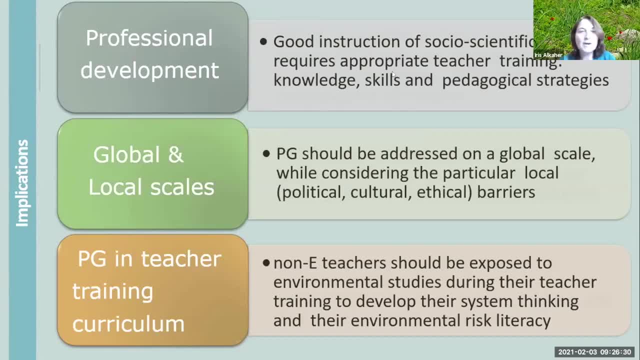 and ethical barriers, and we also we also recommend that non-environmental teacher should also be exposed to environmental studies during their teacher training in order to develop their system thinking and their environmental risk literacy. and and we claim that this topic should should not be studied or addressed only on the global scale. and we also recommend: 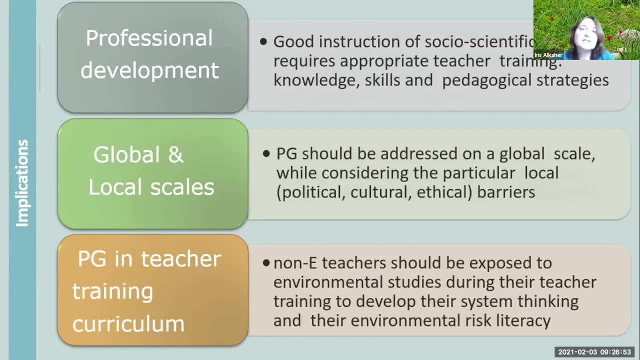 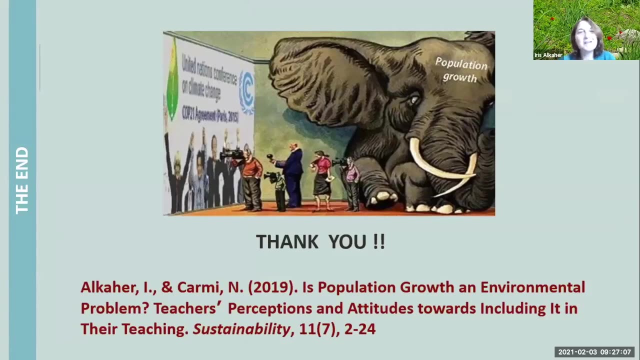 that non-environmental teachers should also be exposed to environmental studies during their education. only only with a science the assigned student or teachers, or biology, or or um geography. it fits everyone. and that's it, very short and very partial for now. should I stop sharing? yes, yes, thank you, Iris. thank you very much. 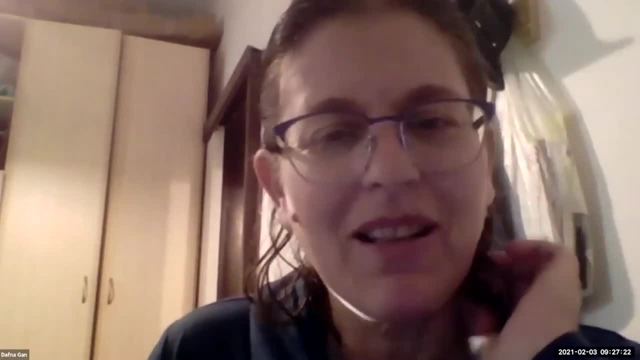 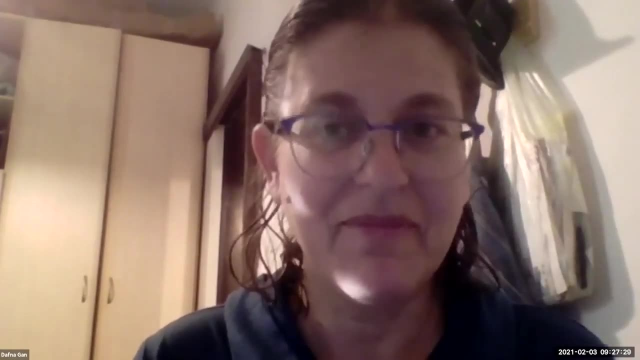 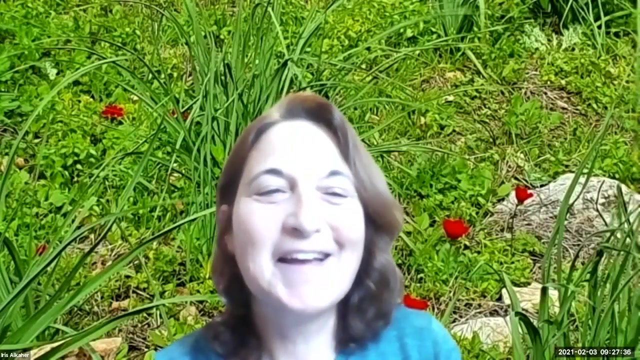 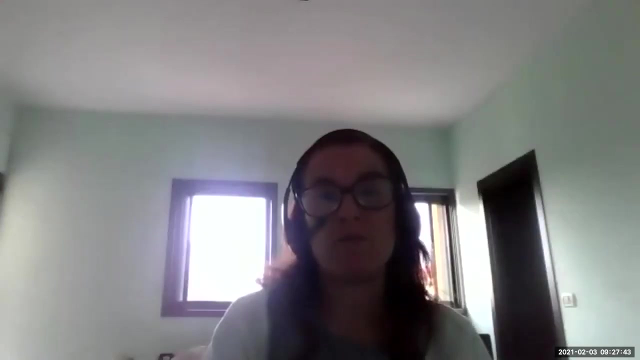 and now we are open to another question from τον questions. this topic is very emotional. it's very, very emotional. so if you have some rejection and resistance, come, come and okay and speak. i have a question. i have a question. which grade grade these children? i didn't understand. 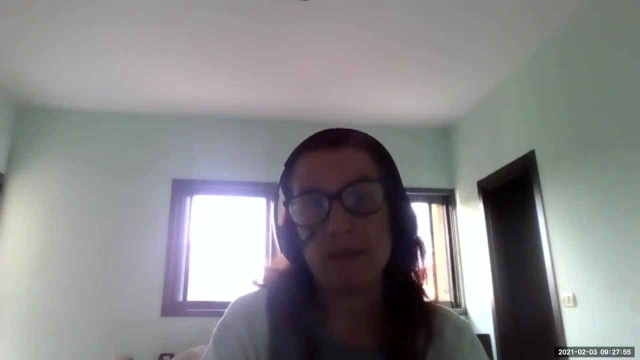 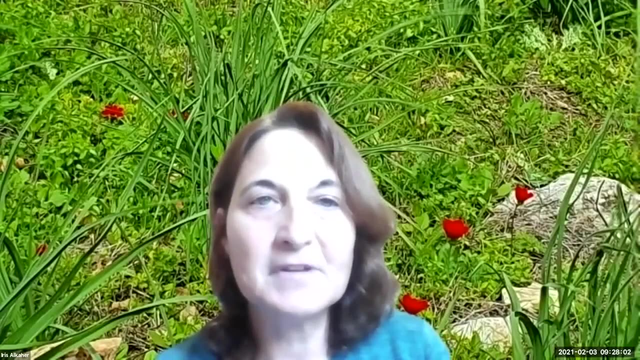 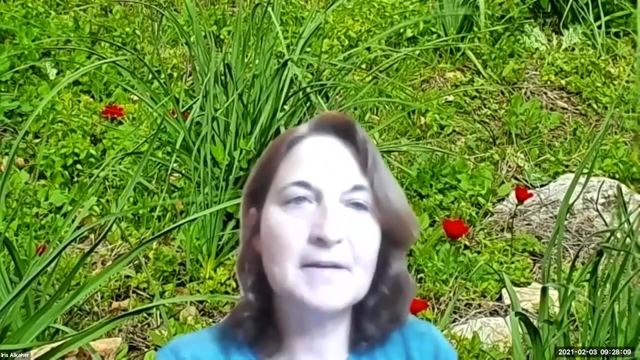 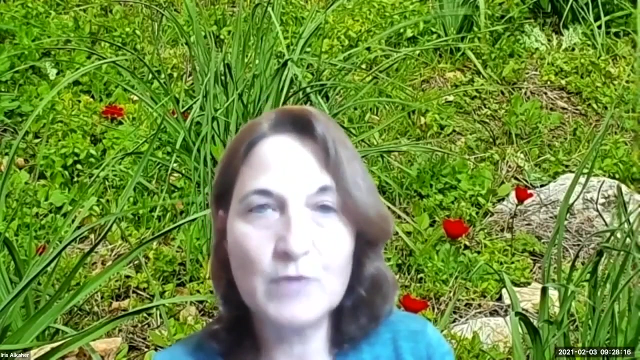 it's a high school or elementary school. i didn't understand the teachers that were included in the in the um in the study were: um were preschool teachers, elementary school teachers and um and also um secondary school teachers. we didn't, we didn't separate them into um, into um, into different groups because of the um of the sample. 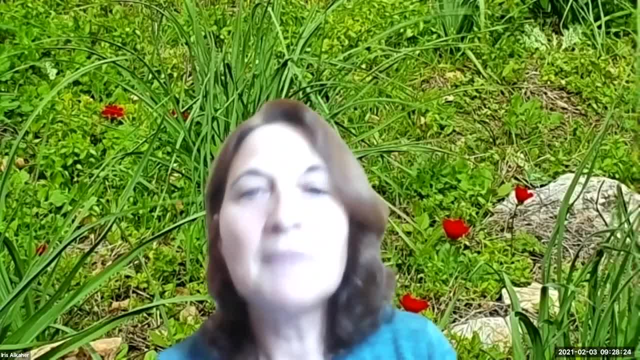 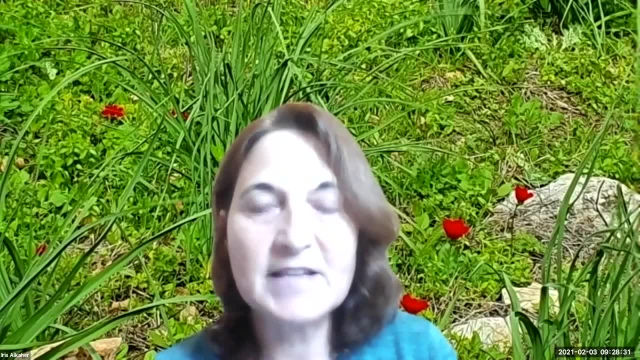 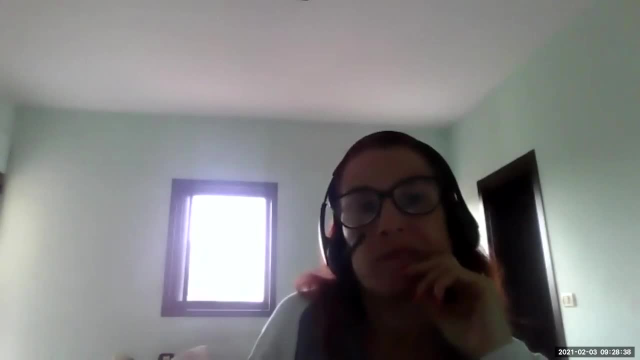 that was not very high and but it's a good. it's a good question because in their explanation, some of the teachers did, uh did, address the age of the of the students or the kids, in relation to population growth. uh, thank you. uh, michael, do you have another question? no, no, 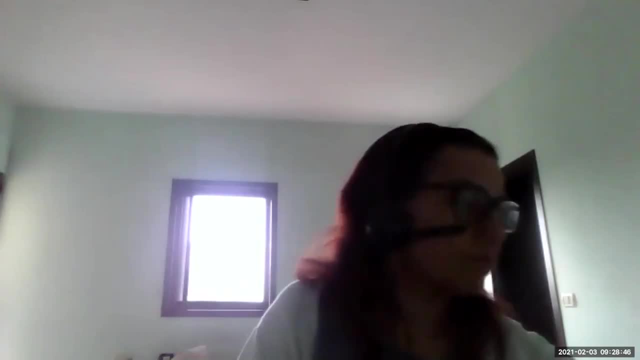 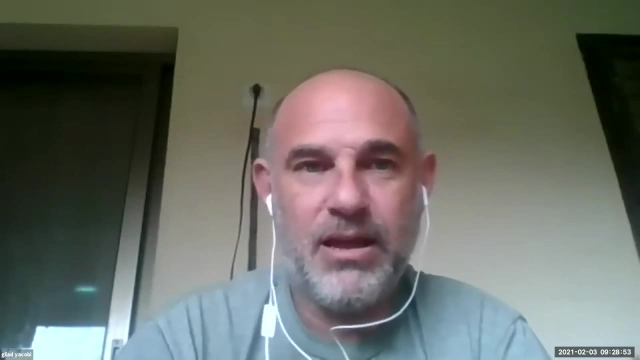 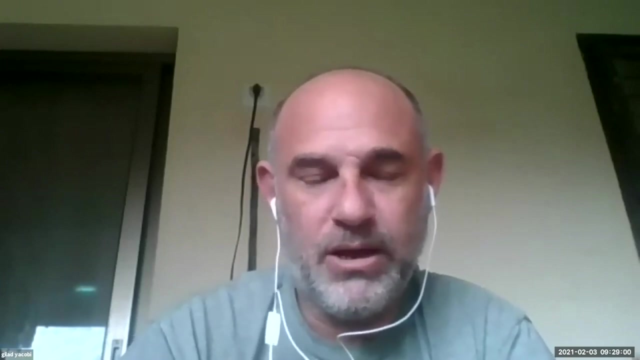 gila, yes, um, i. i wanted to know if you addressed them and the answers and if it was part of the the problem that they they didn't want to to talk about the issue, or if you didn't address the the answers, what do you mean? if i, if i, if i, um, um looked for the answer? 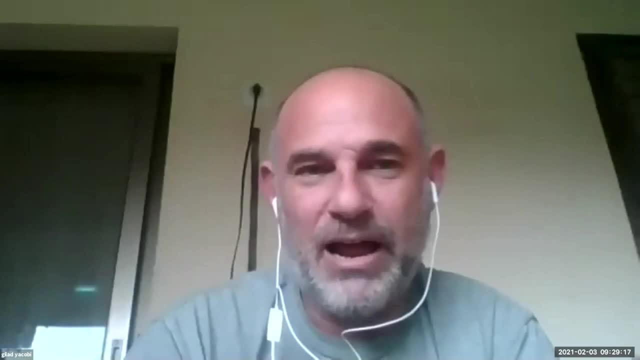 you, um, i, i, no, i i mean that i think part of the problem that the, the teachers don't teach about this problem is the problematic answers that may occur. so i wanted to know if you- if you address the answer as a problem or you didn't- um, we did, we did. we didn't judge this, the teachers. 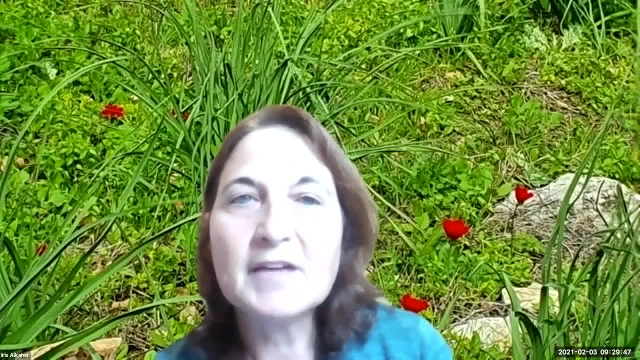 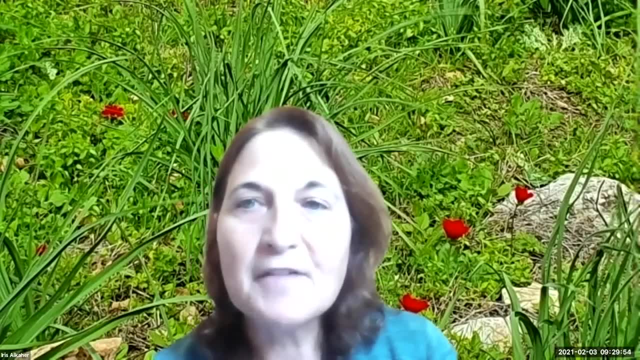 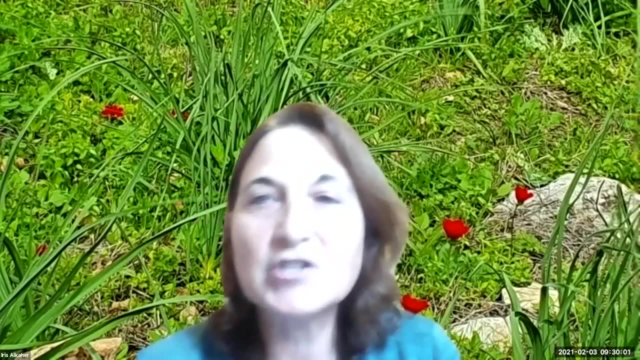 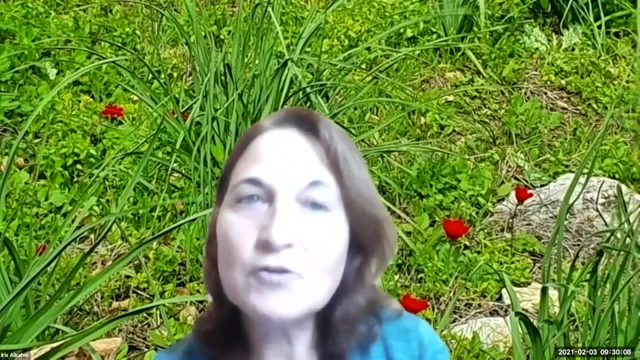 answers as problematic and it was a very it was evident that the teachers and the teachers um reported that this topic is controversial and they in in some of them um, are afraid to touch this, to touch this um, this subject, especially especially with small kids, but also but also. 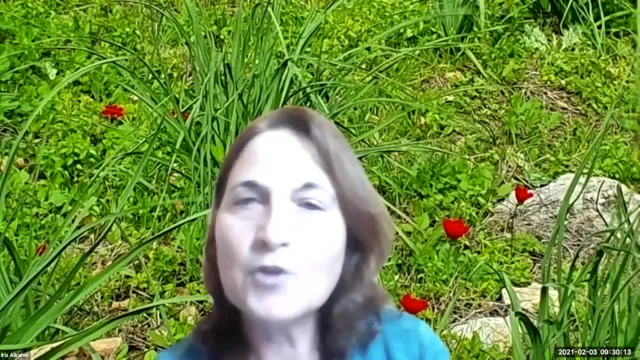 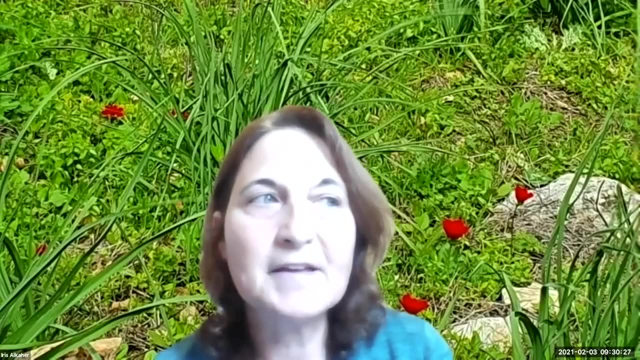 with youngsters in in in high school. not every, not only in the high school, but also in the high school, every teacher agreed that this subject should be part of his or her teaching. But it was interesting to note in the interviews that not only science teachers or biology teachers 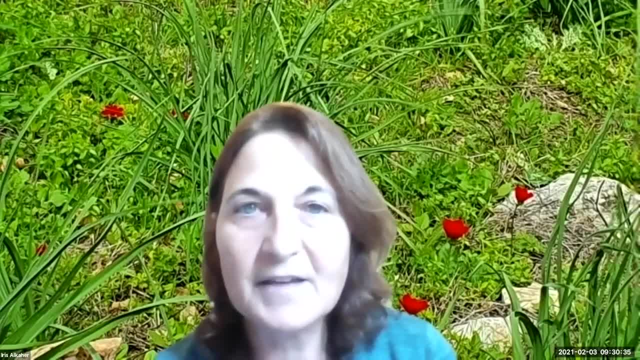 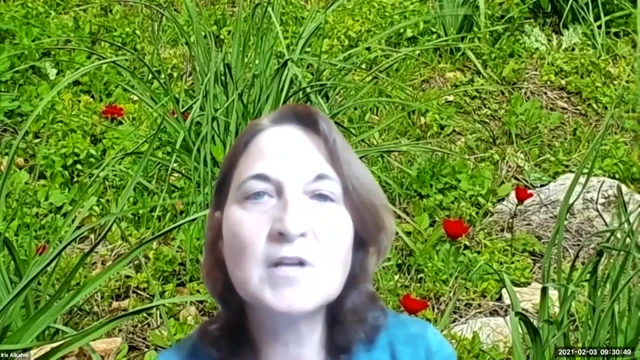 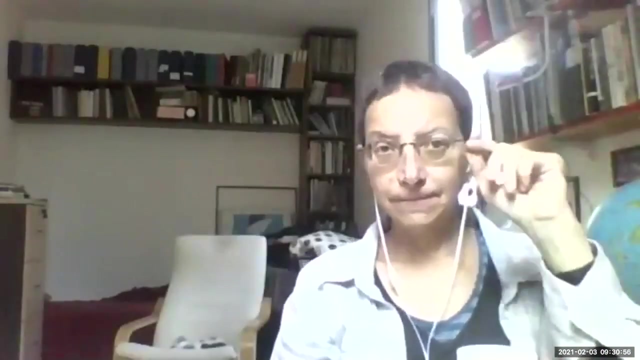 understood the importance of including this topic into class. there were also social studies teachers that understood that it's not only for science teaching and everybody should be exposed. Okay, did I answer your point? We have a question from Christina. Maybe you want to. 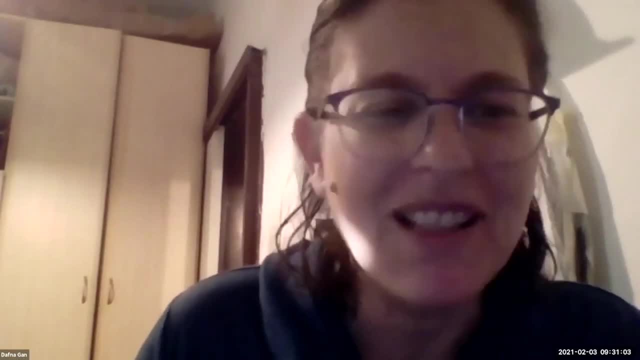 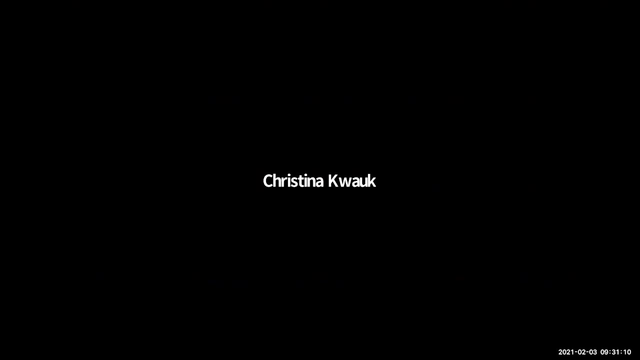 state or not, a comment. Christina, maybe you want to say it. Sure, I apologize for the noise in the background. We have online schooling going on behind me. I was just saying that it seems like I mean. Iris. you mentioned that this is a sensitive. 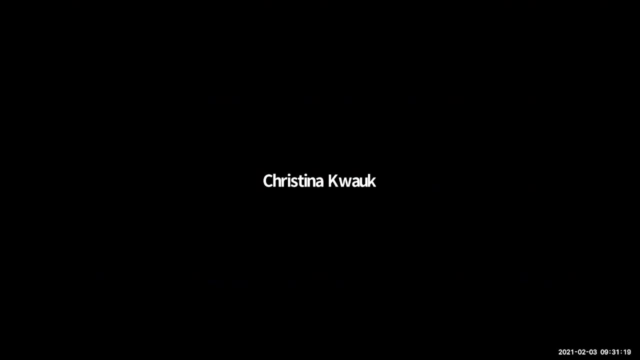 controversial topic and it's very clear that the teachers that you interviewed also sense this, but it seems like perhaps the real elephant in the room is really the discussions around reproductive rights, sexual education, women's empowerment potentially- and I'm curious how this came up or did not come up, or what are some potential solutions to resolving this, Because 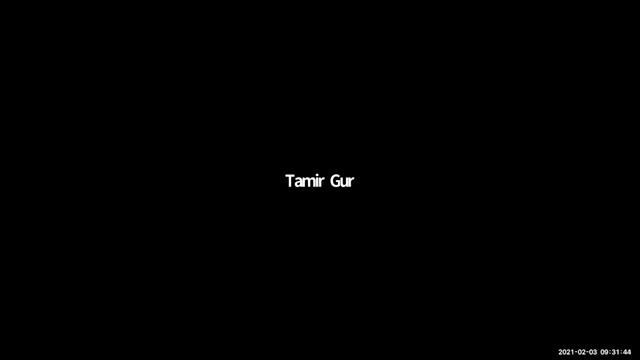 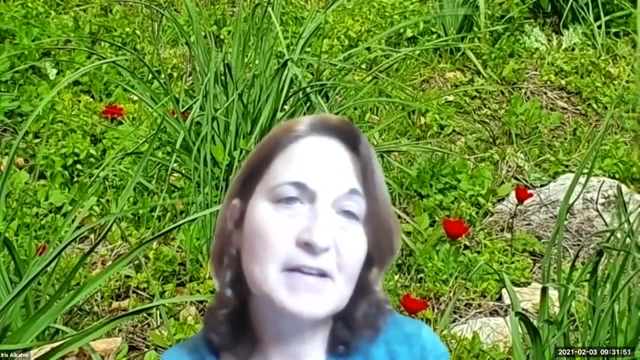 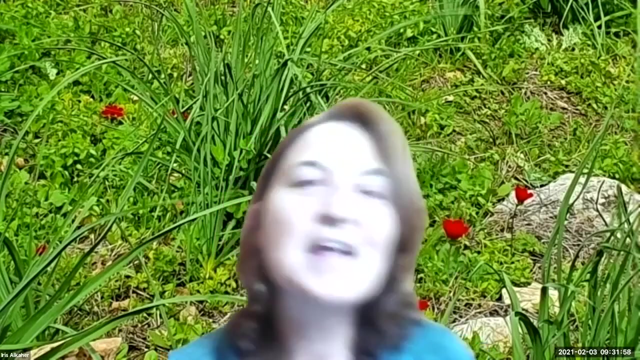 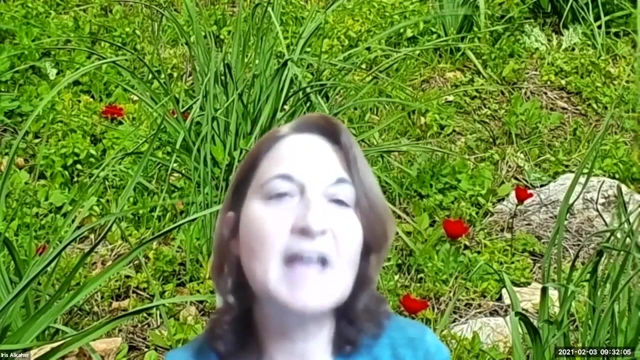 it's intricately tied with the notion of population growth. Thank you for your question. Well, actually the full questionnaire and the research that came after this research, the students who conducted seats here and Naama, so the full questionnaire also added items about teachers' attitudes, attitudes about human rights and women's rights. 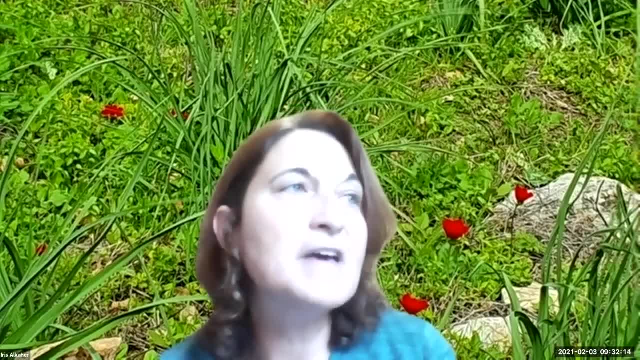 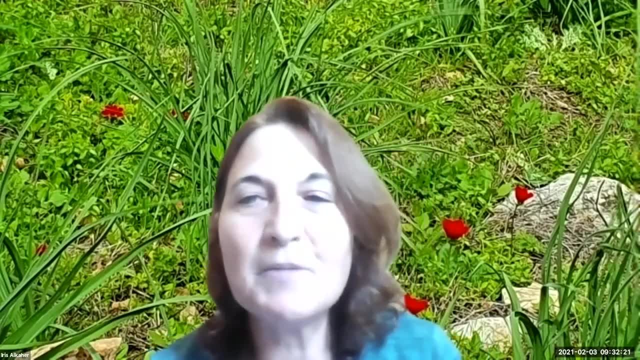 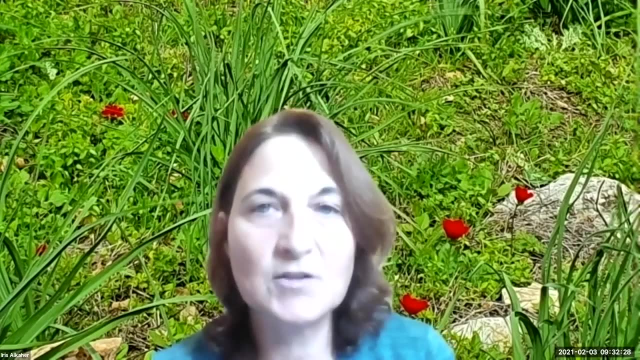 and that the state cannot say how many kids you will have. so all kinds of attitudes that are related to political, human rights and so on, and what we found out is that, in this sense, with these attitudes, the only difference that was evident in the results, the only difference between 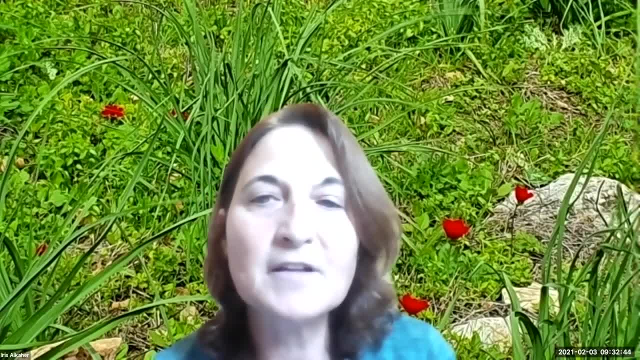 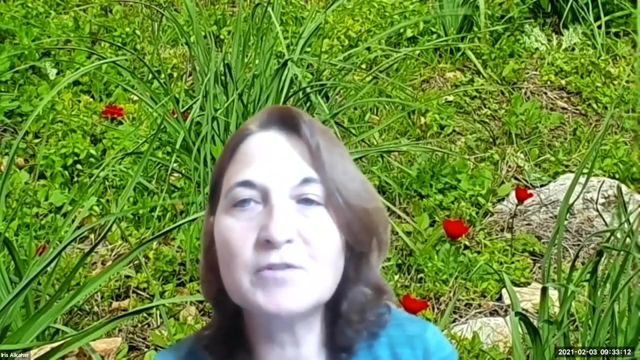 environmental teachers and non-environmental teachers. it was concerning the environmental-based attitudes. The other attitudes were similar in both groups and also in the interviews. the interviewees talked about what you are saying, what you said previously about human rights and human rights and so on. So you know, the decision about how big is your family is not the business of. 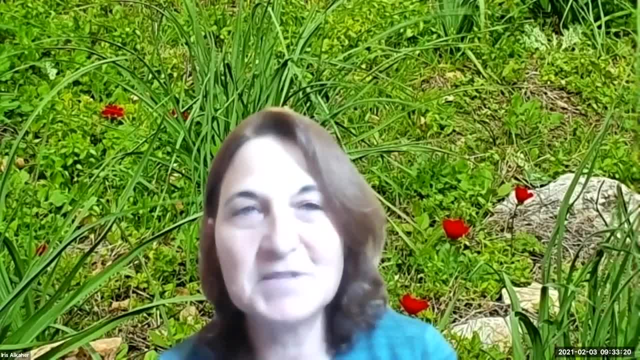 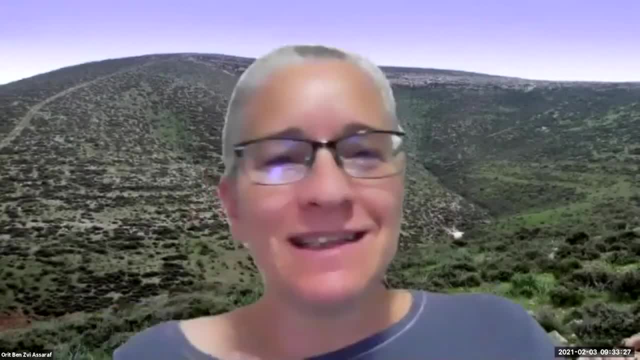 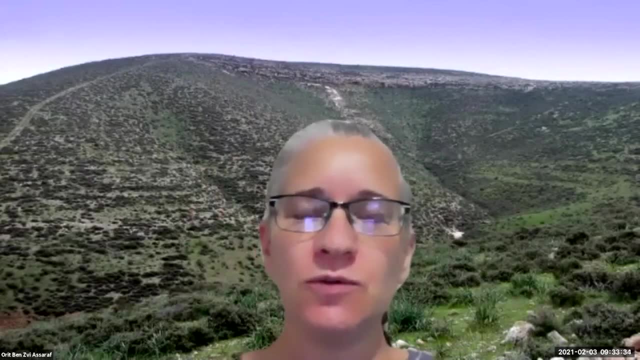 the state and other claims. Thank you, Orit. you wanted to ask a question. Yeah, thank you. It was so interesting and important issue. Iris, I wonder about the system thinking issue. In many research we don't really see connection between the level of 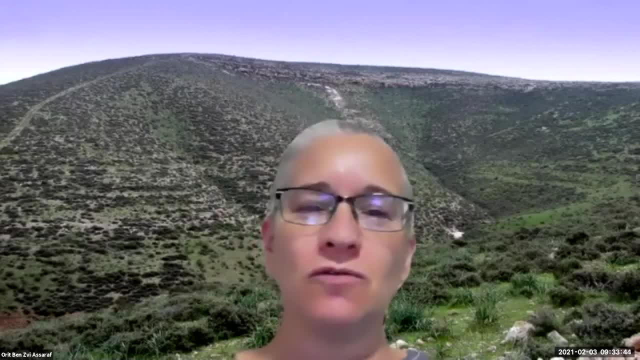 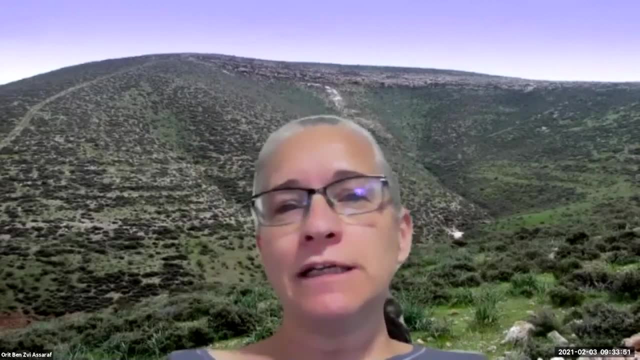 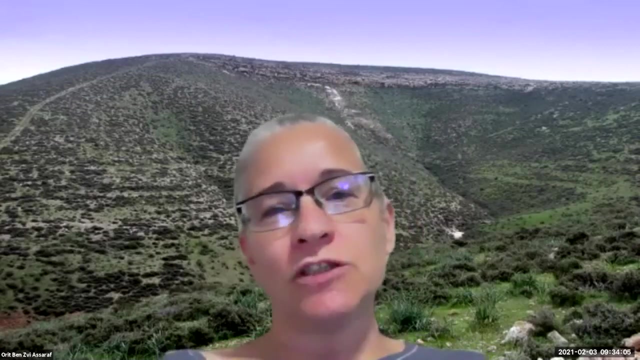 sophistication and or argumentation or cognitive skills or system thinking and ethical or environmental literacy. even So, could it be that someone will still hold non-environmental perspective of this issue, but still, all the very sophisticated system thinking skills or argumentation skills? Yes, it could be, Statistically. 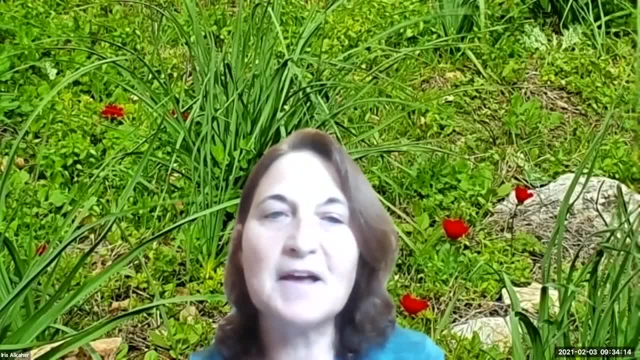 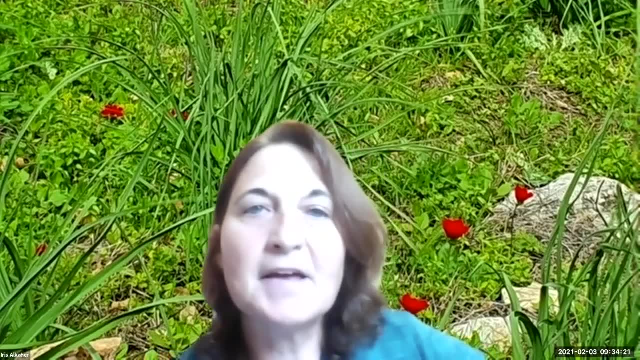 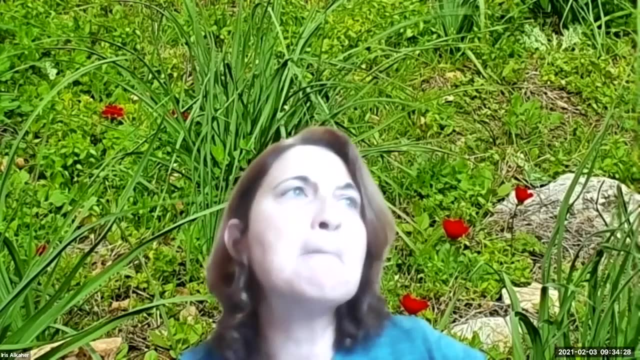 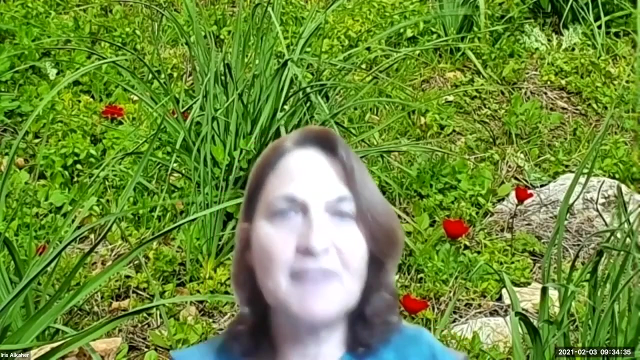 what we found is that the environmental teachers had a more developed understanding system, understanding with respect to what are the consequences of population growth, and they better understood the chain effect, or the domino effect, that population growth, if there is an overpopulation, so the impact is, for example, environmental degradation, and then it goes to them. 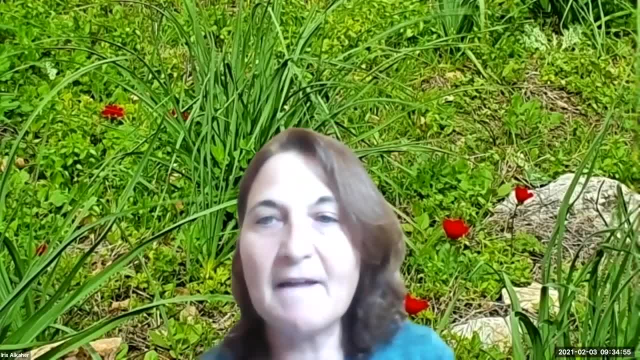 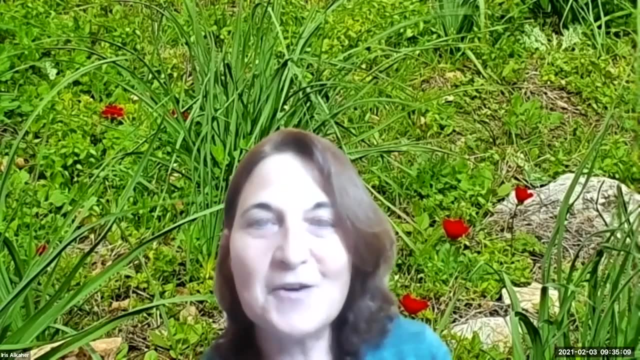 to specific pollutions and degradation in biodiversity and so on. So statistically, there are more environmental teachers who perceived it. It doesn't mean that, as you mentioned, that ethically or when you go to their %, they were willing to agree that birth rate should be stopped or should be reduced. 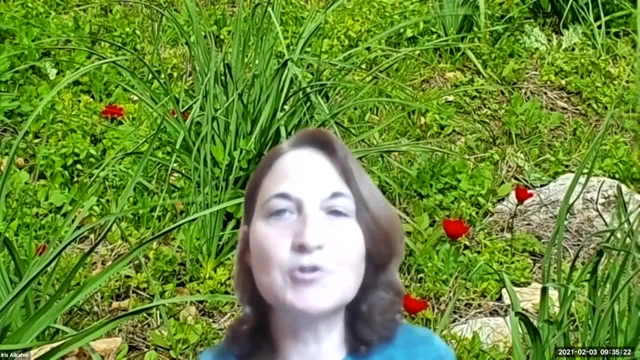 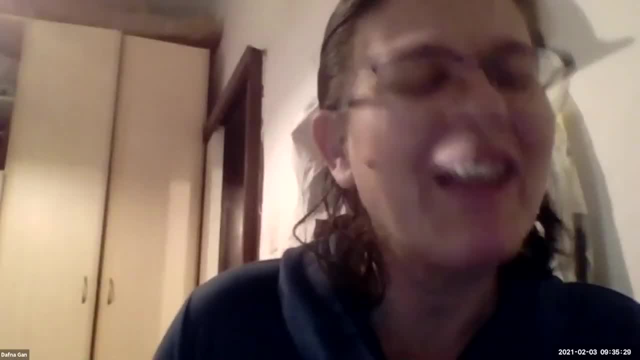 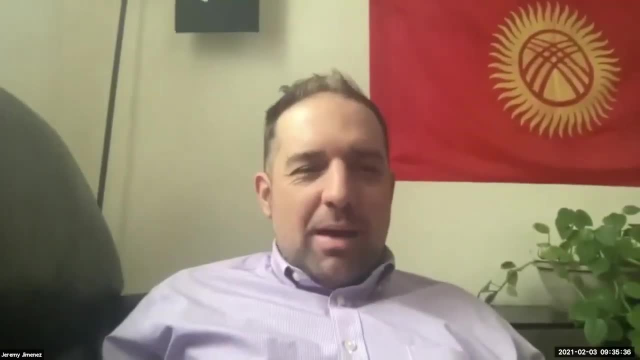 or should be controlled. Thank you, Jeremy. you're very quiet. You raise your hand. Yes, so I know your studies about high school teachers, but I was wondering if you could also comment on academics, college professors or international students. So what do you think? 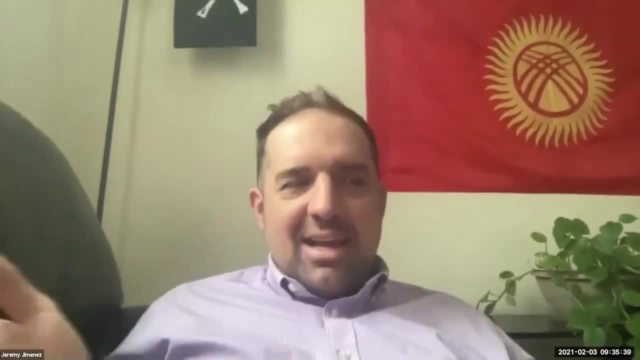 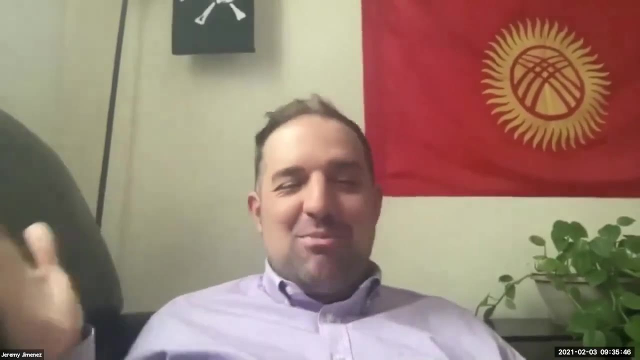 about these. I think it's really important to do a lot of research on these things, and they do. academics, college professors like I find. you know, if you even raised someone like Paul Ehrlich, you could easily be labeled eugenicist just for mentioning his name. So I'm curious to what? 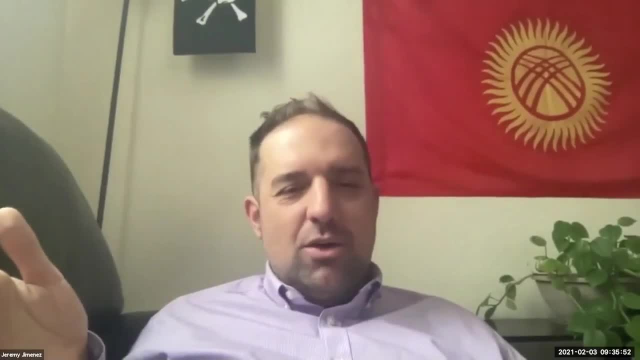 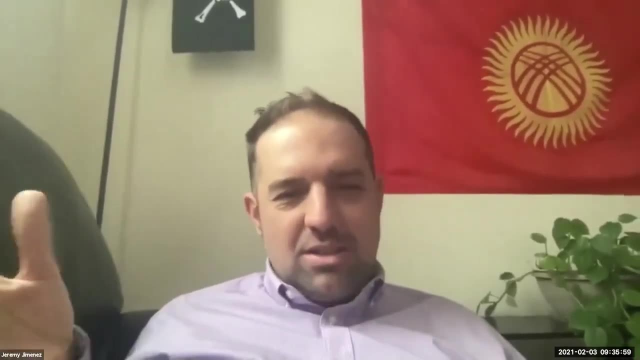 extent do you think, like professors, are adverse to talk about population growth because they're going to be labeled a racist or sexist again, given the racist, sexist oppression associated with population control policies? To what extent is it they're afraid they're going to offend? 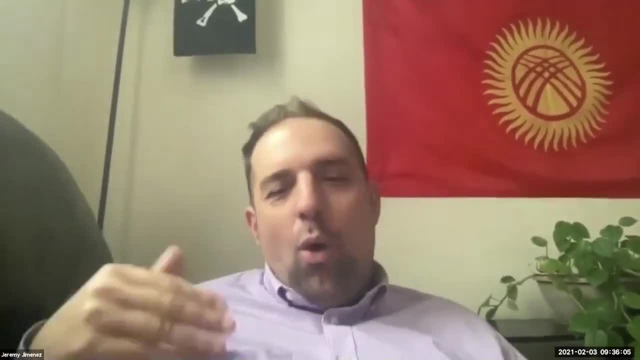 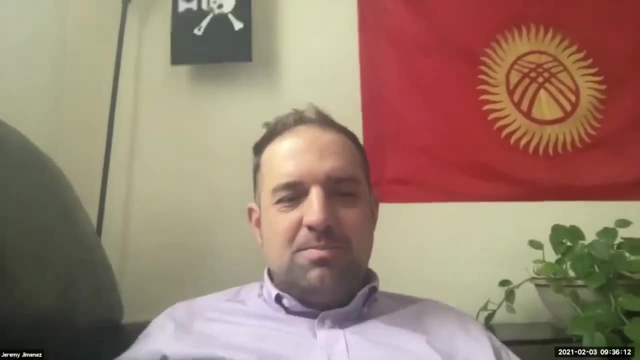 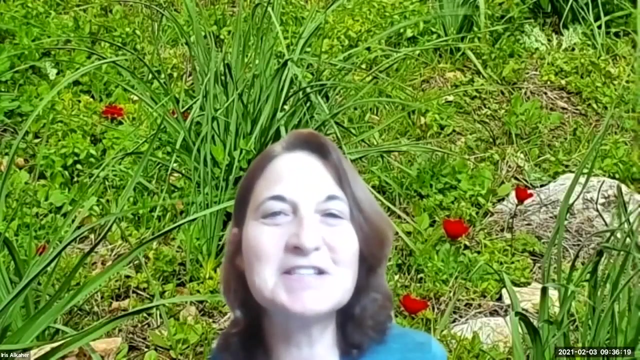 their colleagues who had children or want to have children, Or are they mostly, do you think, just not exposed to how detrimental world ecosystem health is with an ever growing population, Or anything else? Well, I believe, I believe that both both directions might be, might be true. 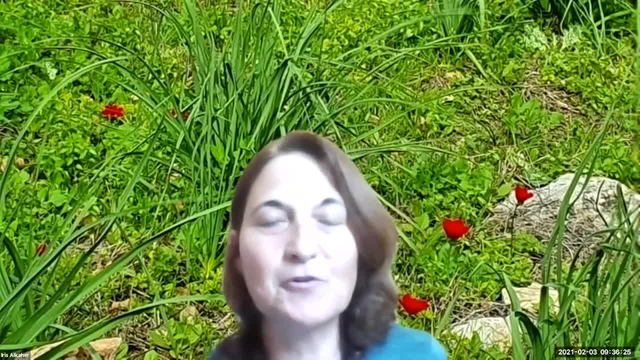 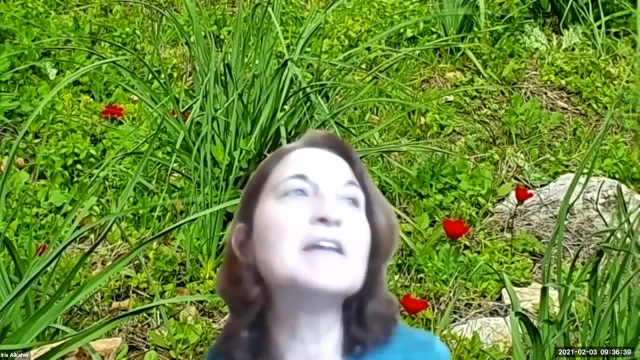 At least for Israeli professors or teachers. And okay, I don't know how it goes in the US or other countries. I'm curious, I'm curious to, to to know, maybe in the in the small, in the small discussions, But for sure, in the Israeli context, in a, teachers are not encouraged or not. 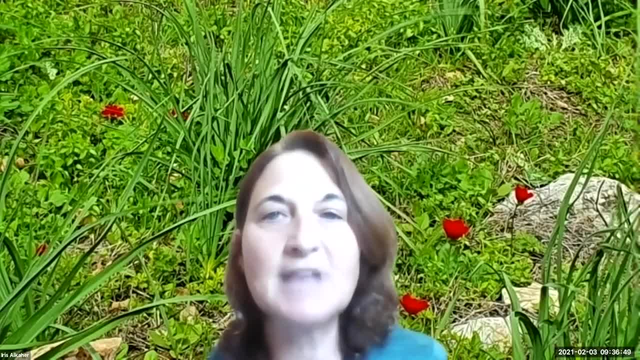 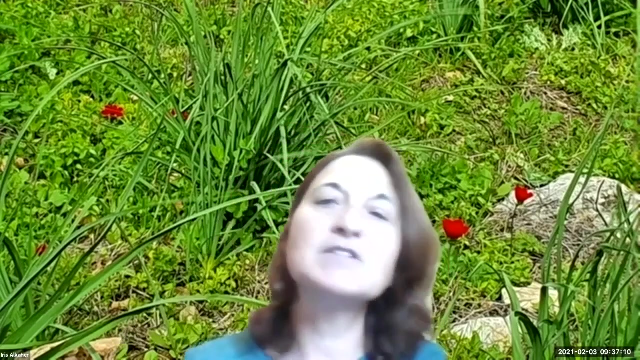 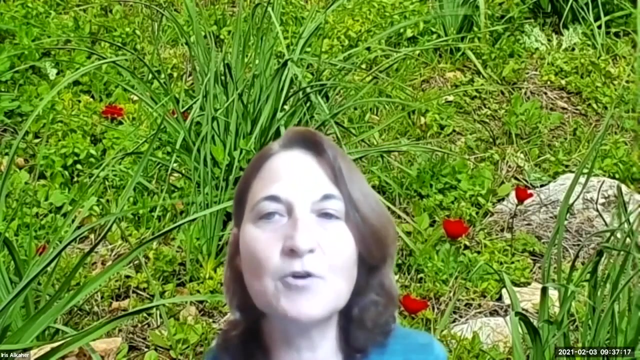 encouraged to talk about the about the subject as well as about other controversial a subject. And because they are a, at least in Israel, they are a strongly connected to political, to political issues or disputes or demographic issues with, you know, the majority of Jewish population versus the minority of Arabs and other minorities. So so it's very, very sensitive and teachers and professors really, in many cases, run away from this, from this hot potato. 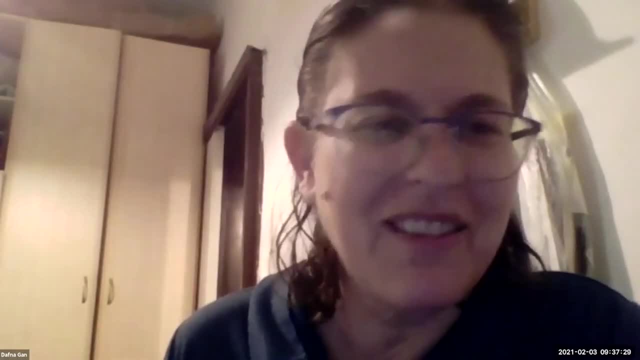 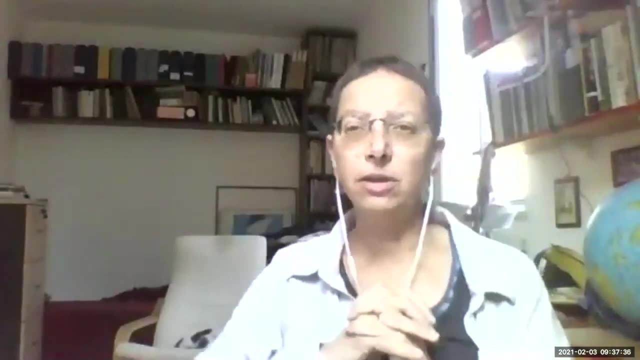 Thank you, Chagit, you're waiting too, And then Daren. I was thinking: many times this falls on the curriculum now. Thank you, Chagit, you're waiting too, And then Daren. Thank you, Chagit, you're waiting too, And then Daren. 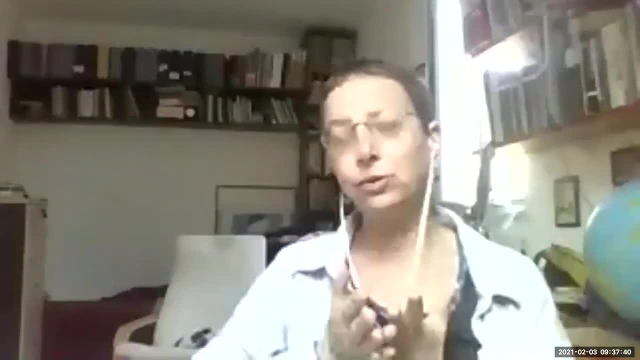 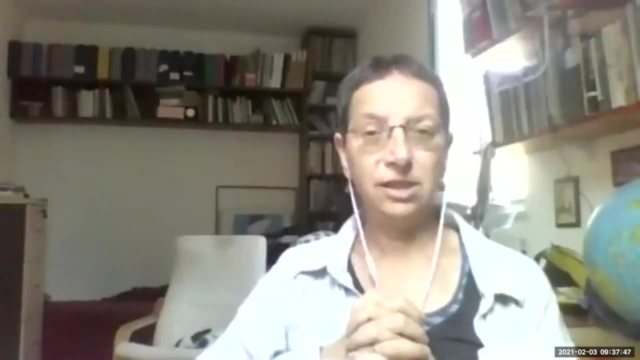 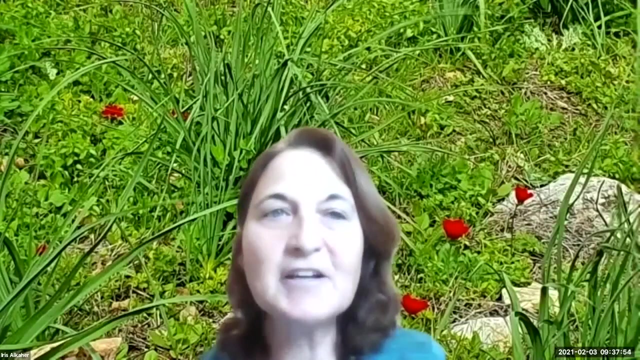 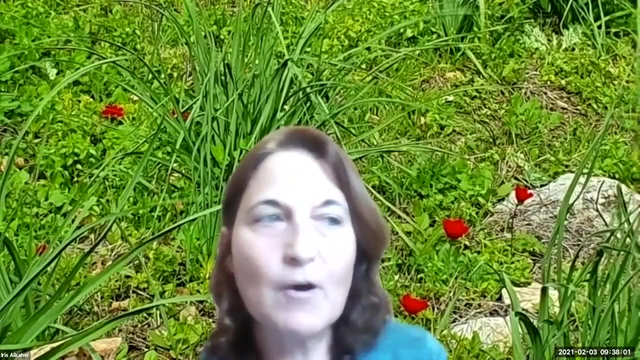 I'm curious about the curriculum and tools that teachers have. so are there any tools at all in Israel with for teaching this, for the teachers Strategies, content? anything Good question? There are. there are in geography, for example, or even in biology. there are chapters or a or specific concept, For example, in geography, the concept of 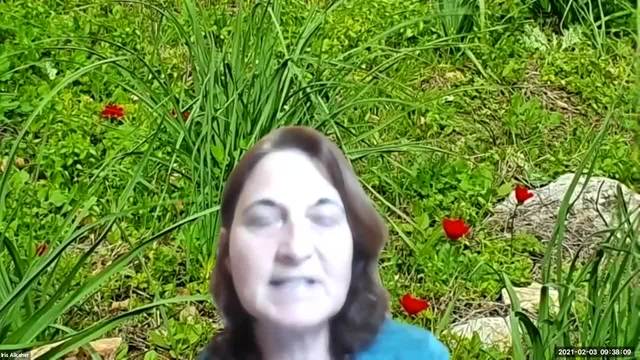 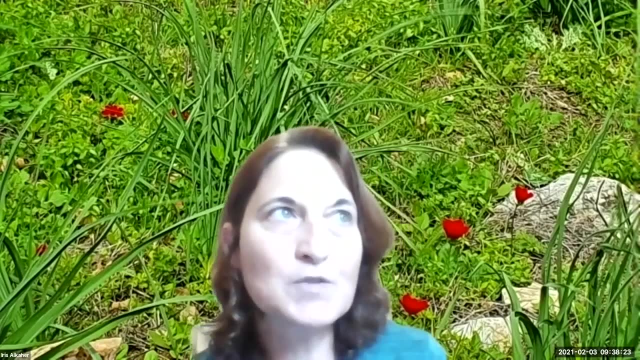 Or a or a specific concept. For example, in geography the concept of overpopulation or population growth is really studied, is in the curriculum, But raising dilemmas is less common. I think that a very useful tool or strategy is raising dilemmas. 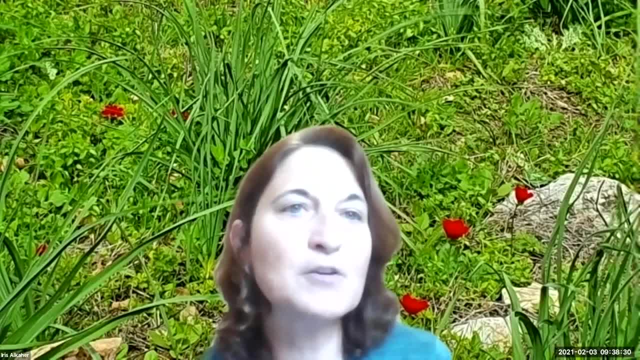 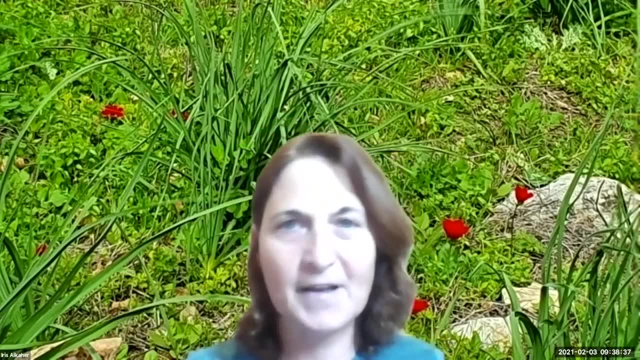 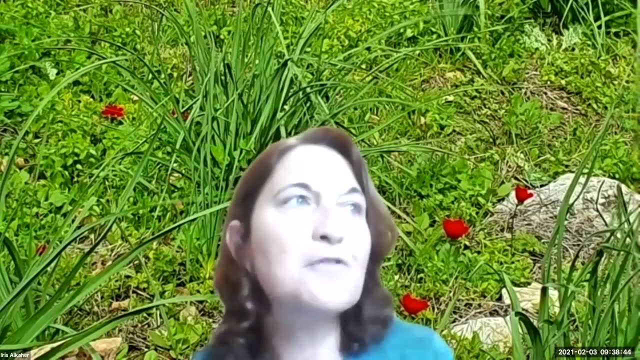 but not dilemmas which have the good and bad guys, only A dilemma which has diverse of actors and through raising dilemmas the students could think of it, could read about it, could present their diverse perception. I think students do it and in other subjects. 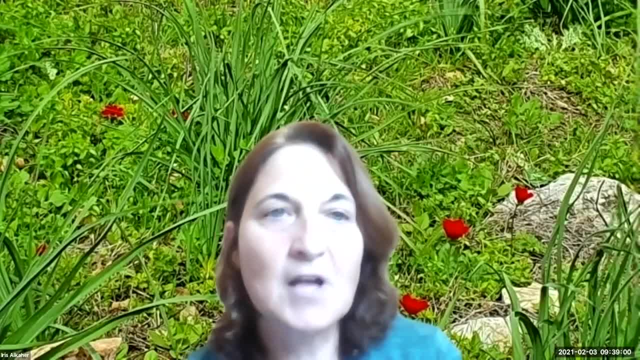 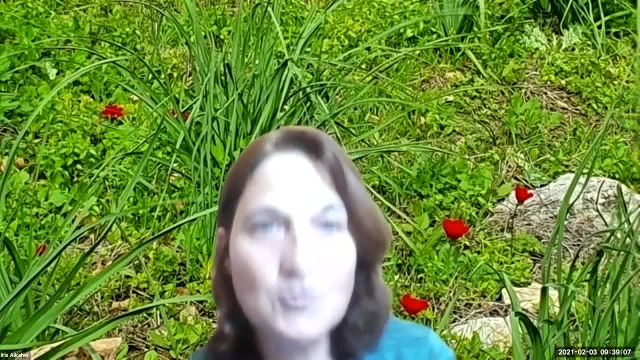 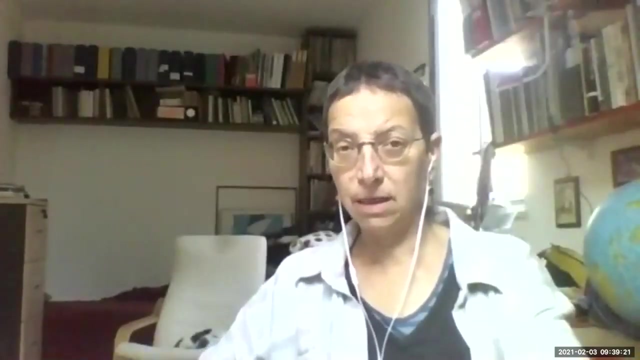 in science education in genetics, for example, there are social scientific issues that are well discussed in the classroom, So I think that the same could be with population growth and social scientific topics, But it still doesn't exist as a program or as a program that's written. 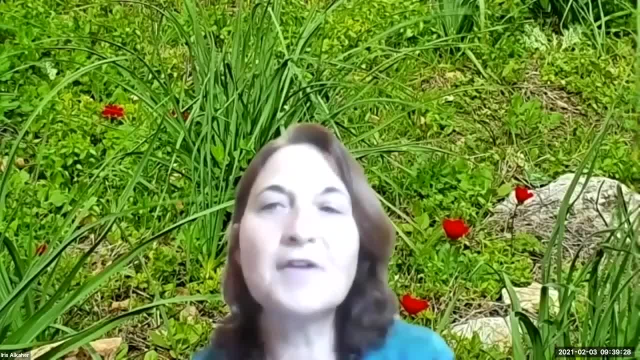 so it's not there yet? No, no, there are no. as far as I know, and as far as I looked at the curricula, there are no explicit objectives for teachers to talk about population growth as a problem or as a responsible for the environmental crisis, or as a major responsible for a major. 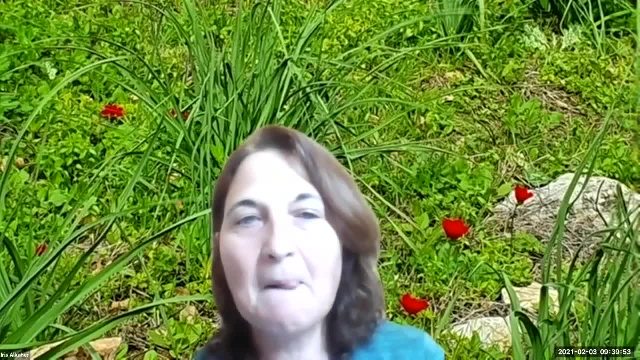 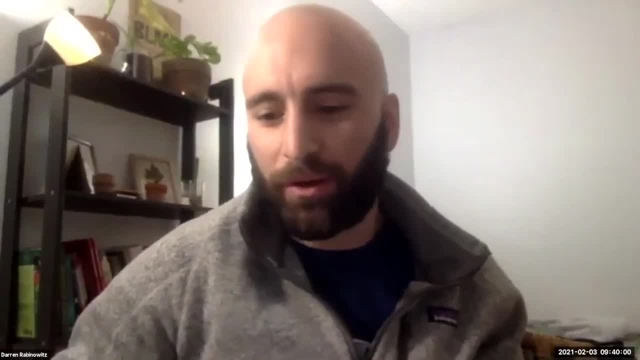 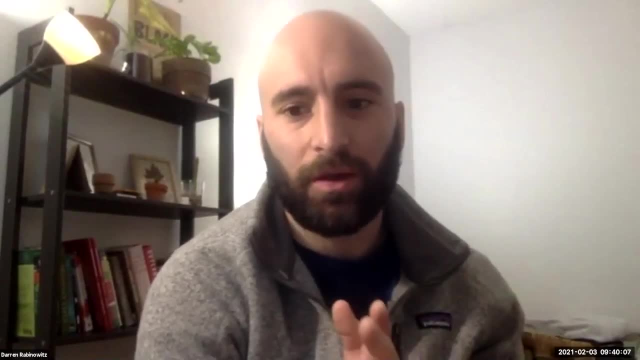 for the environmental crisis, Thanks. Thank you, Darren, And then Attila Iris. thank you so much. I have a question about if your participants overtly mentioned anything about like the religious implications for population growth and if they're, you know we may know that perhaps environmental education is more aligned. 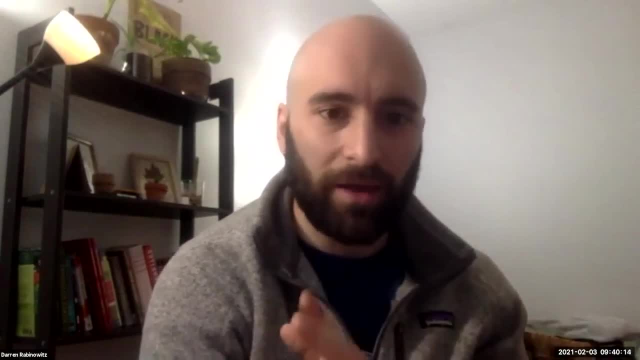 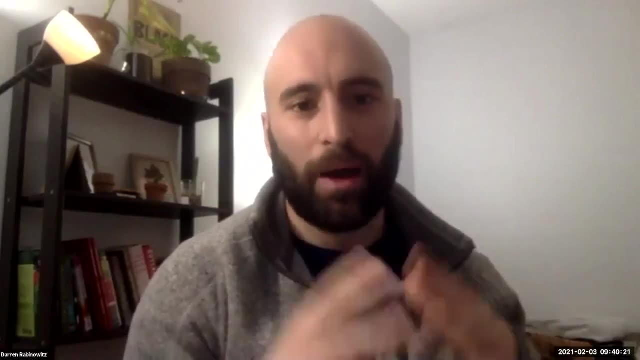 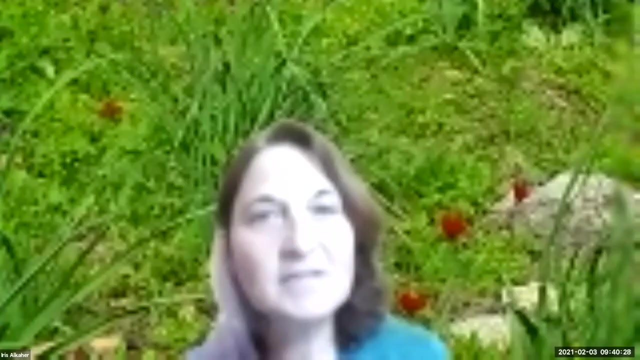 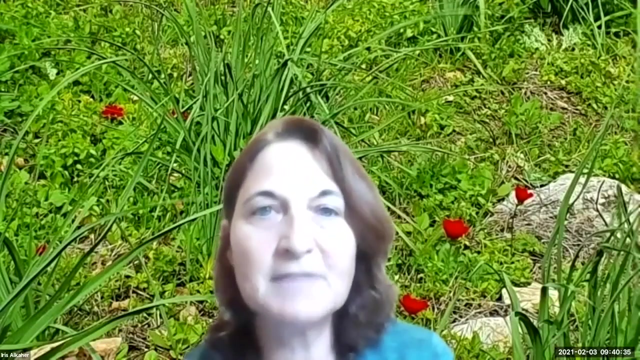 with progressive ideology or even maybe more secular life in Israel. I'm just curious to know if that part of the conversation was included in answers around population growth and environmental education ideologies. So I'm curious to hear your response. Yes, yes, it definitely came out. We could not split the participant into, you know. 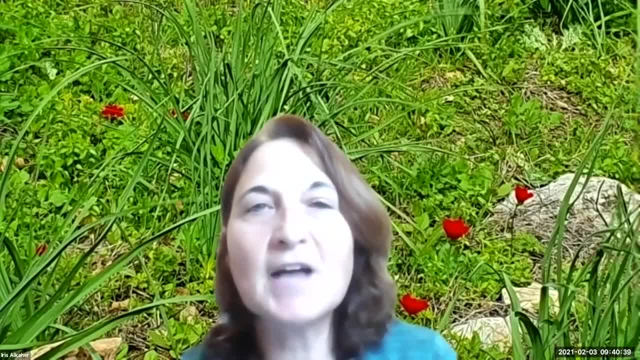 religious and secular or traditional, because you know the sample was not. it was not big enough, But in teachers' explanations and written answers and in the interviews, even the less religious teachers, some of them, several of them, did raise. 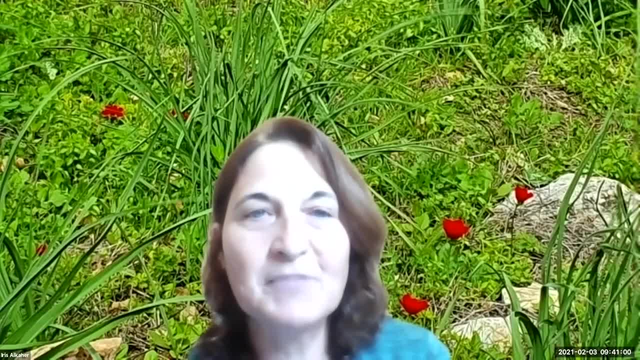 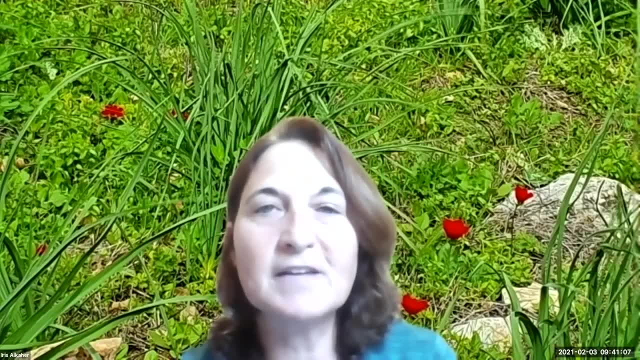 the. you know the conflict with the religious faith And in Hebrew it said: I don't know how to say it in English, but you know the encourage of reproduction, that is a command in the Genesis book. Yes, they raised it And I found myself, you know. I think that 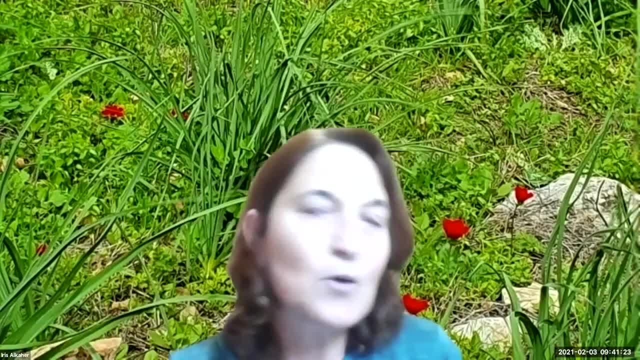 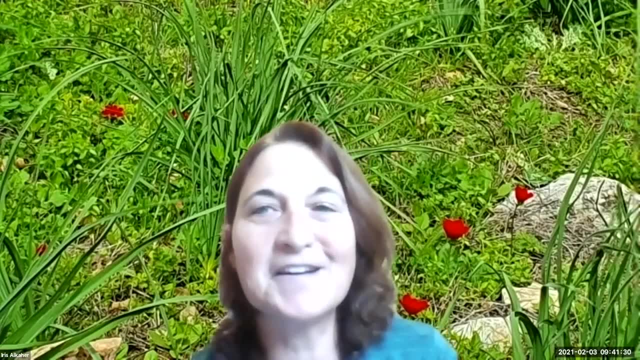 it was similar. it was similar to the, you know, to the problem of evolution, education, that when you want to deal with it, a similar concern raised. But also I found we found in the research many similarities with teacher perception and even religious one concerning the climate change. 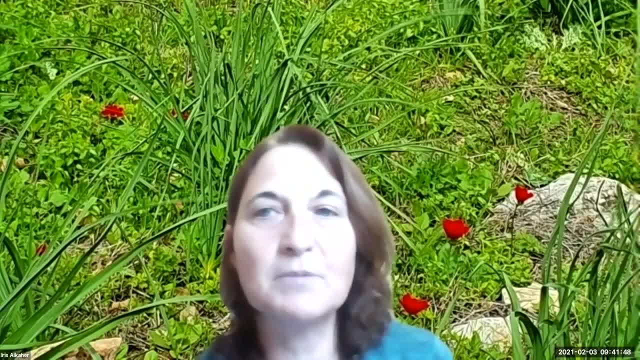 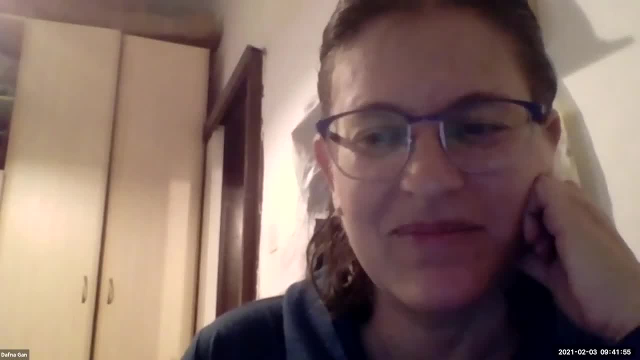 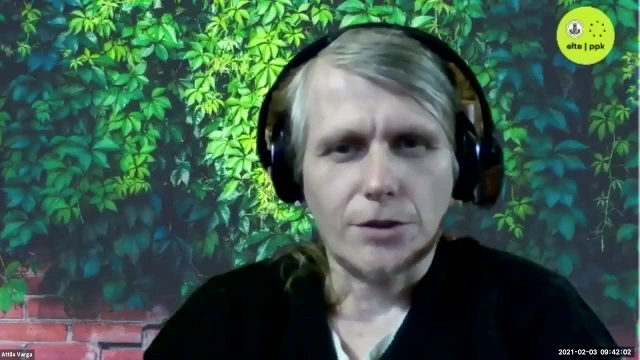 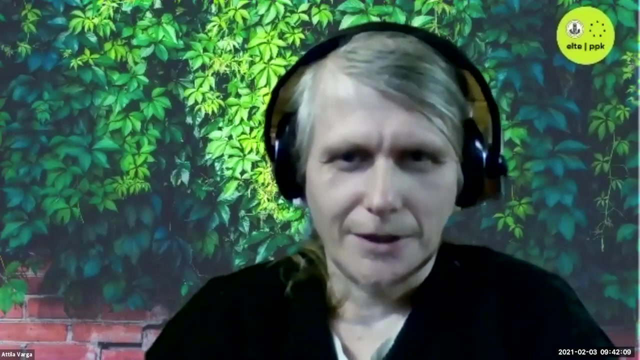 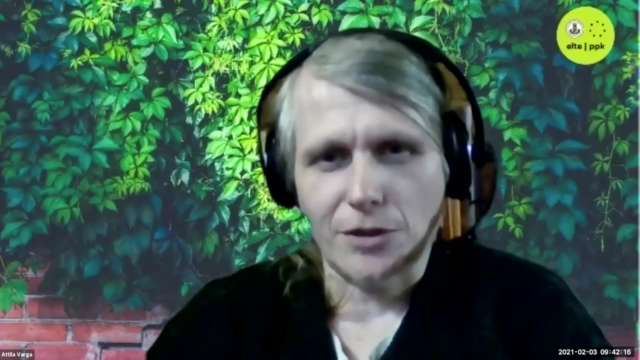 I found very many similarities between these two topics. Yeah, Thank you, Attila. Thank you very much. I'm very interested if you have any international comparison of this data, because I'm coming from a country where the population is actually decreasing, And if there is anything about population growth in Hungary in education. 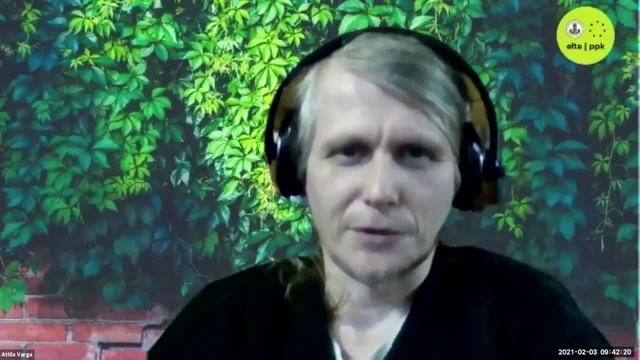 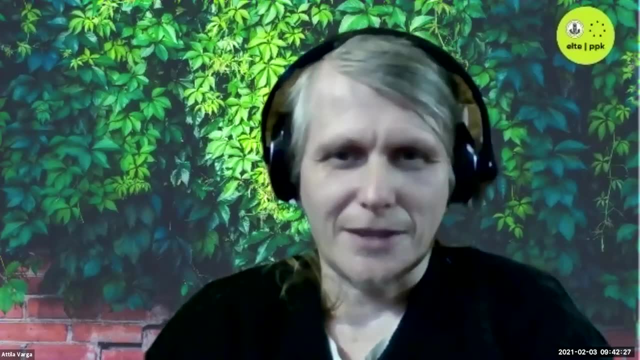 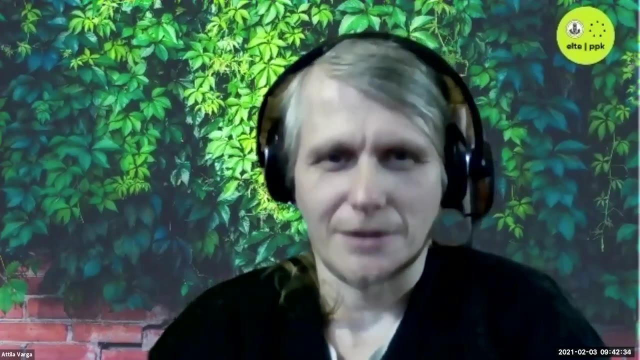 it is about to increase the Hungarian population and not to decrease it. So that's, and I'm interested if you have any suggestion for including population growth issues in a country where the population is decreasing actually. Thanks for the question. Well, actually. 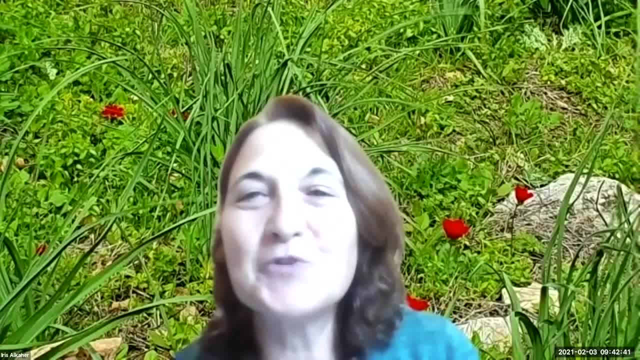 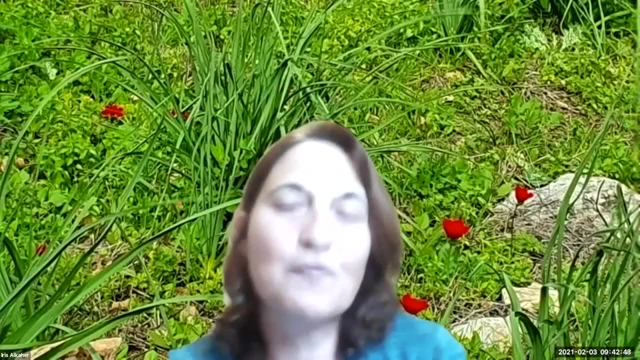 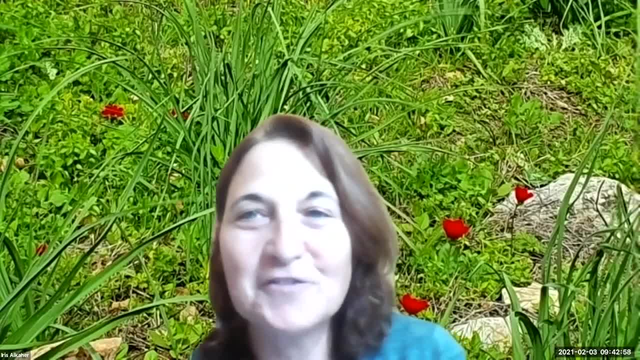 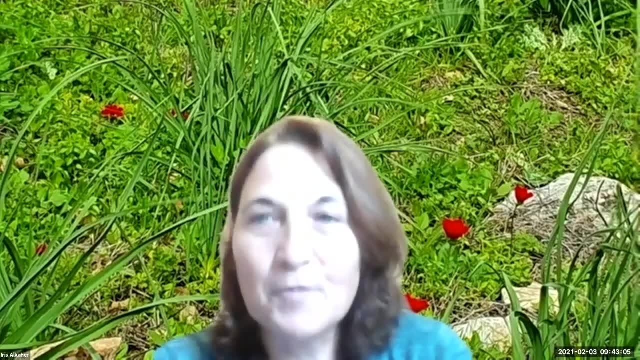 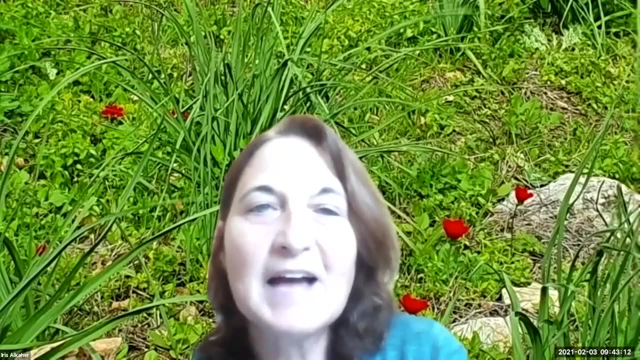 they say they want, they want to encourage the the population and not decrease the population, because they don't see that there is a problem of, of of overpopulation. So this is, this is the next step, But I know that there are differences. That's why I I emphasized in the beginning of 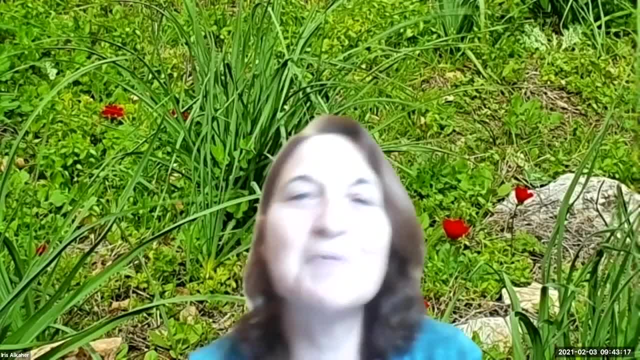 my presentation, the unique or the unusual phenomenon in Israel. this sense, because we are also considered, you know, at least considered as a Western country, But the international original state, but usually the Western leadership, is oil, rather, you know you. 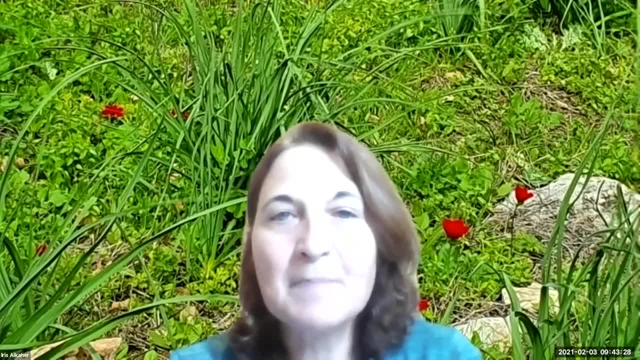 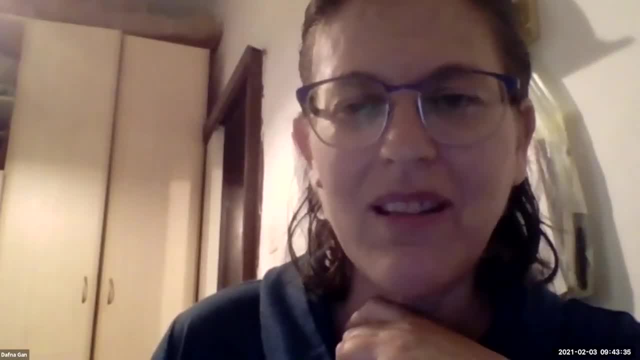 know none by choice, So I hope we can secure people watching the webinar in any sort ofília MOOC. this a subject. this is something very unusual. i think we will do. you want to say to ask something before we? uh, yeah, i know, i know we want to move to the breakout session. first of all, thank you for 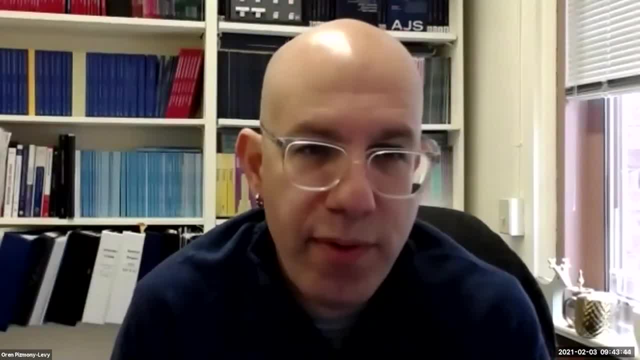 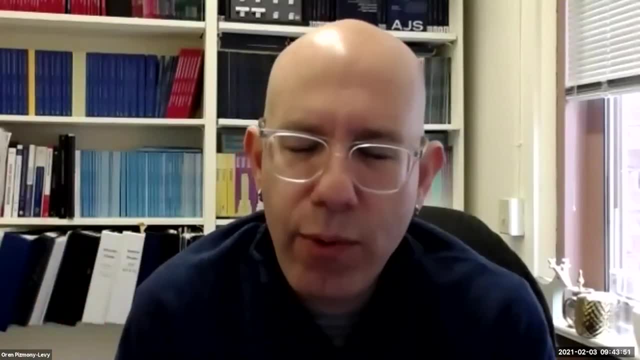 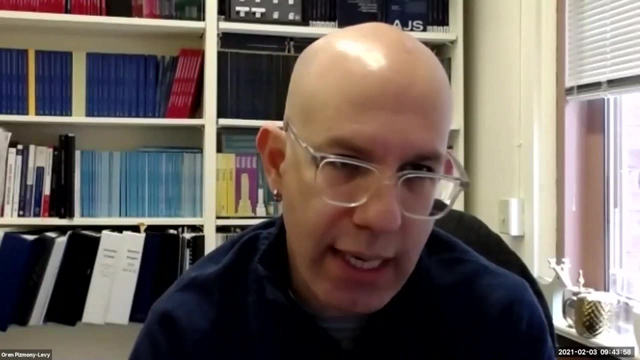 the talk. this was fantastic and i had the chance to look at the paper before, so i i appreciate, uh, hearing you speaking about the logics of the different pieces, but i wanted to make a quick comments, or maybe it's a question to connect what orit was asking and what christina was asking. 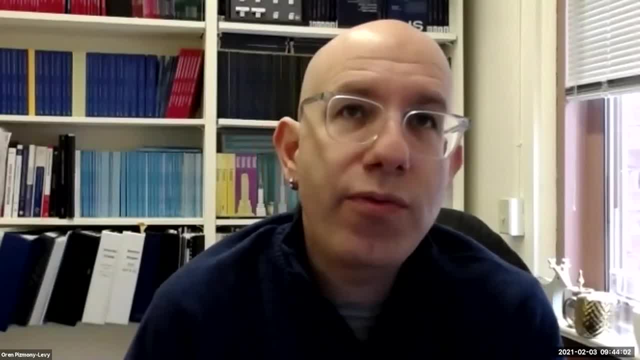 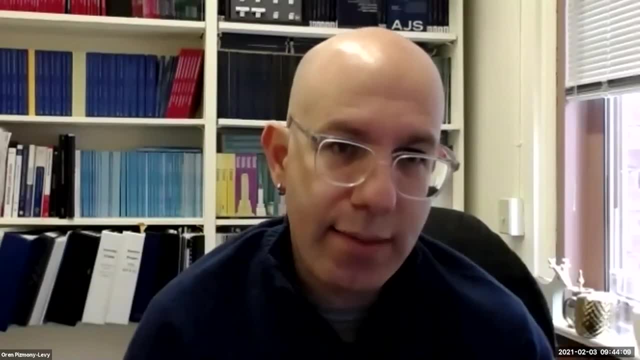 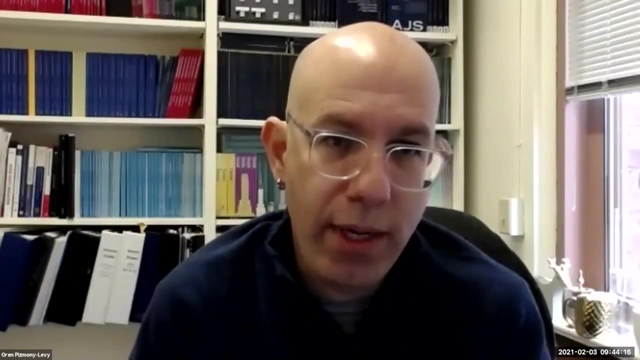 about system thinking, because it seems like, while you find that the environmental ed teachers have more system thinking around environmentalism, it seems like they don't have the system thinking that we need when we talk about sustainability, that connect the human, the economy and the environment together. because if they had that, i would expect that they would show different. 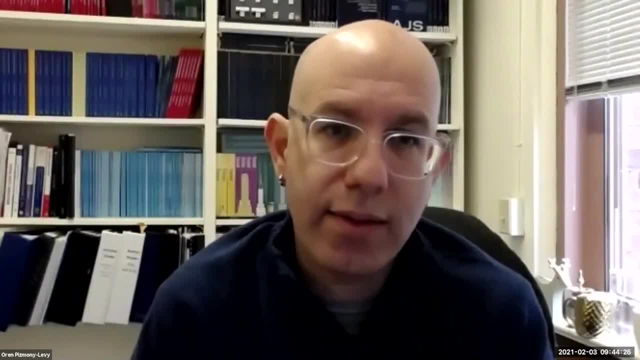 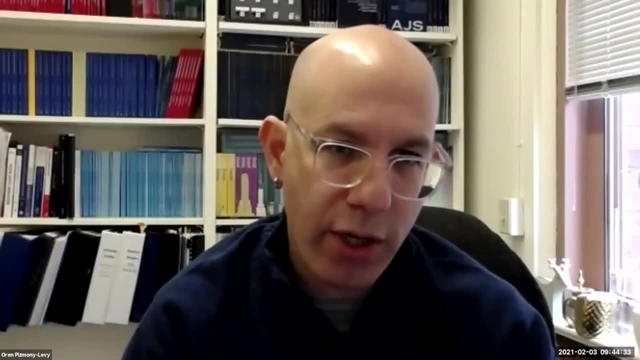 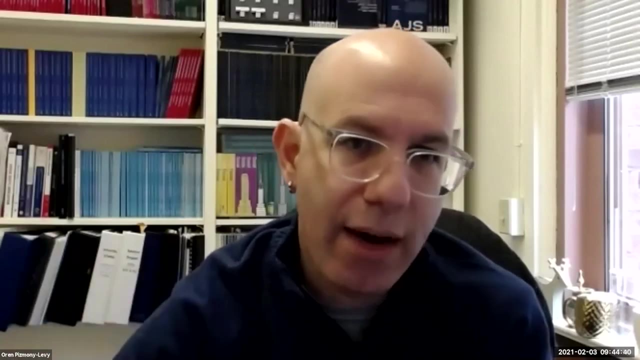 attitudes on the issues of women's rights, uh, empowerment, etc. so i wonder if that's the next part it's. is that the next paper we are going to see, something that will connect these attitudes as well, or are you moving on to increasing the sample size? i'm just curious about how. 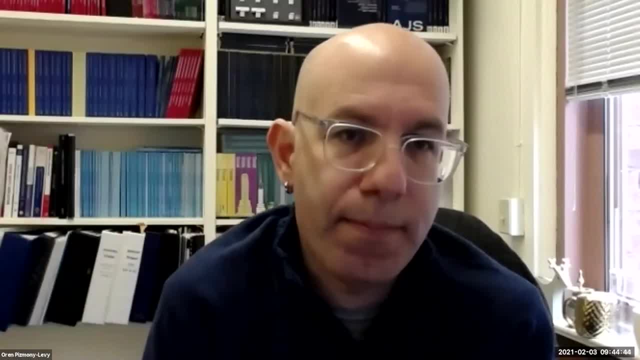 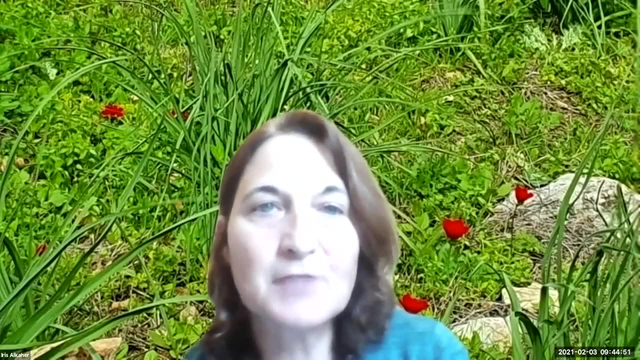 to address this puzzle around the system thinking piece. this, this is, this is the. the next step, this is the second, the second day, the second day in a study that really connects between the, what you have, what you have said in teachers attitudes concerning all the issues that you. 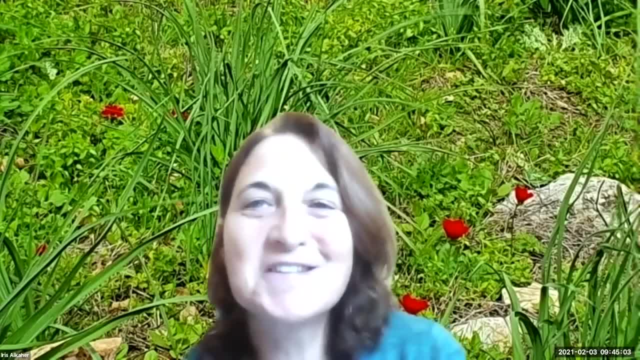 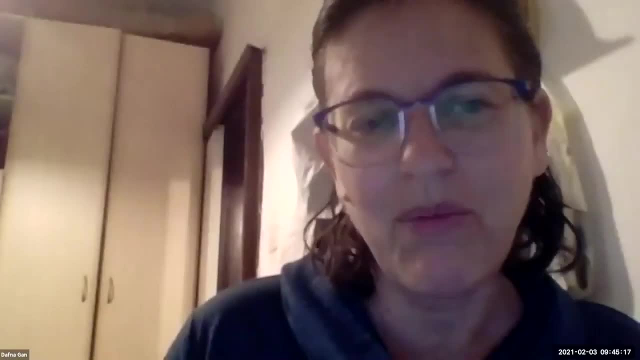 raised and in their system or not, system thinking with respect to environmental a problem, and i think this is a good comment in a good day, in a good direction to focus on. so, thanks, great, so we will move on and, uh, we will now break out. oh, and i think, uh, six rooms. 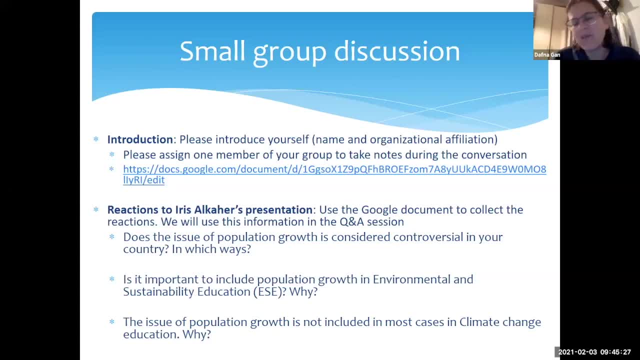 is, it will be good and we will have a small discussion in the breakout rooms and we have three questions. we we would like to have some interaction and a really engaging discussion. so if you can introduce yourself and then assign someone to take some notes, i put in the in the chat this link to the. 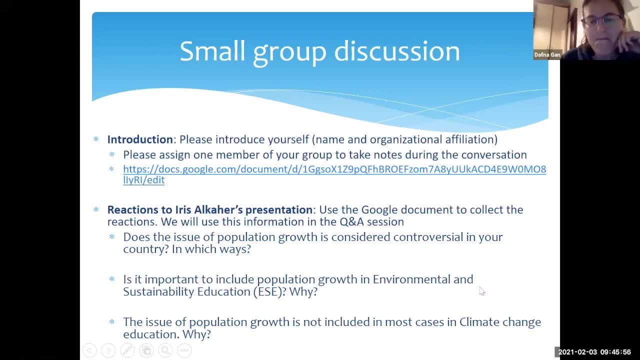 google docs, that we collect all the uh, all the discussion from all our meetings. and uh, we have three questions about uh, uh, to, to, to look about if in your, in your country, there is a, a consideration of population growth. and uh, do you think it's important and why, and maybe 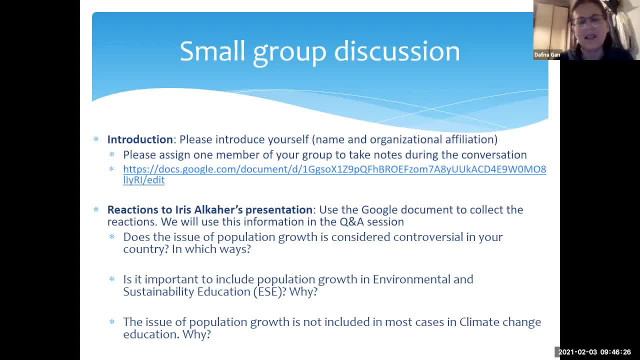 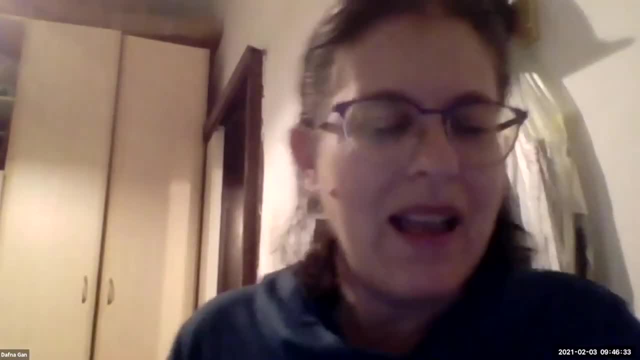 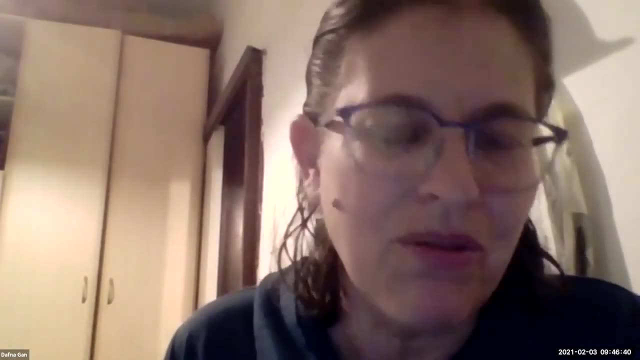 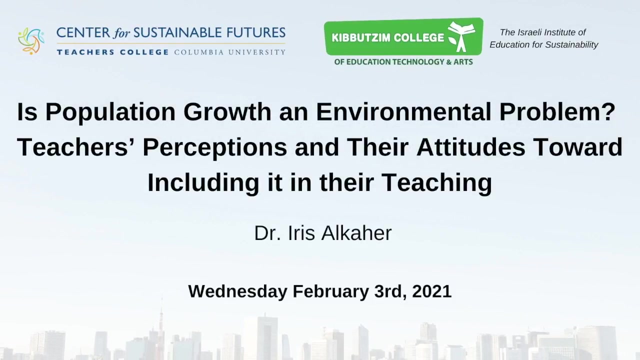 how we can connect it to climate change. so this is some of the questions. if there are other questions, uh, of course, more than welcome to raise it, and we will meet here in about 25 minutes, half an hour back, to conclude our discussion. great, so we will be happy to hear. 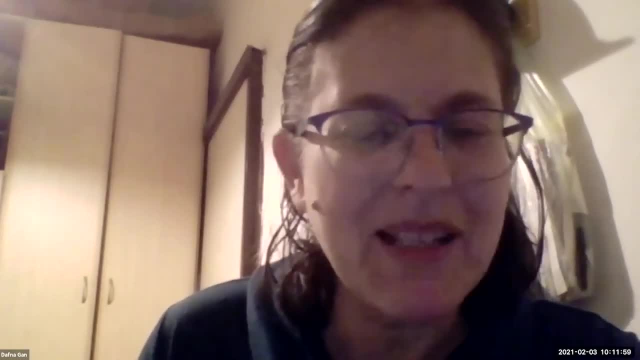 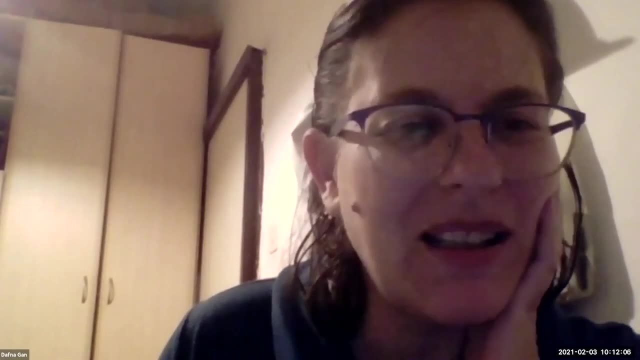 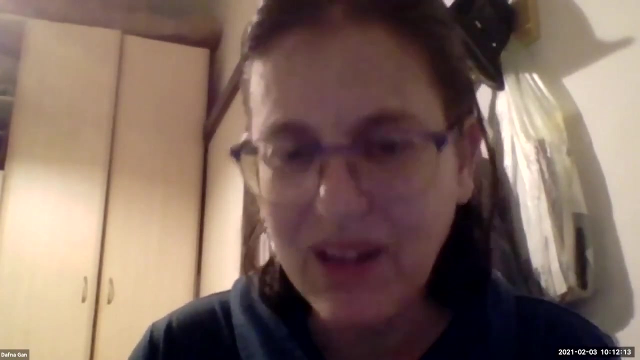 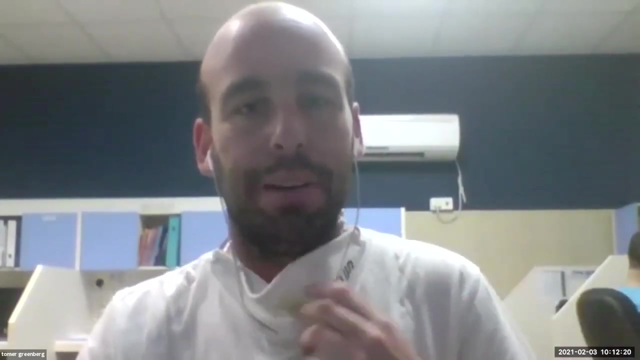 uh, some thoughts about your group discussion, some ideas that uh, you discussed in your group. uh, is someone from a group one want to share with us? uh, tommy, do you raise your hand? yes, great, uh, in in my group. i started to say something and then, before i complete my sentence, i: 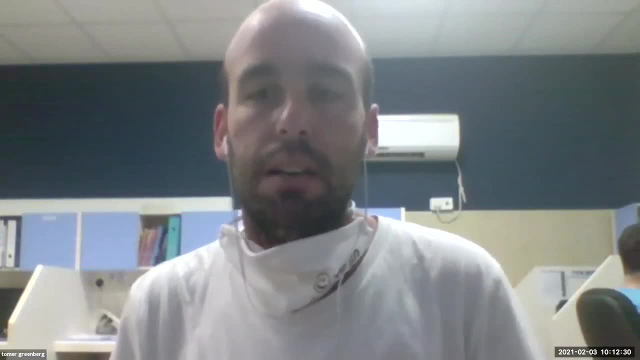 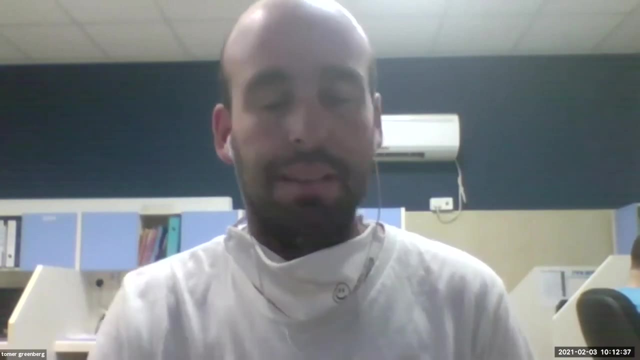 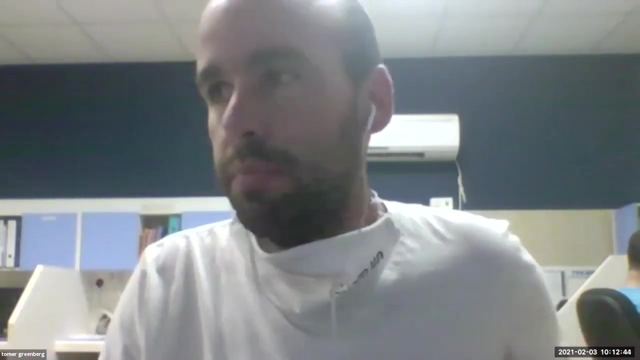 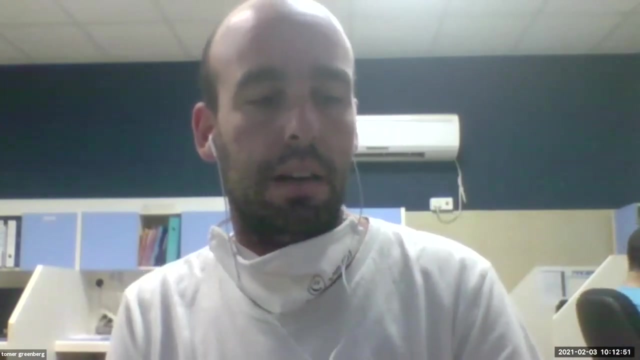 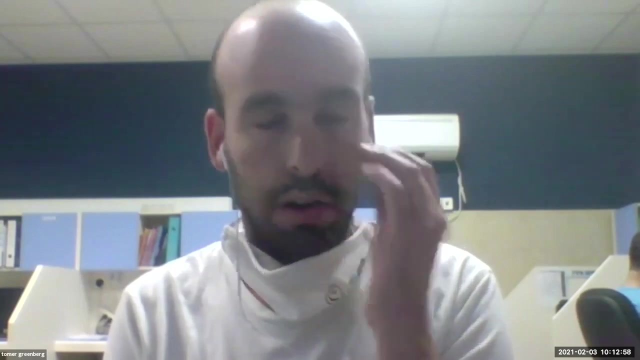 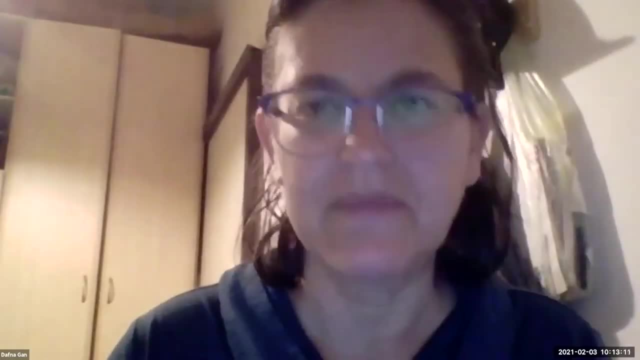 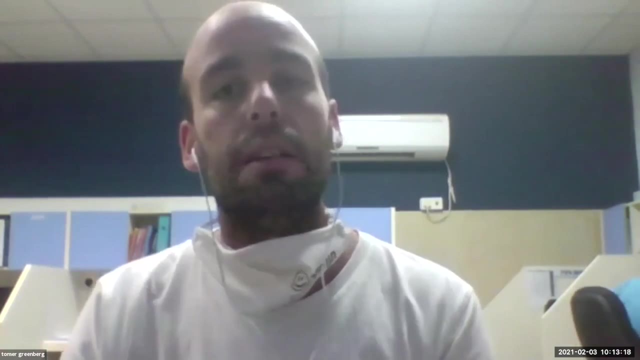 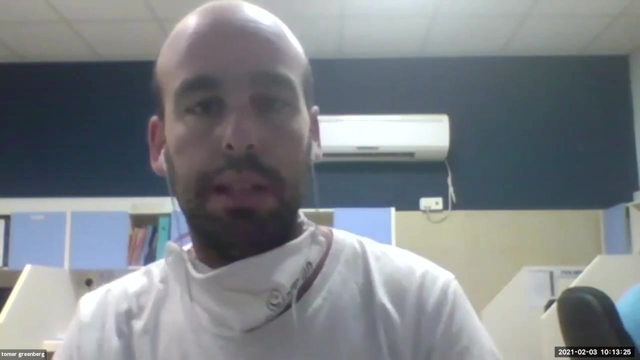 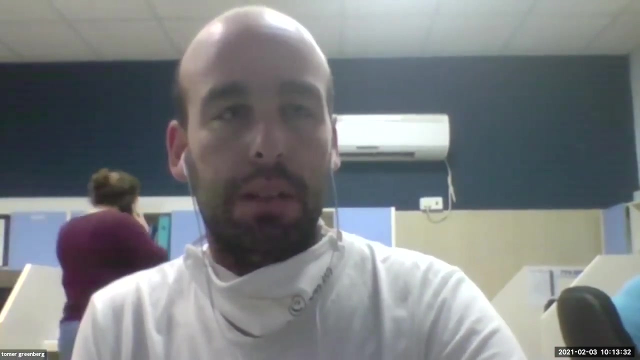 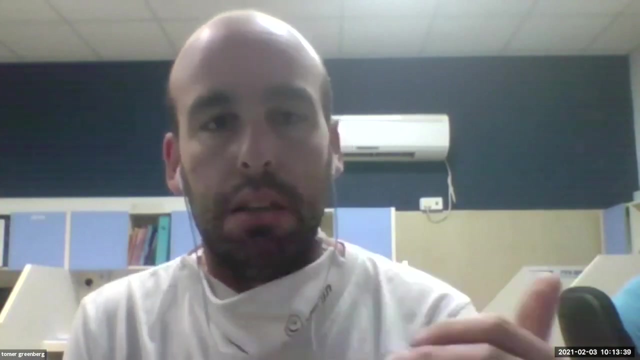 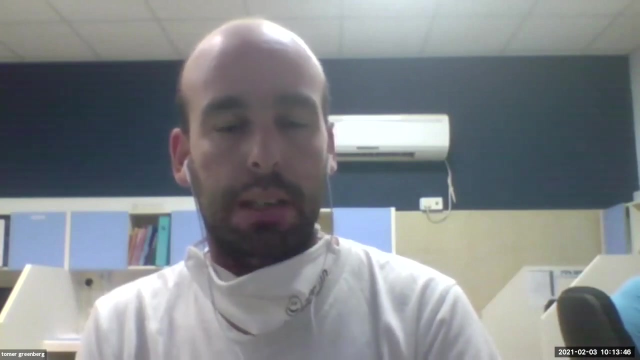 events, events that make us make us need to survive and make more children, and we we need to have more children because we need to survive, and uh, etc, um, and i, and i wouldn't wanted to say ah, before, before this, uh, someone say that, um, that the, the footprint is the, sometimes, um, sometimes it's related to the number of 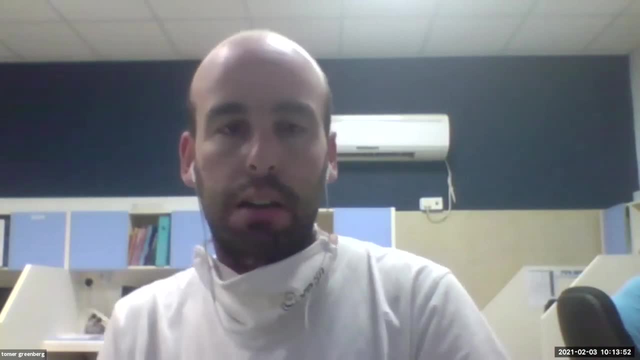 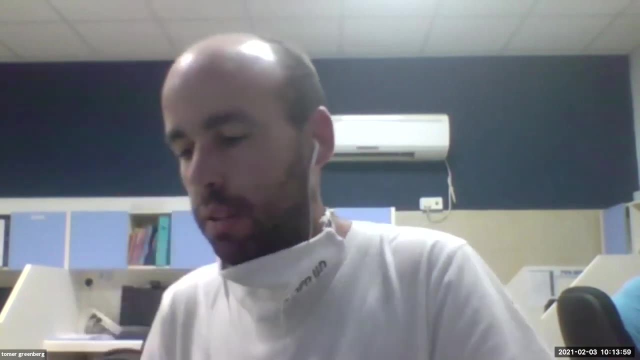 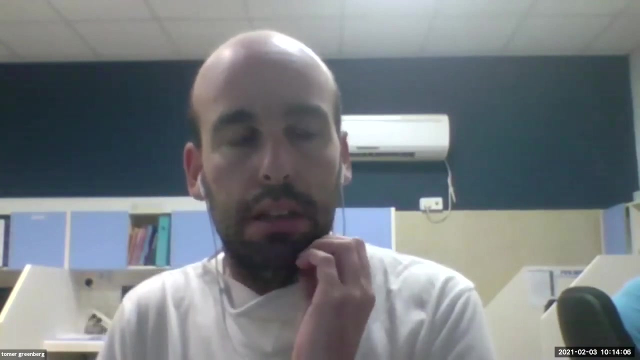 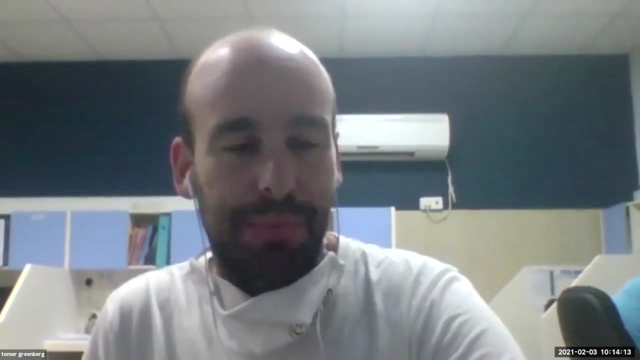 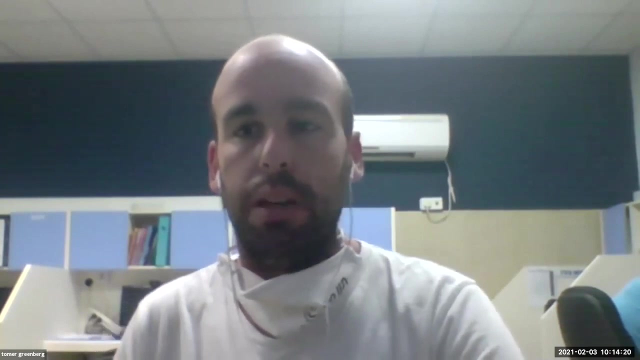 people in the family, but sometimes, uh, um, in small families, they do more damage to the environment from another families. um, so i wanted to say- and that i forgot, i wanted to say that, no, in israel, we, we have a very well, uh, well-being, very well, well-being. 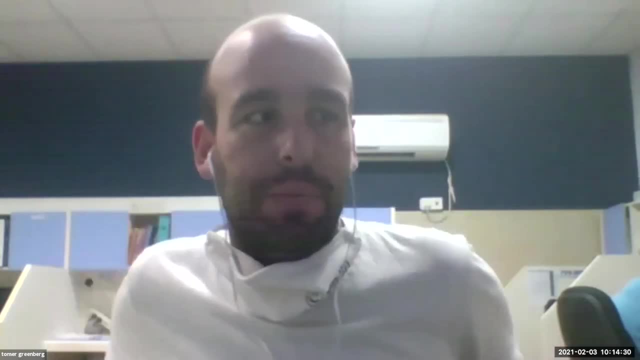 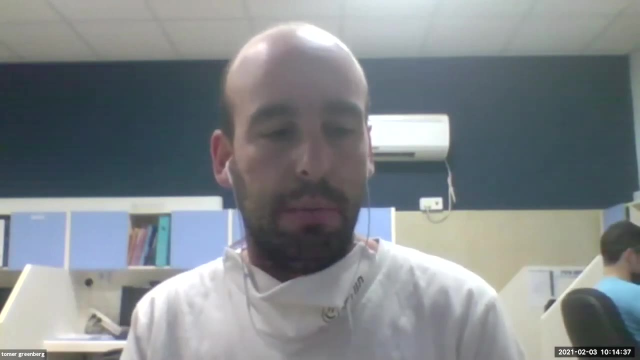 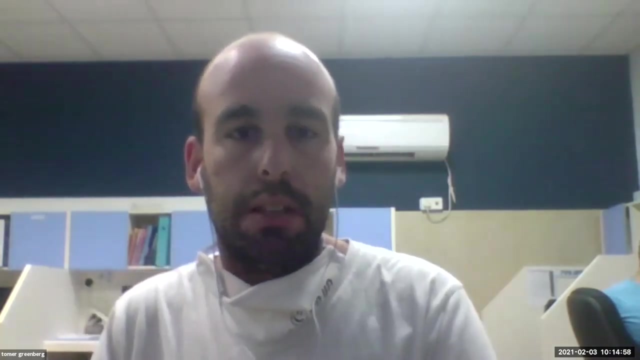 very, i will be um, so. so it make us a confidence or a make us opportunity to, to make changes. this is what i think. because we have a good economic- although there was and the and the and stuff like this- we have, uh, we have the opportunity to have children because, because the life is, uh, is good, we have problems, but the 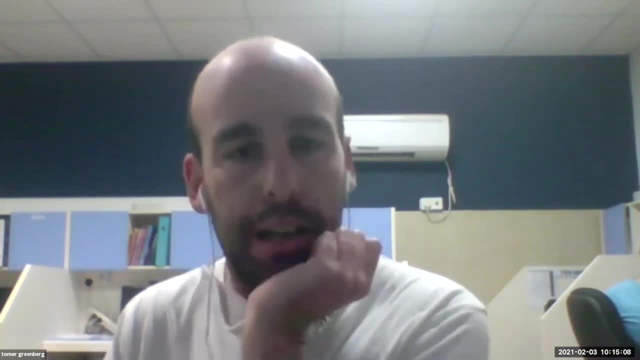 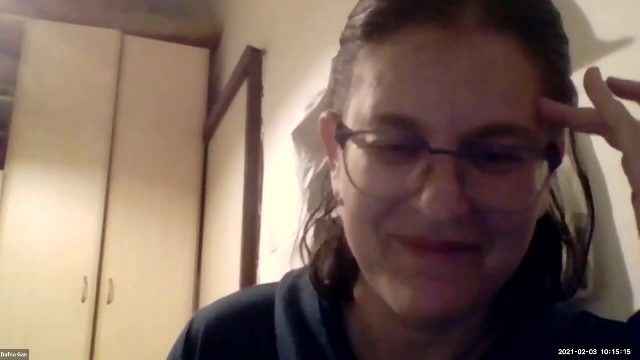 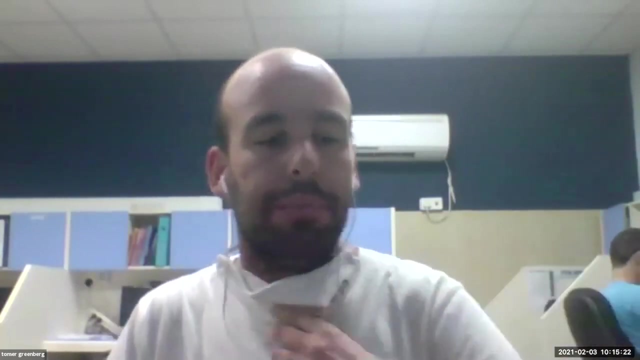 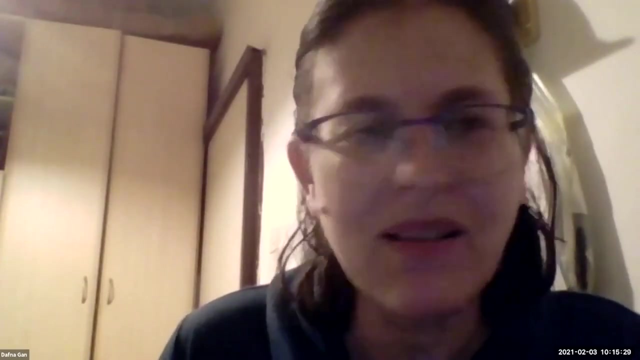 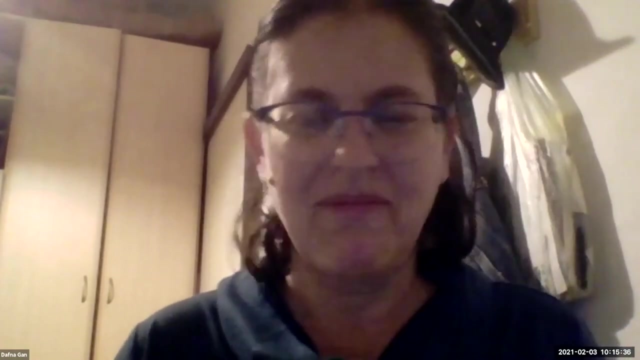 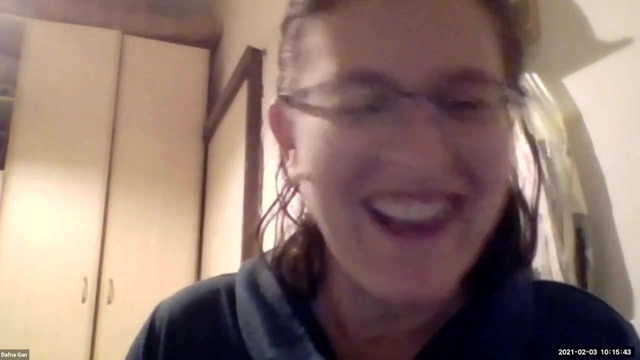 but the life, but but the but. we have the sources. um, no sources, resources, okay, yes, resources, and this is what i think. thank you, thank you, uh. is there any other groups that want to share with us? uh, some thoughts? one, then i will ask, like a teacher, i will ask you. 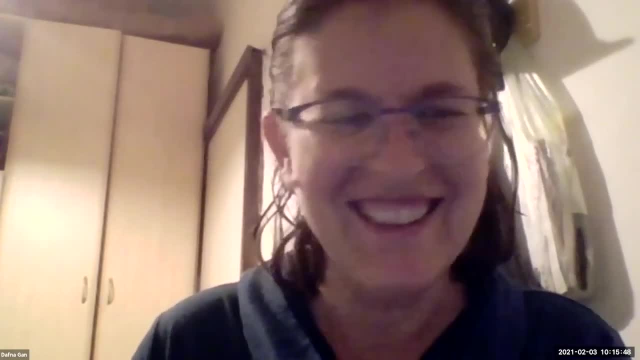 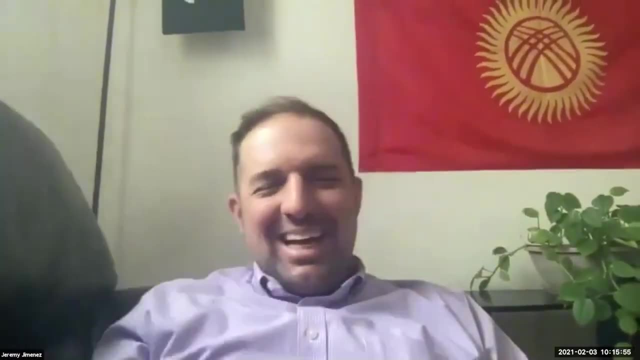 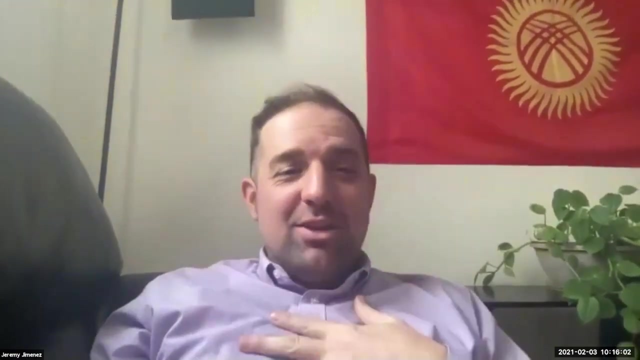 i can say: oh, jeremy, great, thank you. thank you, so we were a bit off topic. uh, i've been, but uh, etty and- um, i'm sorry, it was a gib- uh, uh, gilad and etty they. they really enlightened me about israeli politics. 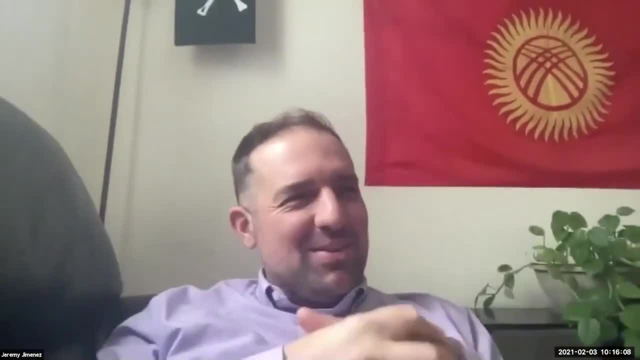 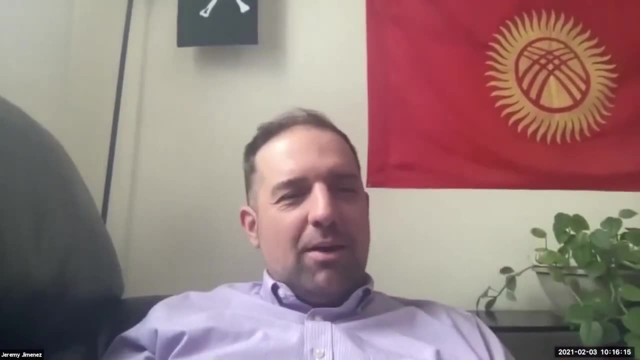 i had a lot of questions about uh the politics going on with netanyahu, and so that was very informative and, um, we did talk a little bit about the why people are resistant to talk about uh population and i pointed out like in the united states there's a historiation of like racist. 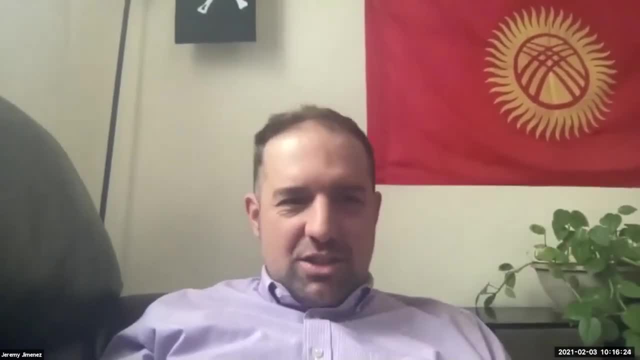 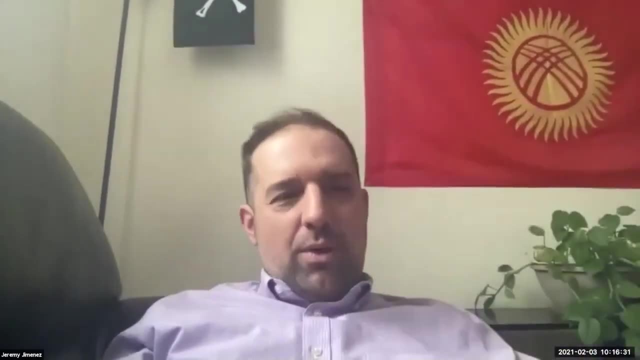 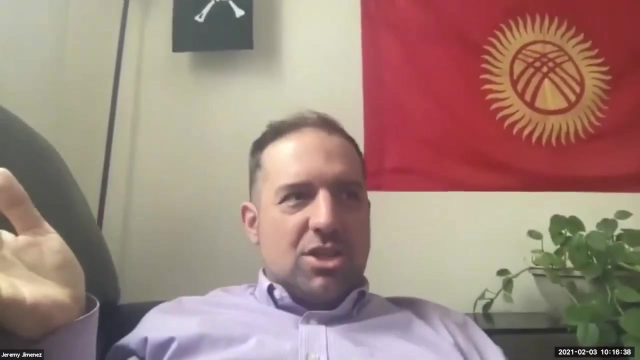 population control right like where, like, a lot of people were sterilized against their will, and so part of the resistance, i think in the united states talking about it, is that racist history associated with with forced, involuntary sterilization in the united states and the idea, if you're talking about population, 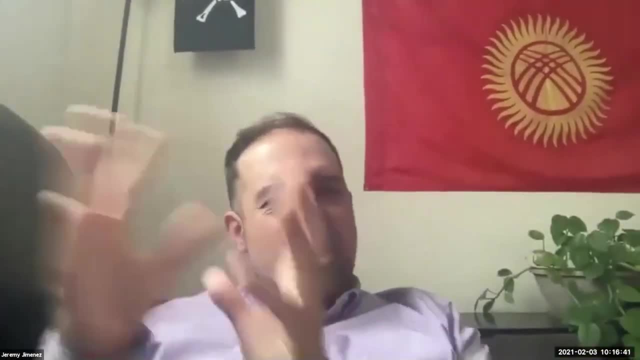 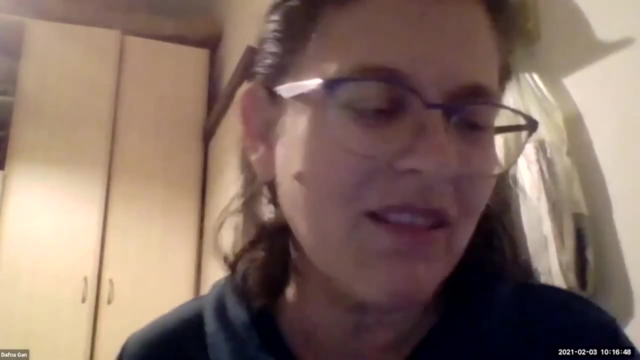 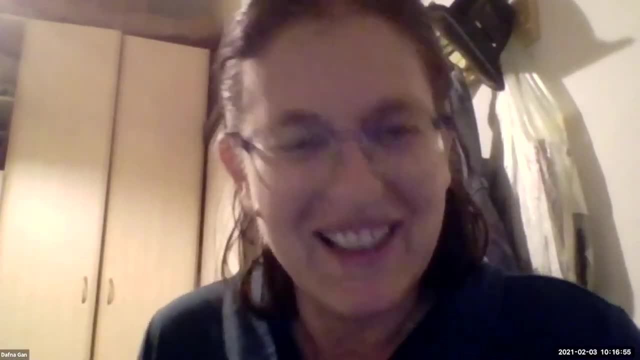 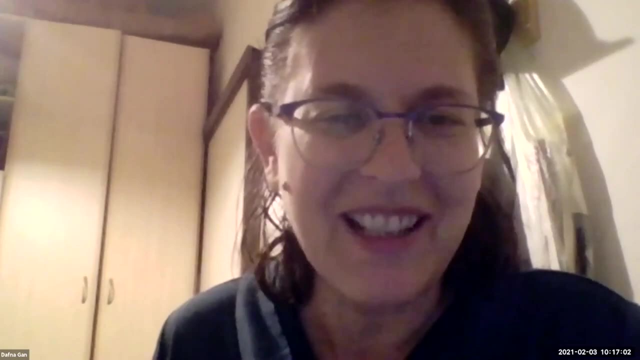 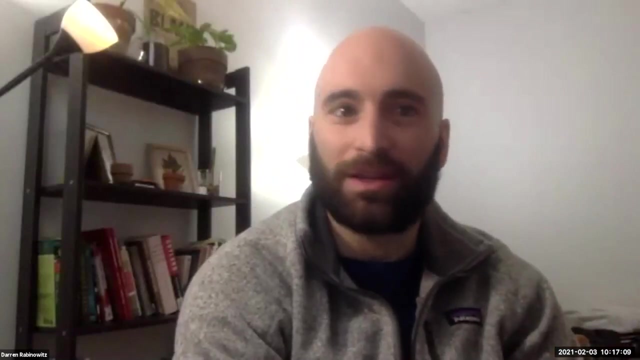 totally part of the of the issue and other group or someone not here yet, darren, yes, yeah. so in in our group we had a pretty interesting conversation um a bit of a comparison between united states and israel, and i think the general gist of the conversation is a lot of the topics regarding 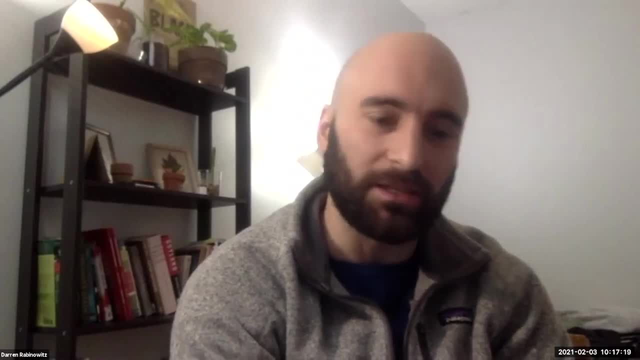 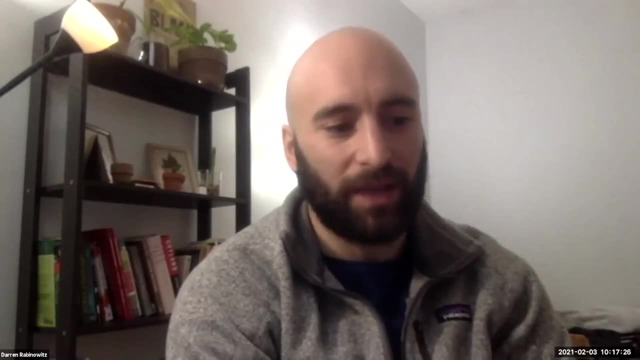 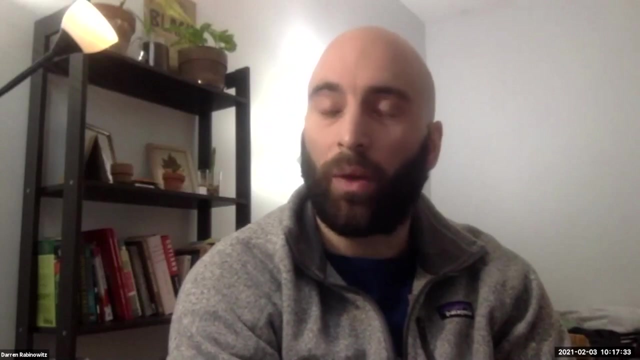 population is very sensitive because it intersects with religious identity, with gender rights and with reproductive rights, and so what we found is that a lot of times, teachers or even curriculum designers are forced to globalize conversations so that there can be a way to talk about in a 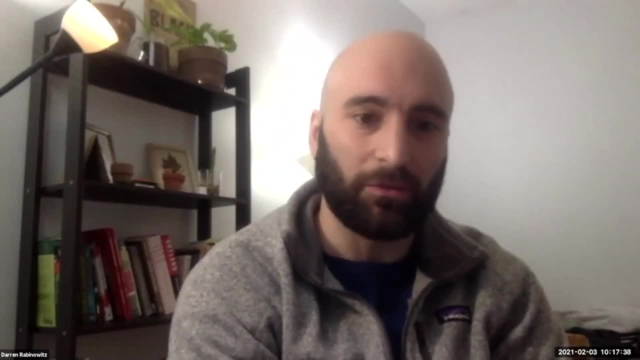 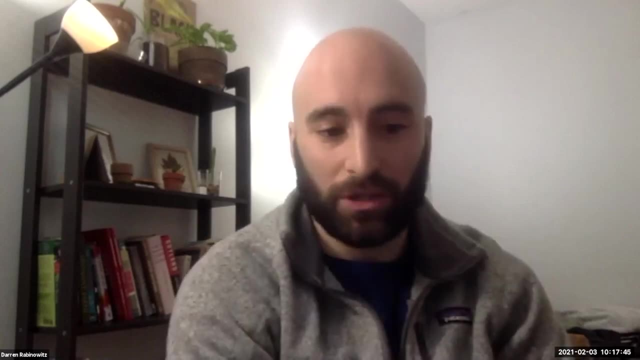 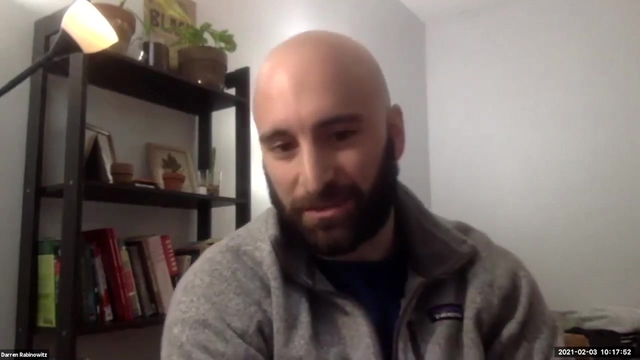 more generalized sense and rather than a context, specific sense. so we talked about utah and perhaps the sensitivity of talking about with religion and population growth is very sensitive. so having some successes when talking about human rights instead of context specific uh drivers, um, is perhaps an intersection. also, environmental ethics, um, rather than talking 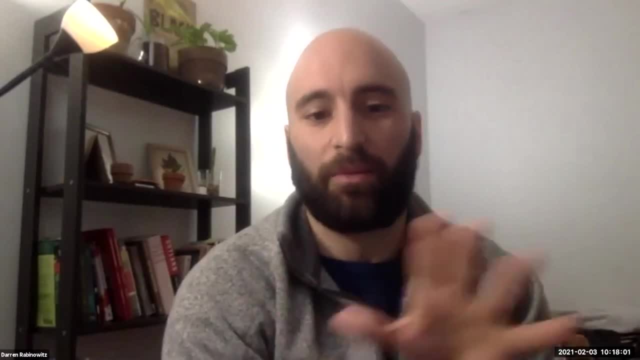 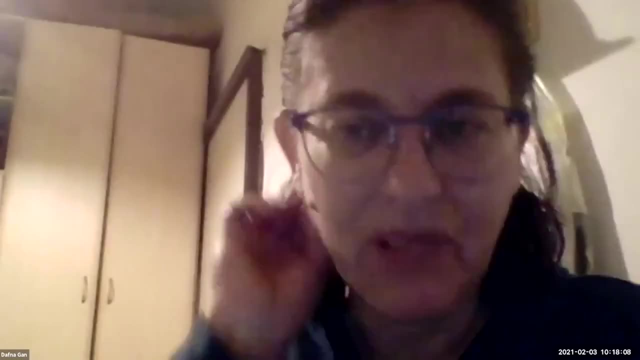 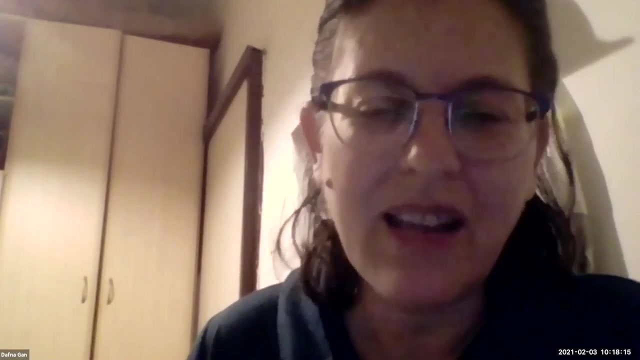 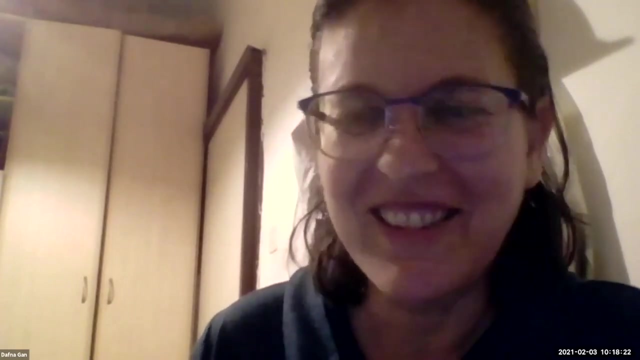 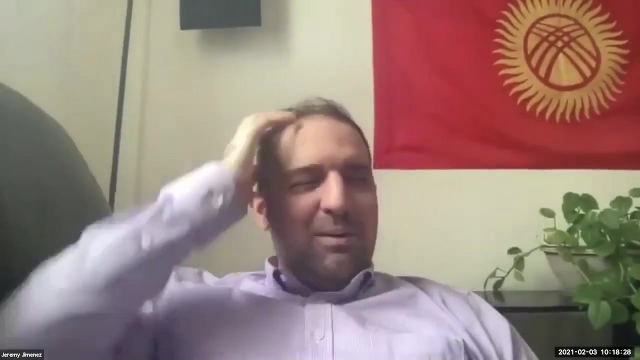 about population growth, so it is fascinating to think about the other directions into this conversation that might not be so context specific driven. thank you great. thank you. more comments. you can say something even if it's not related to your group conversation or discussion. okay, i guess i could say one more thing. um, yeah, we also talked about how we noticed in some of our 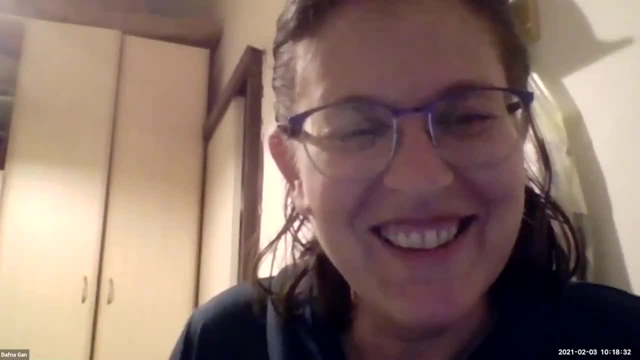 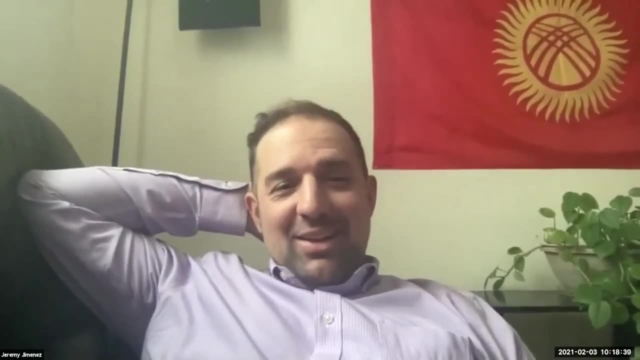 conversations and research that young children seem to be more comfortable talking about it than a lot of adults are. as an issue and um, i'm going to share it all with you, something i've never shared before as an anecdote. i i didn't publish about this, but when i was interviewing students 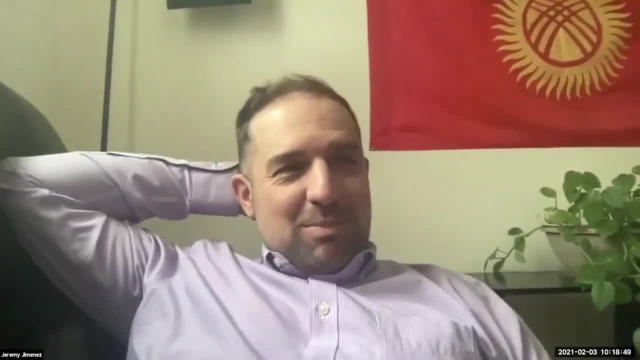 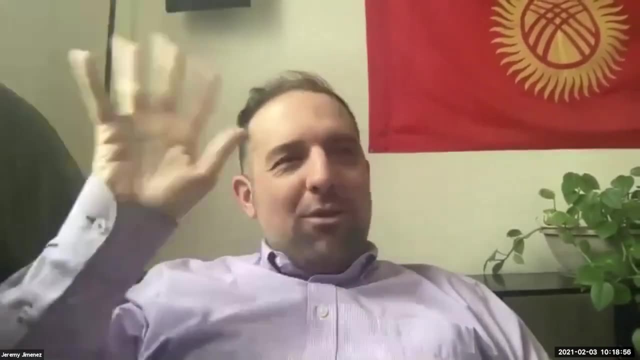 about like environmental issues. i was like, okay, i'm going to talk about this, i'm going to talk about environmental issues and you know, things like population and sustainability came up one fourth grader. i'll never forget what he said. i was talking about like solutions and what can be done, and he 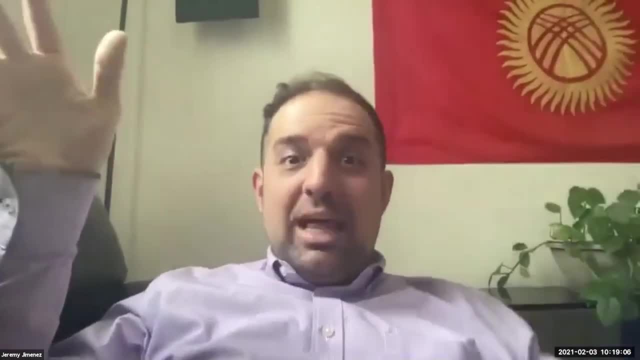 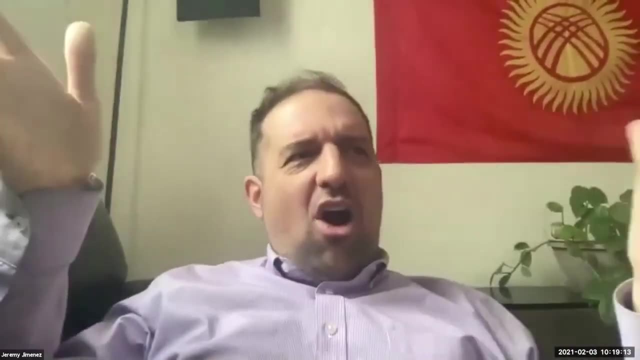 says we should put electric batteries on planes, right, and i'm like, and i was like, oh you, but this is a fourth grader, like you might remember- that i said like it's very hard to put an electric battery on a plane because it's, you know, the energy density to propel a plane with the battery. you need. so many batteries it's not really feasible. 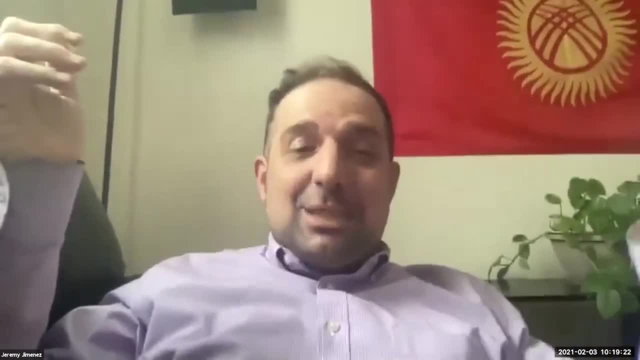 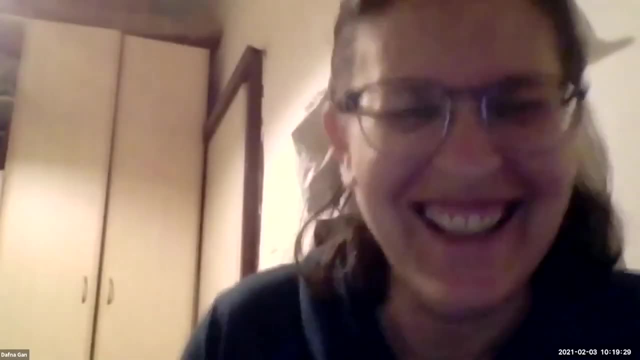 you need so many batteries. it's not really feasible. you need so many batteries. it's not really feasible, like he's. like, exactly that's the point. we'll solve two problems: we'll stop the plane from flying and we'll get rid of the people on the plane as well. so, like that's like the level of 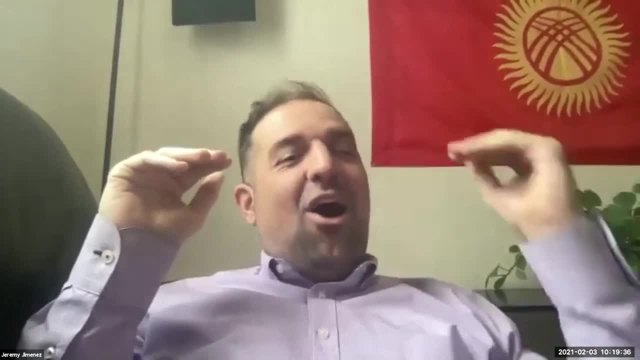 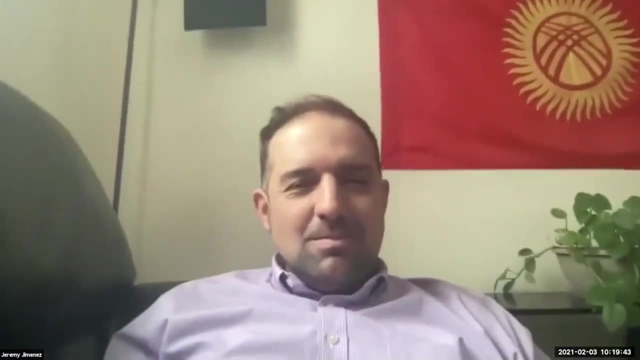 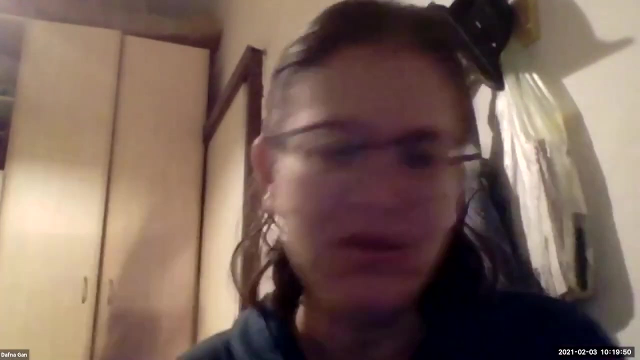 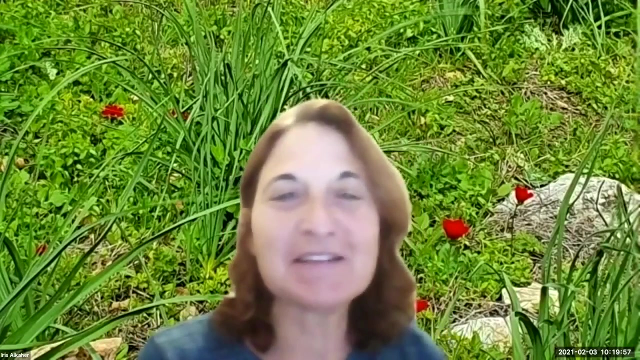 like dark brilliance with which i think some students are thinking and talking about population in ways we adults might be averse to. thank you, thank you, yeah, iris. do you want to to say something? oh well, it was a good opportunity to- uh, you know, to present it in front of a. 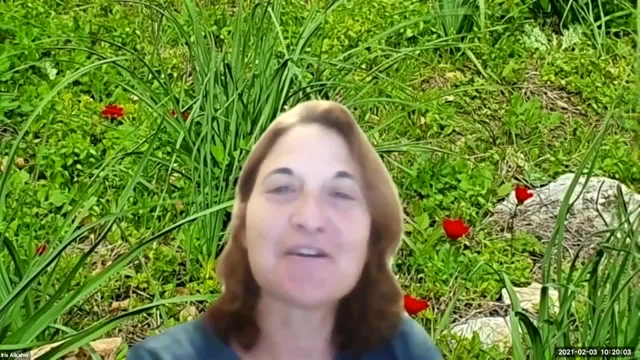 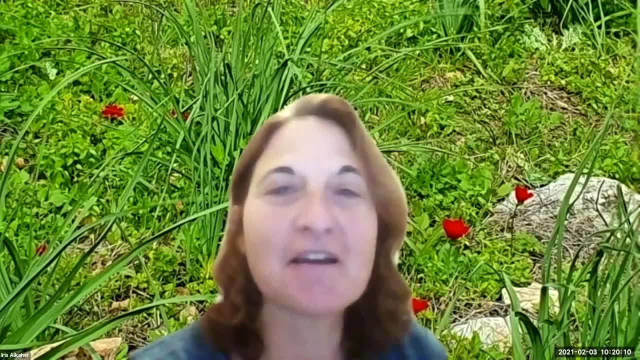 israelis as as well as the other, uh, other countries and for me- and i would like you know to call for uh, you know if there are other students or researchers here who are interested in in continue this research and make it, make it international, because i know. 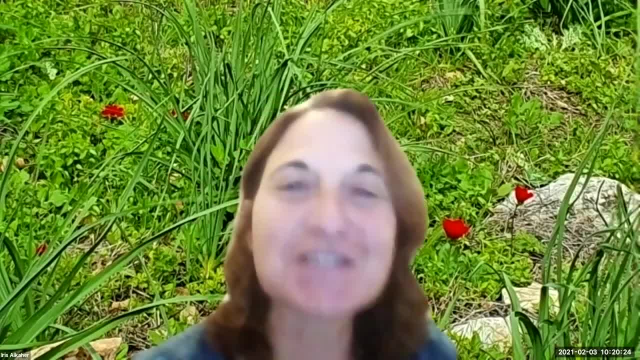 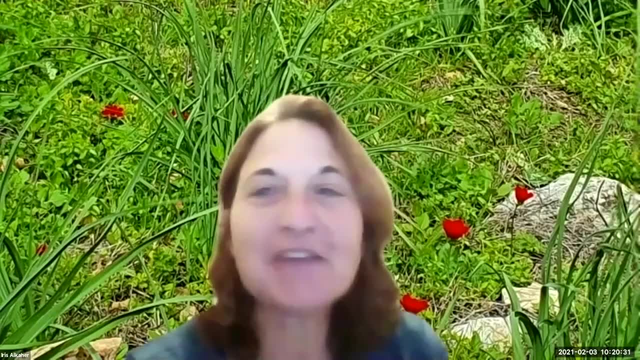 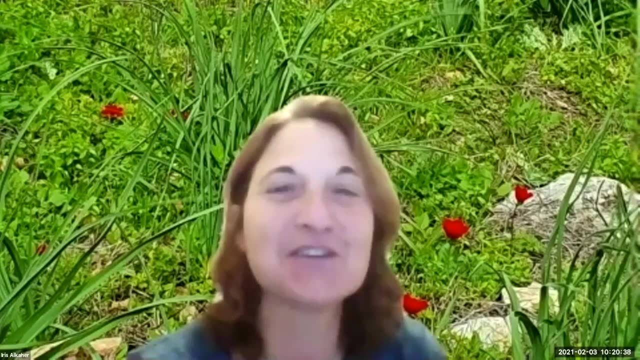 that, uh, you know the findings would not are not necessarily uh, will be the same. so, in right to me, suggest yourself you know for, uh, you know for conducting, you know maybe to administer um questionnaires or join, join the research. i would be very happy and and it was interesting to hear, 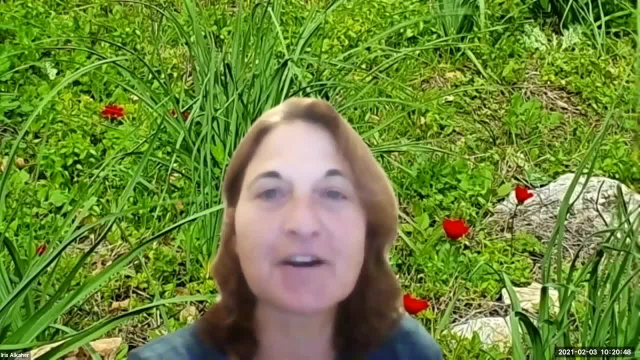 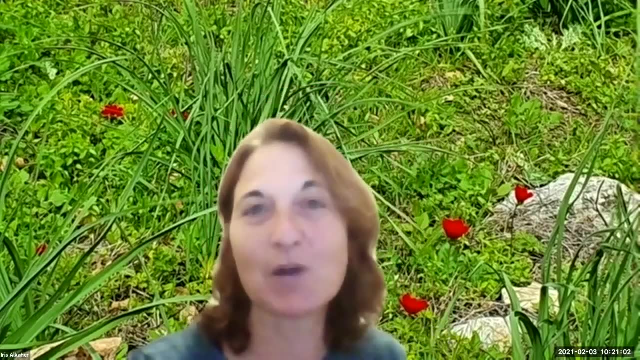 you in the small discussion and also here, and you know, i heard the same explanations and and you know and reasons that the people he raised- as, as we found, you know, in the interviews and in the questionnaires about the topic, the same issues were- were raised here. 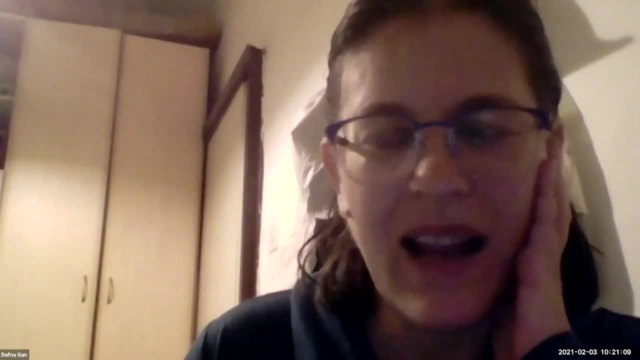 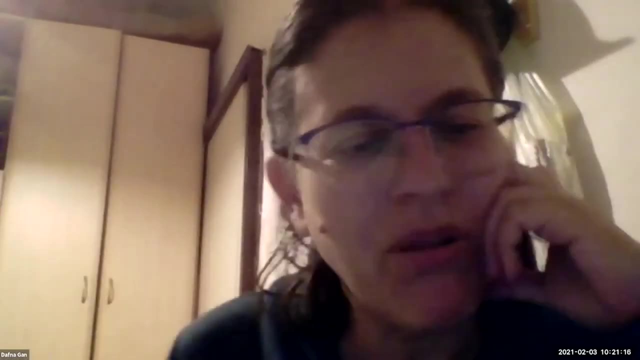 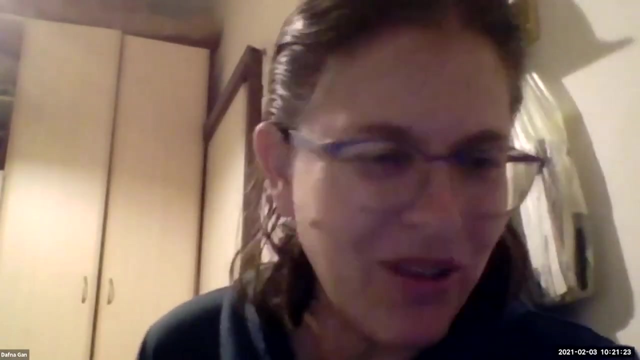 thank you, thank you and uh and i, i think if we, if we are looking, and so we're trying to look at this workshop in diverse ways and diverse approaches to the questionnaires. um, we're, as you know, serious about the questionnaires because the description is carte blanche: on the one hand uhly and but uhsten, who were. 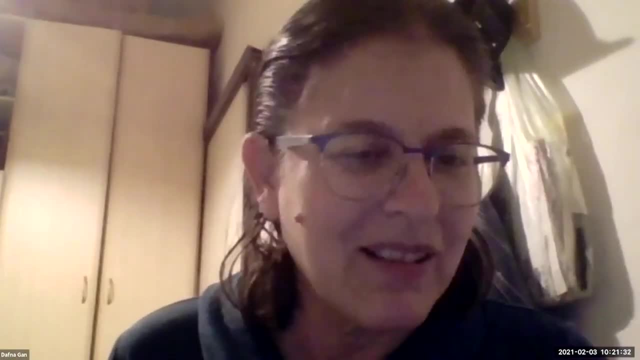 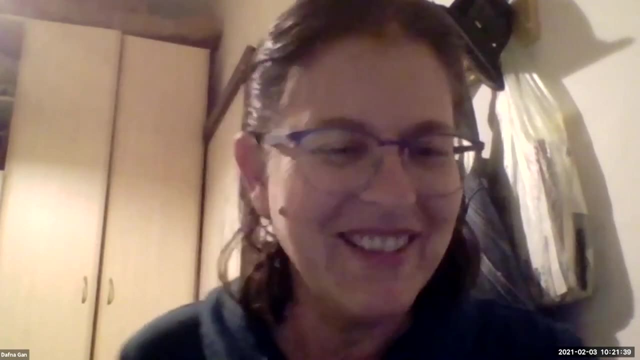 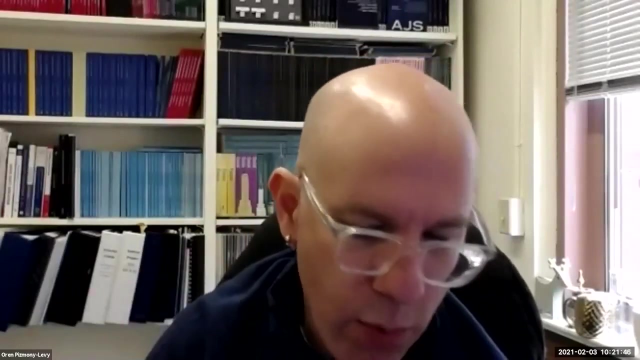 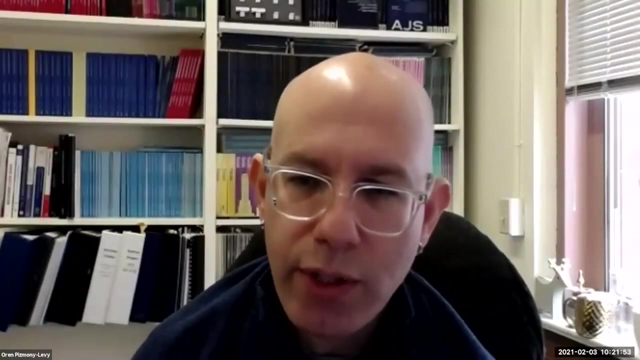 growing above популярity among the scientists's uh, some of the questions among the scientists to ask the questionnaires, the questionnaires, and on the other hand, i want to be nepal into an uh of the group. It seems like we are always dealing with topics in our field of sustainability and 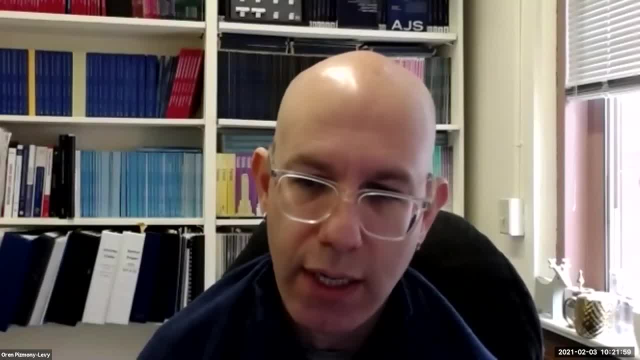 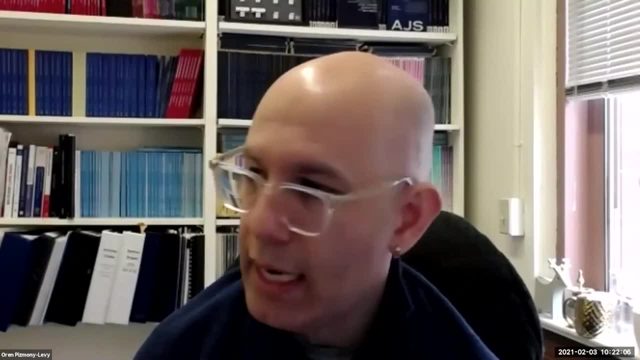 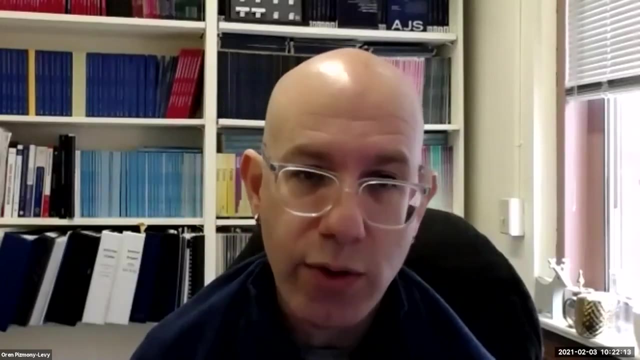 environmentalism. We always deal with topics that are controversial. I'm thinking about climate change, I'm thinking about evolution, I'm thinking about, in some context, I'm thinking about an environmental educator in Texas trying to talk against the fossil fuel industry. 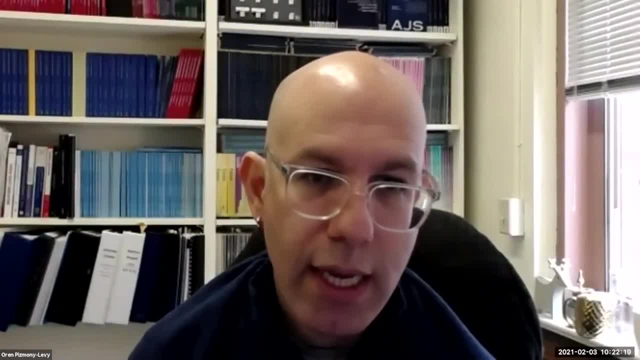 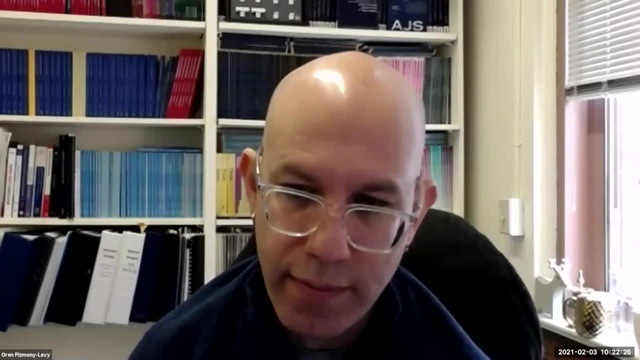 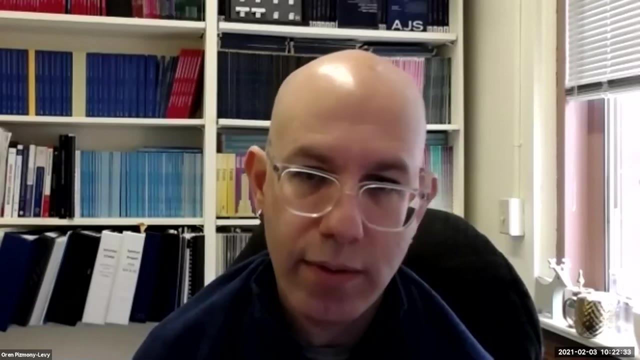 That will be very controversial. I wonder whether there is something unique about population growth as a topic, or is it really another case of these hot topics that are just difficult to talk about? I wonder whether Iris has thought about it, but if others, 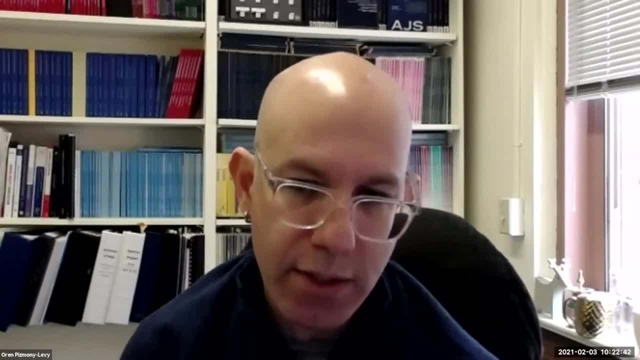 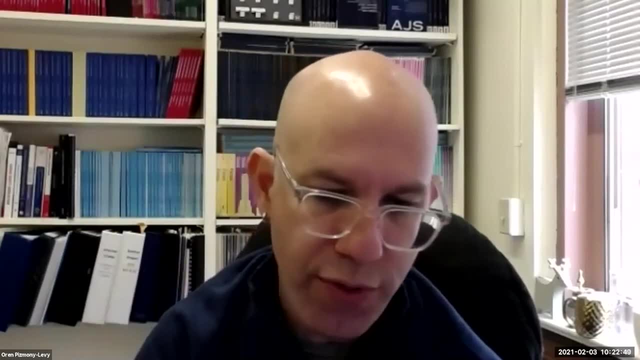 Because if it is unique, then maybe we should talk a little bit about the uniqueness. If it's not, then we might want to think about a broader system or framework of thinking about these hot topics that goes beyond just the population growth and climate change. 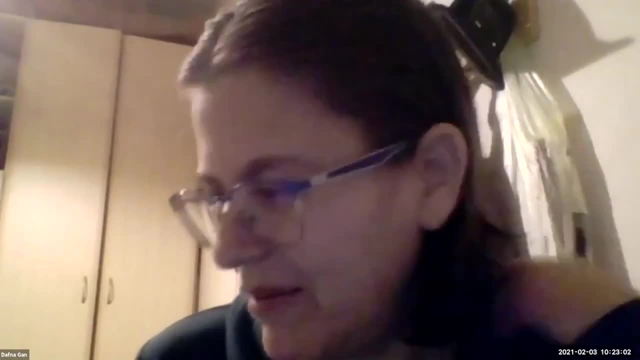 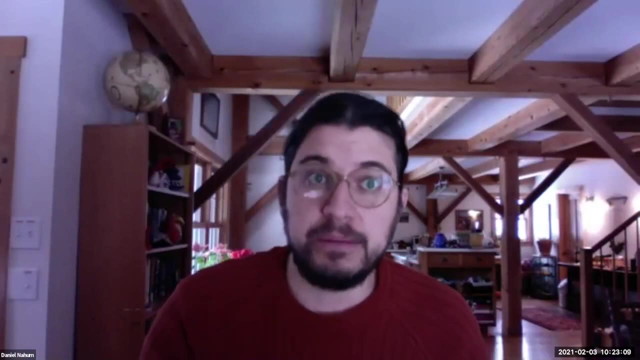 I see, Daniel, Daniel, yes, you can go ahead. Yeah, I just wanted to touch on that. I find it to be just like climate change. I find it to be a topic that needs to be unpacked and unpacked a lot. 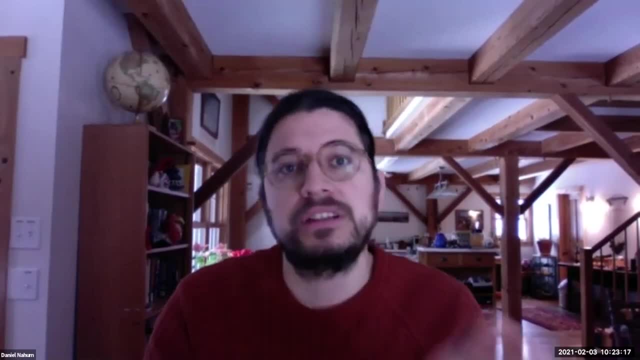 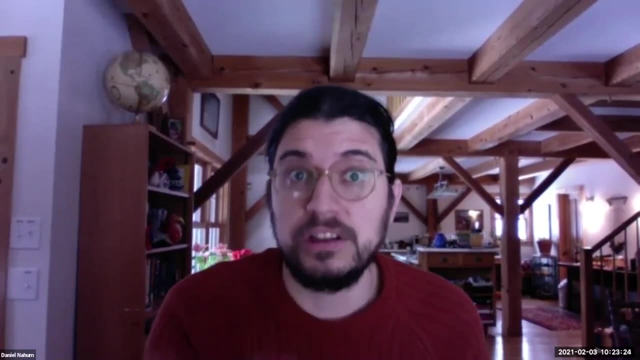 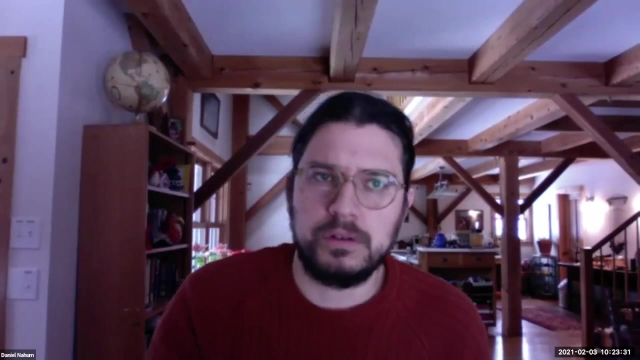 like really dissect, and dissect in different contexts. You can tell that here the conversation was focused on Israel and the US, because this is our context, This is our lingo, but I think that to help talk about these difficult topics is, I think, to dissect them and try to make them. 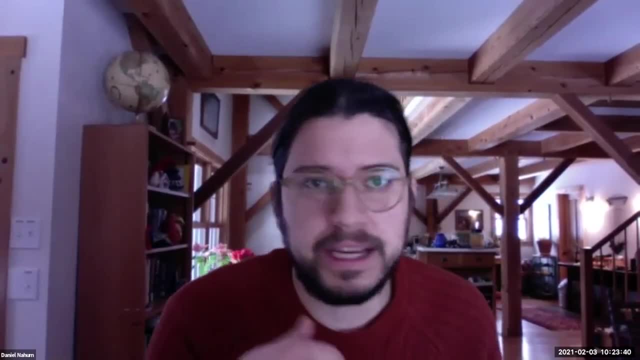 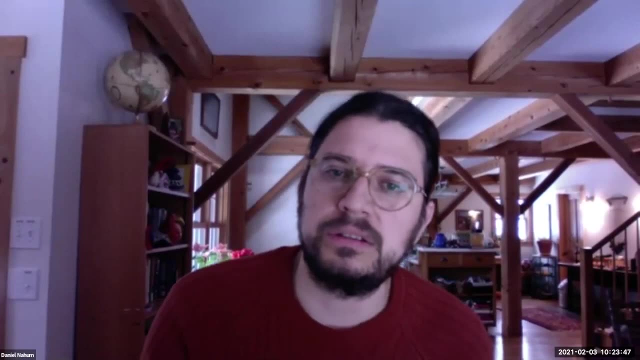 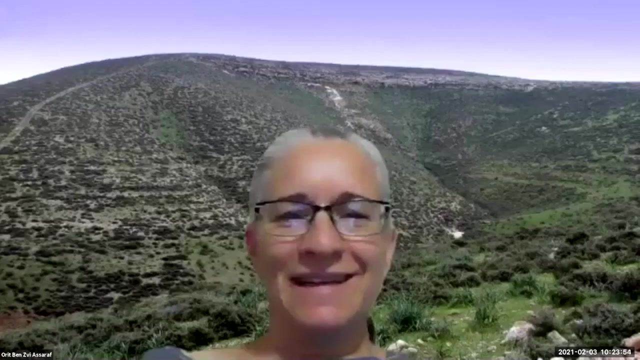 trying to build bridges right with ways in which a Texas teacher can talk about it, aligning with his identity and his context. I see Orit and then Susan. Okay, Orit and then Susan. Thank you all for your comments. I think that, for me personally, I would like to embrace the 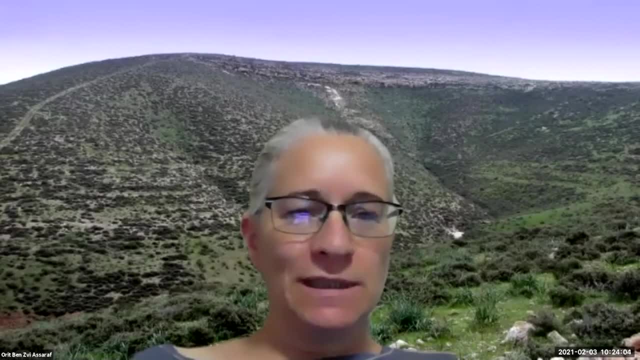 cultural, responsive pedagogy when dealing with such an issue. It's very familiar for me as biologist, like evolution. Personally, you know what is the right mechanism. Nevertheless, you know how difficult it is to teach such issue in the overall population in order to achieve 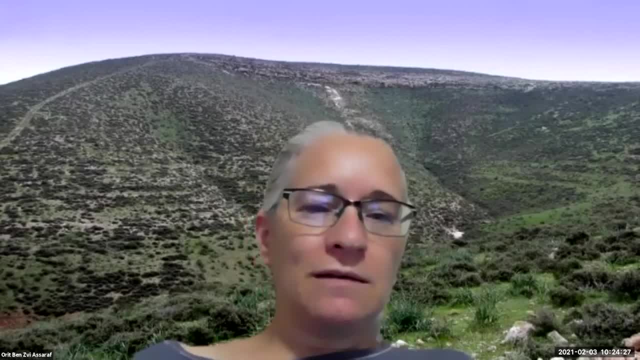 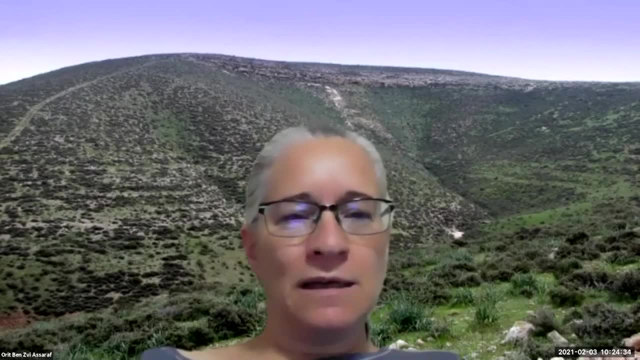 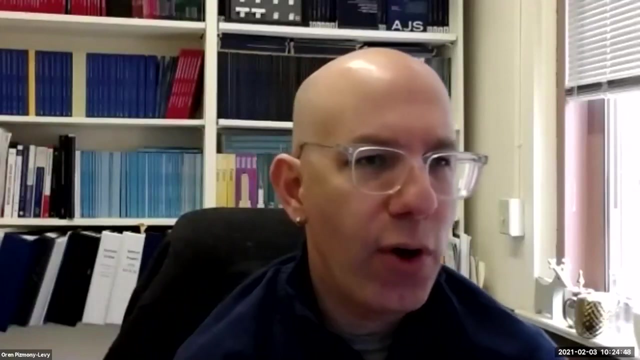 what we call informed decisions. So I think cultural responsive pedagogy is in a framework that really helps you to be more modest in how you relate to population growth or revolution, But for me they are in the same level. Can I ask a follow up, Orit, because I don't think we ever talked in this group about 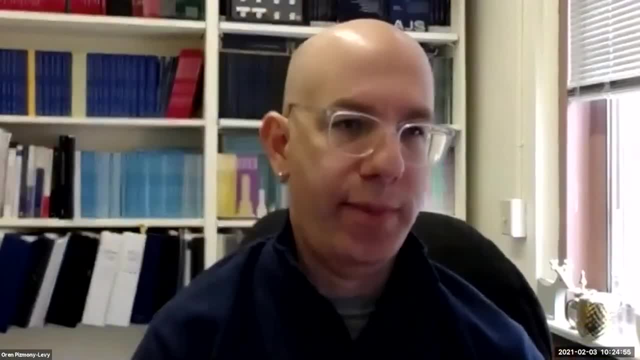 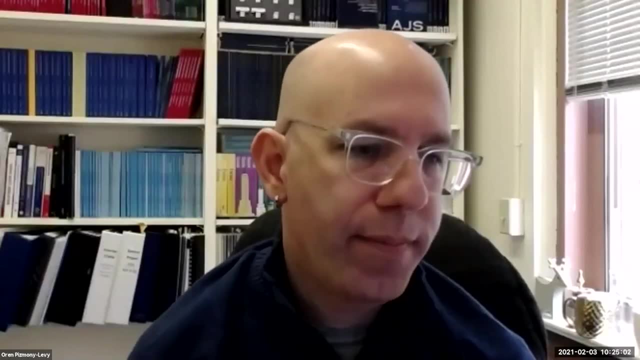 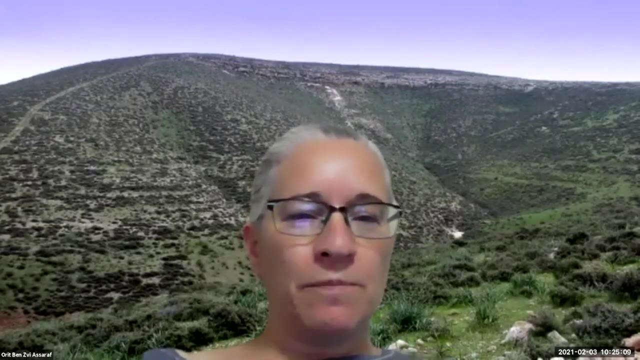 cultural relevant or cultural sensitive pedagogy. Can you say a little bit more about how you see the connection? I think it will be useful for everybody. Yeah, when we speak about cultural responsive pedagogy, we ask ourselves: what is the cognitive model a person holds, What are the norms that influence those and how can we improve? 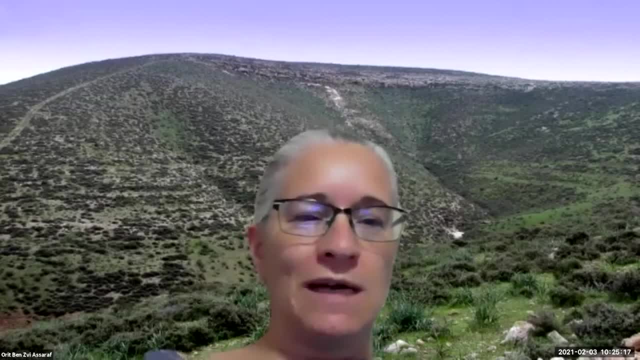 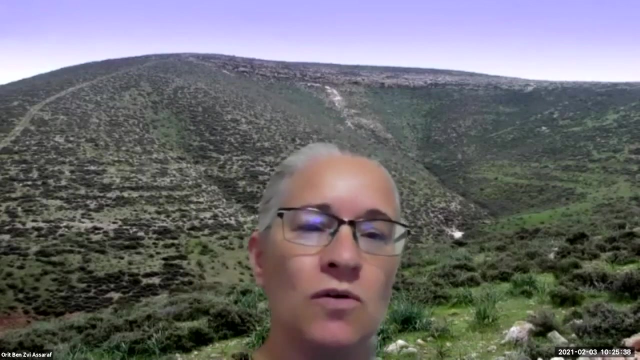 um cognitive models. what kind of cultural attributes are related to? how is um self identities related to the issue? uh, there are in discourse and there are. there are many papers more recently, like the last five years, on cultural responsive: all kind of discourse and dialogue, teaching and meaningful learning experiences that promote and scaffold a understanding. 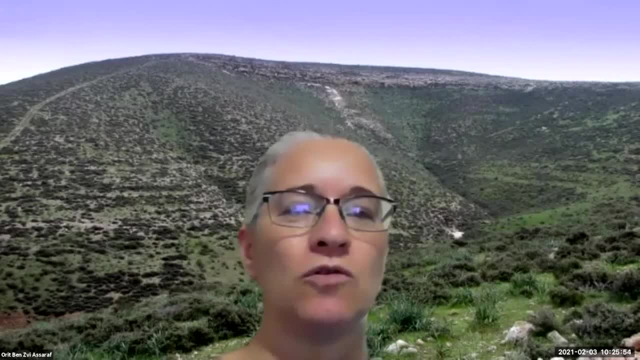 but it must be very open. it's not like you can convince someone to doing a replacement. it's more refinement and in this process of refinement you you can negotiate the meaning of what is mean population growth. but it's not really um a replacement, and this is something that many environmental educators. 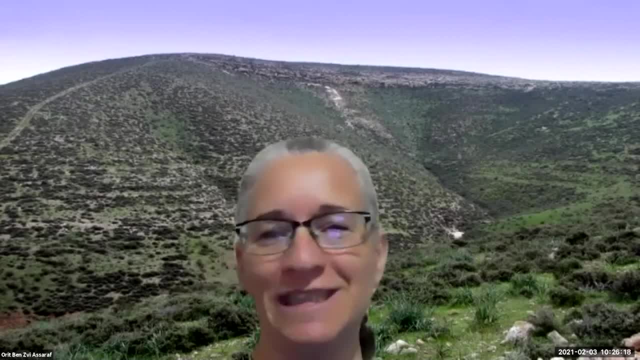 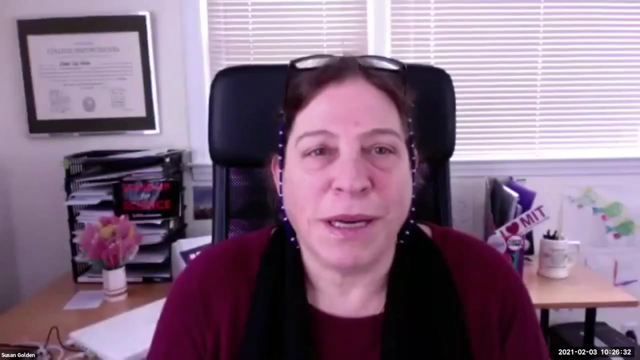 have problem with. they really want to convince and and it will not work in my. this is my opinion, of course. thanks, thank you say, susan, you wanted to to say something. yeah, i think orit said it much better than i can, but i was just answering oren's question of: is the population topic um? 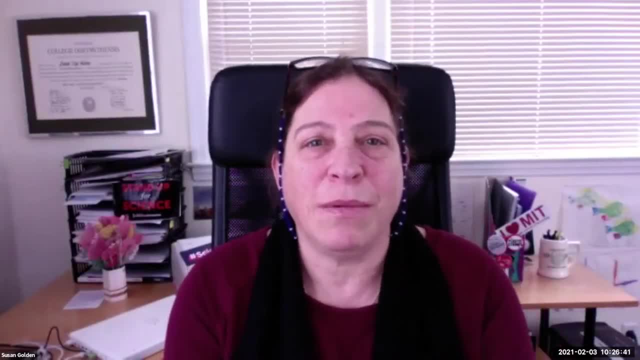 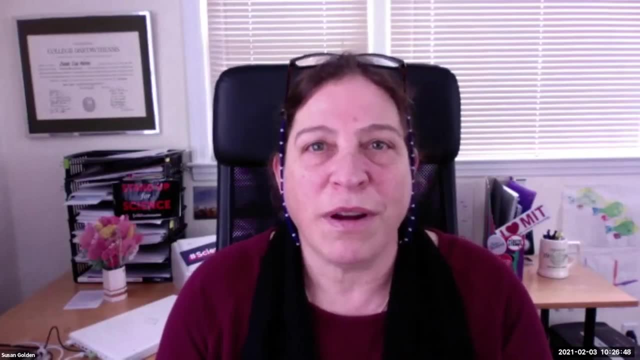 different than the other hot topics and i think that said it well. i think in a way, it is it yes and a no. um, if you want to talk about it from the environmental perspective, then i think it's just another hot topic. but what population growth does? 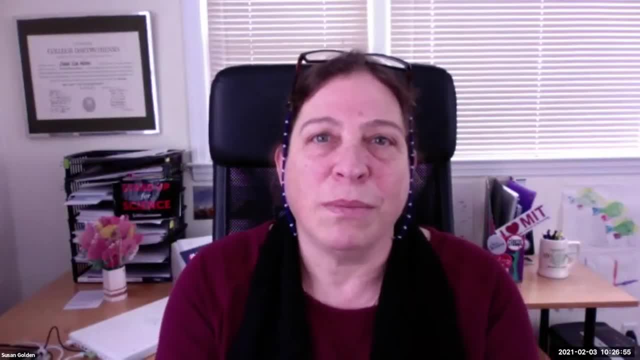 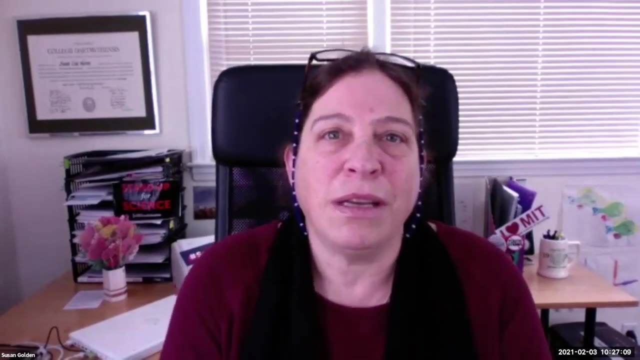 is that, as we mentioned earlier before the breakout rooms, it brings up the issue of fertility choice and personal freedoms and women's rights, and when you get into that discussion you bring up the cultural norms and other expectations and things like that. so that to me, does that aspect of the 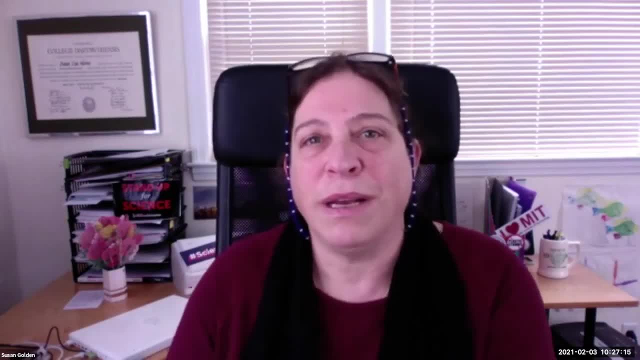 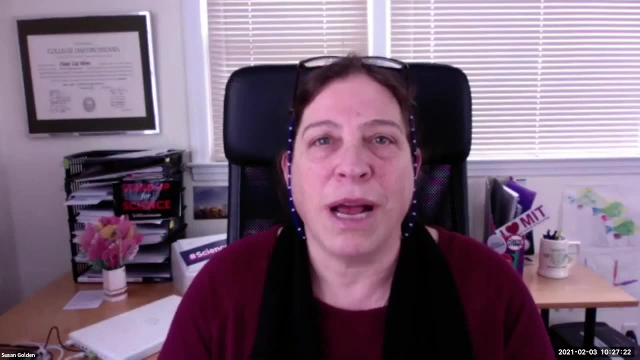 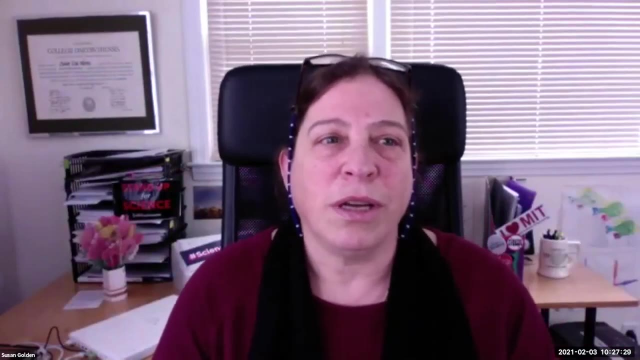 issue makes it a unique problem. however, i think it could be dealt with as just another hot topic as well, if we stick with the environmental implications and don't address personal choice. so let's talk about it as a global or community issue and not a personal issue. 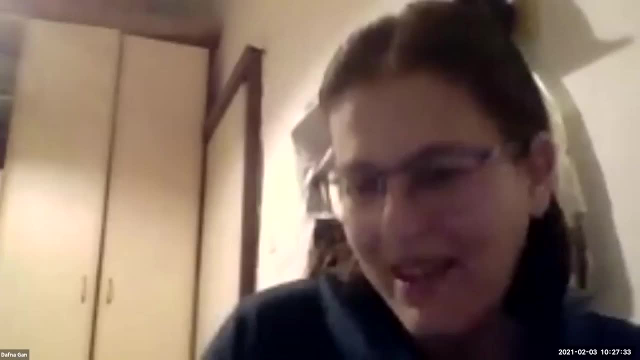 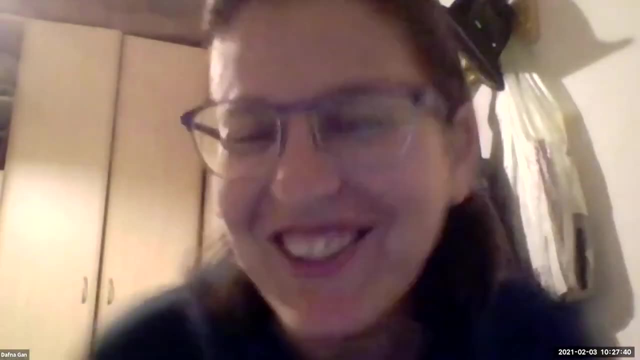 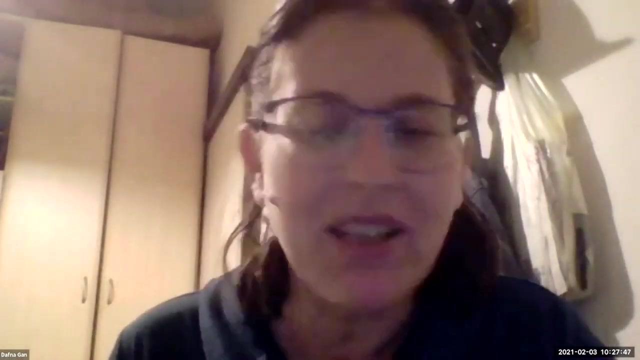 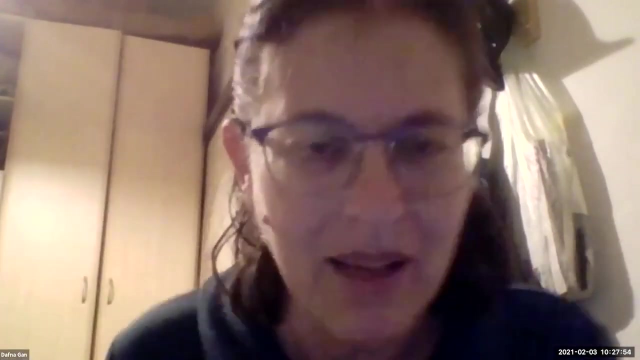 thank you, great thank you. so we have um um, three more minutes, uh, uh. so now i can wrap up what i wanted to do 10 minutes ago, but i wanted to say that they, we are looking, and actually it relates to your question. oh, and we're trying to look at this workshop from really diverse angle, about sustainability and about 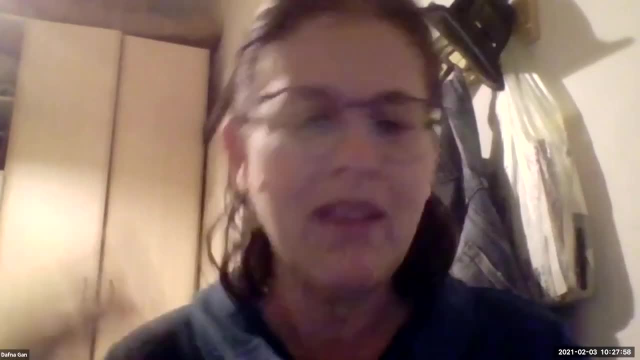 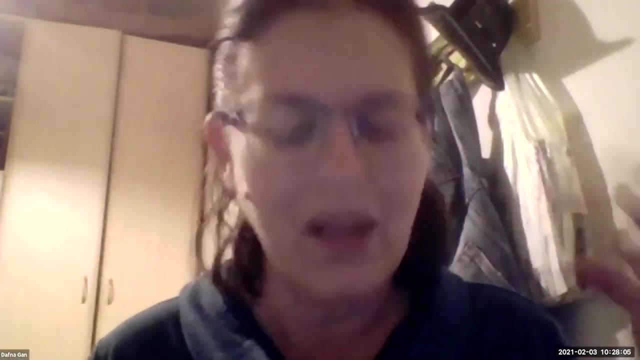 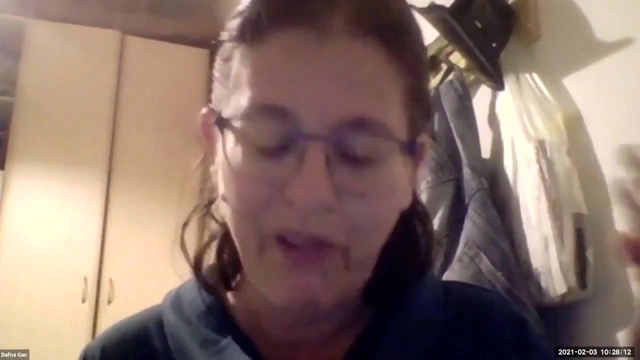 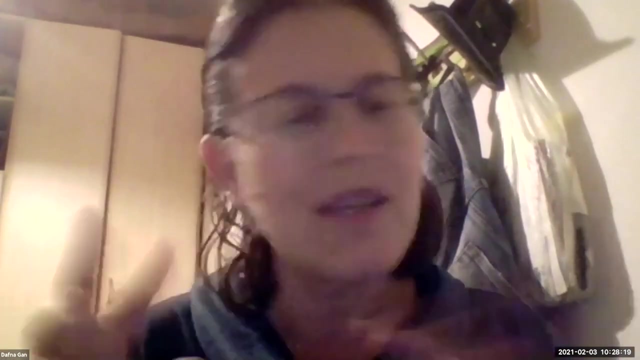 research about it, a quantitative uh tools and qualitative, and from the perspective of uh a population growth, or from the perspective of climate change, or for or from the perspective of uh our imaginary world. i think every everything is connected. i don't think it's separate uh war. i think